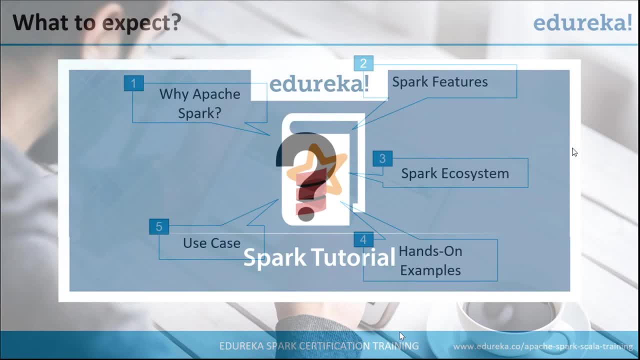 So this will be the agenda for today's session. So in today's session we will understand why Apache Spark, what are the Sparks feature, what is Spark ecosystem. then we will be looking at the use case of Spark- Spark is being used- And then also I'll introduce you to the Edureka's lab and we'll see how do we perform the handsaw. Okay, So one thing I would. I would. I would like to clear the expectation here very clearly that, given the time duration, it's not practically possible to cover each and everything in detail with respect to all the ecosystem components of Spark. But it's like I'll make sure that the complete picture is clear or you will be able to see the entire picture. 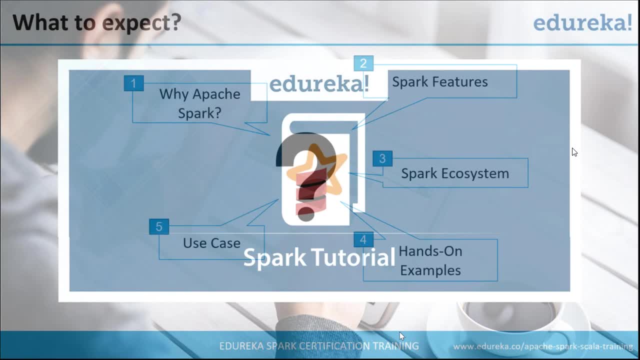 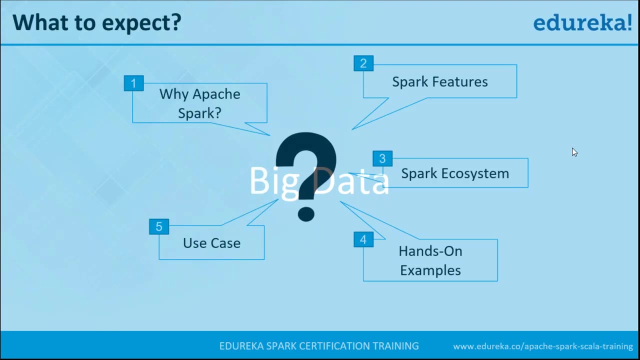 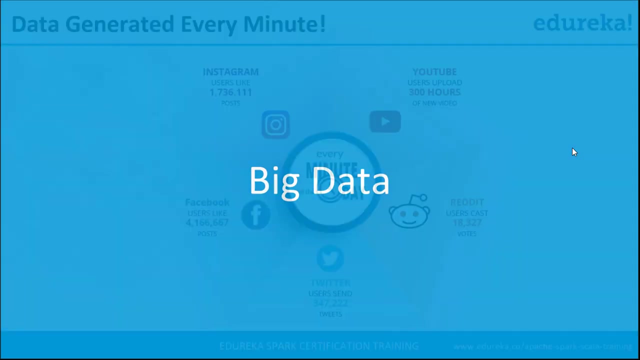 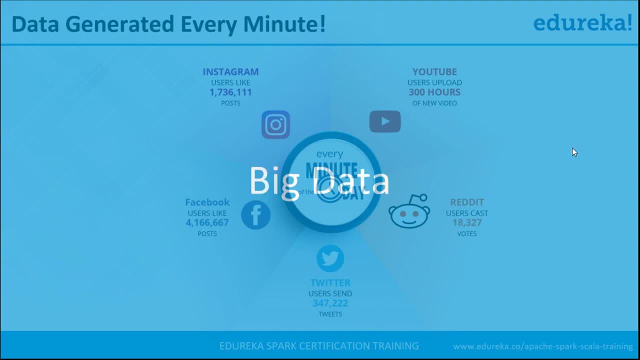 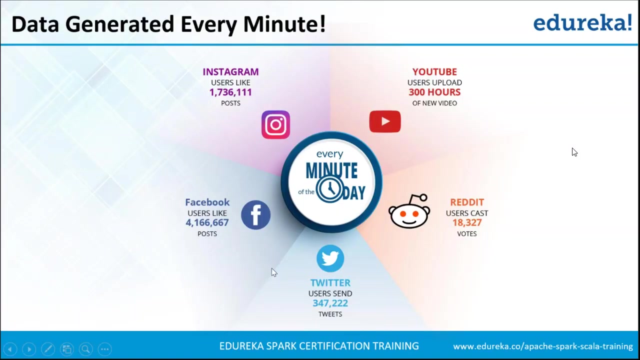 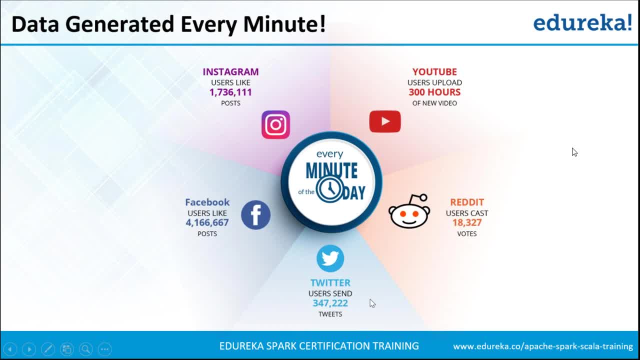 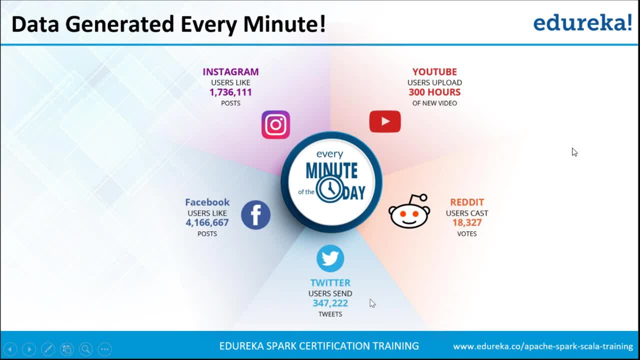 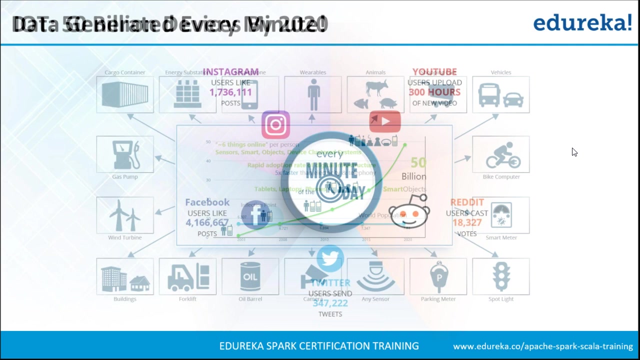 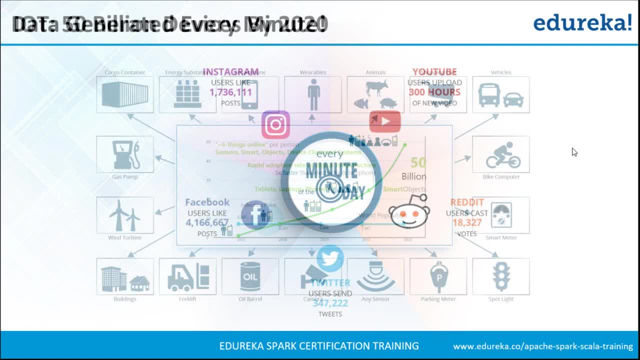 or what are the facts, factors responsible behind this growth of data. so we will be talking about social media platforms, right. and then we will be talking about smart devices as well, right? so nowadays we talk about iot. it's like we are using n number of smart devices, and what those devices? 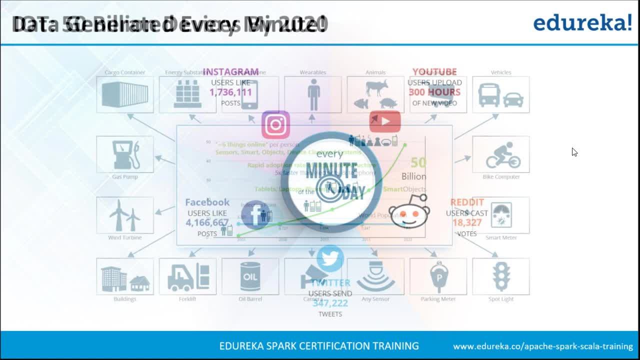 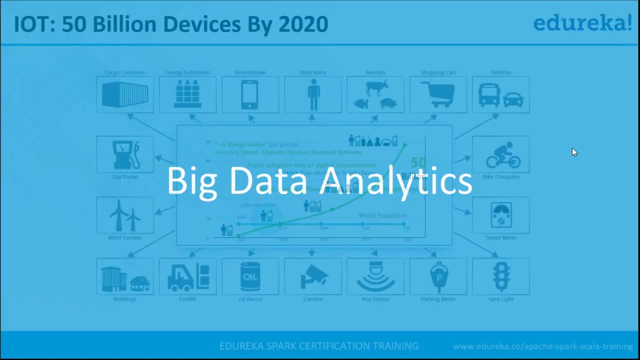 are doing. those devices are, uh, generating huge amount of data every second, right, every millisecond data is coming from these smart devices, right? so, yeah, and also, we talk about evolution of technology as well, right, like smart devices, as in, technology is evolving and hence more data is getting. 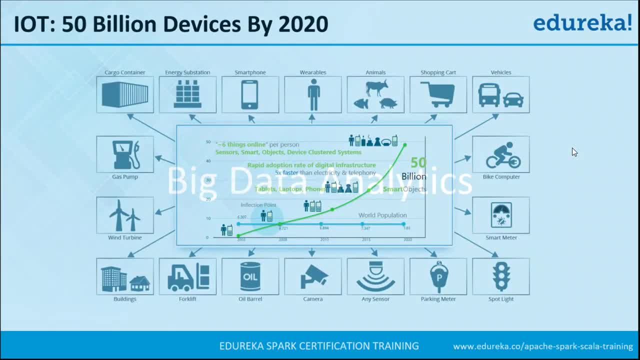 generated. right now we will talk about big data analytics. so the point is: we have understood what does big data and how is it getting generated. so if i talk about the formal definition of big data, it says that it's the huge amount of data. it's a huge amount of data which is 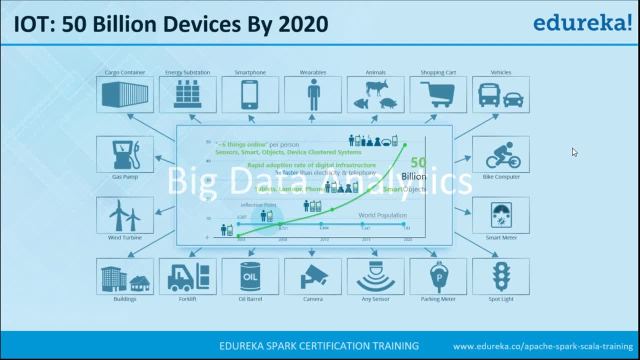 getting. it's a huge amount of data which is getting generated at a very high speed and also which has got varieties of data, varieties of data as in- if i talk about facebook, right, you know that on facebook we have text data. we do have audio data, video data, all kind of data and that data. 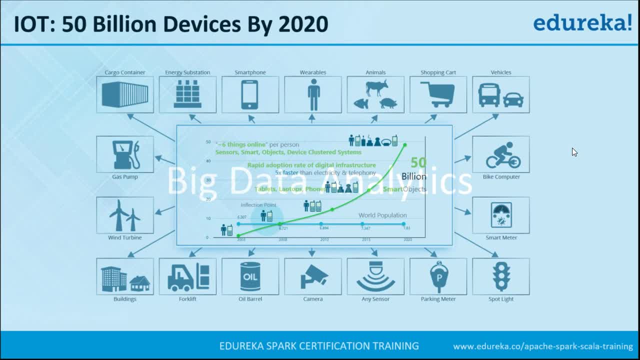 is getting generated at a very high speed. so, at the end of the day, facebook has to deal with huge amount of data which is flowing continuously and also which has got varieties of data. so now big data analytics. so the question comes: what is the need to store and to process this huge amount of? 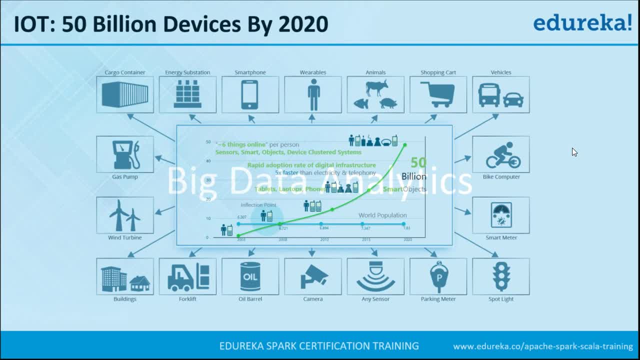 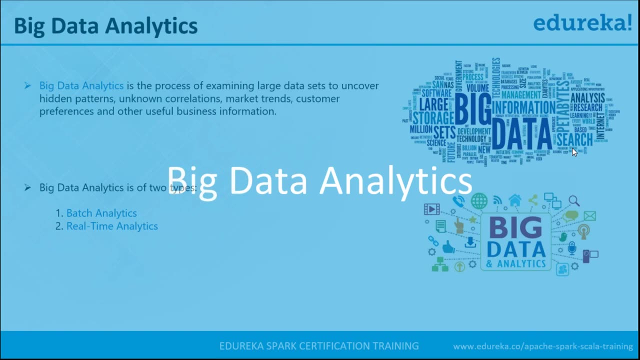 data. question is: what is the need to store and to process this huge amount of data? right, so the process using which we we process this big data- we call that as big data analytics. so let's look at the technical definition of big data analytics. it says it's a process of examining large data. 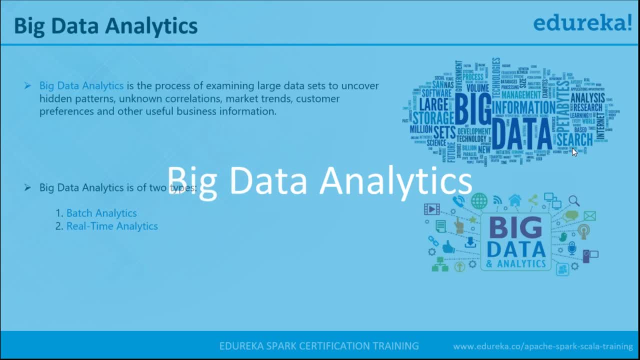 sets to uncover hidden patterns, unknown correlations, market trends. so the point is: why do you think that organizations are interested in uh, storing or and processing this huge amount of data? objective for each and every organization is to make more profit. so, end of the day, the organizations are saying that whatever data we have got right, let's try to find out the. 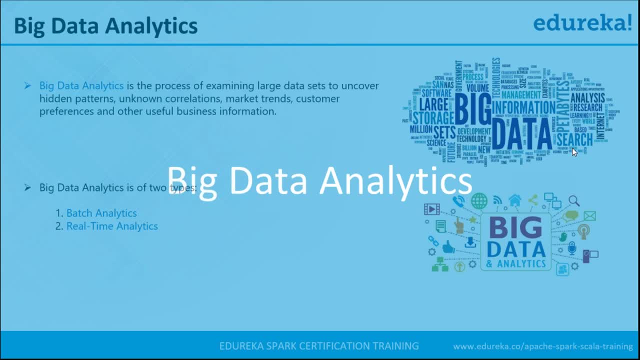 meaning out of it so that we know how how, how customers are behaving, what is the sales trend? you know how can we increase the sales? so one very, uh simple example: let's say that i do have hundreds of students in my class and out of those hundred students i do have tens of rahuls, and i am 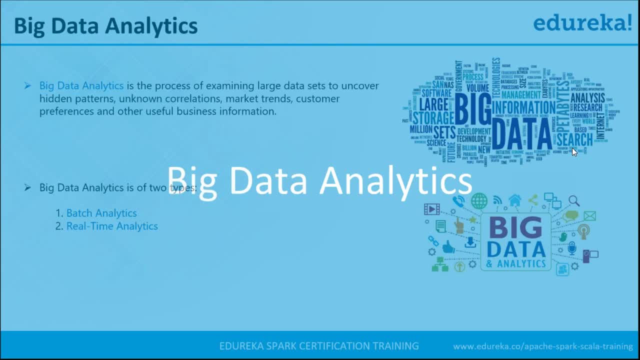 interested in talking to a participant named rahul sharma. what am i doing? i'm just calling out the name rahul. so do you think that if i just name rahul and i just call out his name- so i'm just I just call out the first name- I will be able to talk to the right participant? no, right, but if I 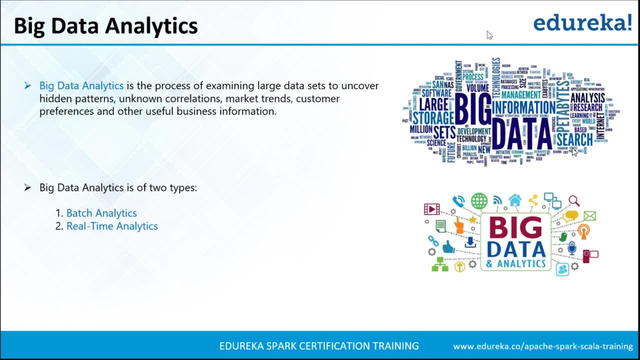 am using the surname as well- what that means. that means that I have the more data, so more data means I will be generating more accurate reports. more data means I will be generating more accurate reports. right, so yeah, now what do we have? so the now, because we do have huge amount of data, and if 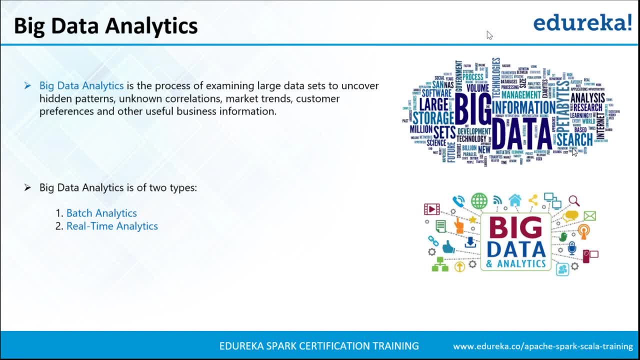 we do the analysis on this huge amount of data or on big data, there is a high probability that we will be making accurate predictions or we will be generating accurate reports which will help us in serving the customer better and eventually we'll be able to make more profit. so that's why each and 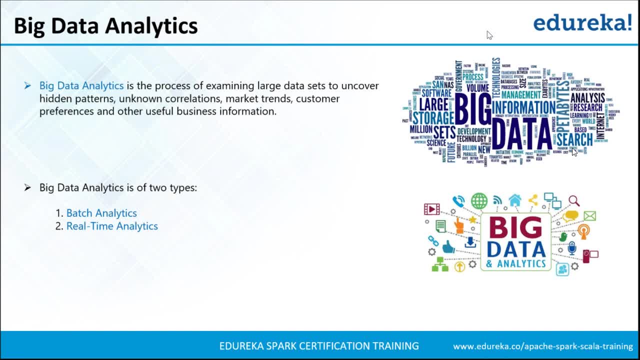 every organization is interested in doing the analysis on huge amount of data, and we call that as big data analytics. okay, and now, when it comes to big data analytics, this analysis can be done in two ways, or basically. basically there are two types. so what do we have? basically, there are two types. 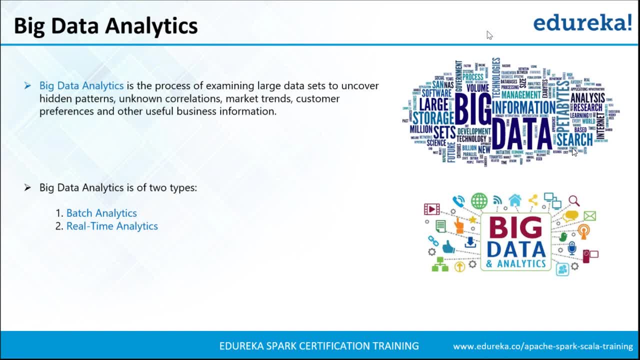 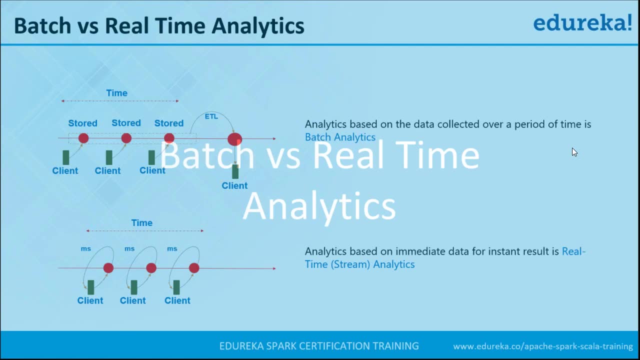 one is batch analytics, another is real-time analytics. what do we have? we do have two types. one is batch analytics and another is real-time analytics. so let's understand the difference between batch analytics and real-time analytics. okay, so batch analytics as in. if you look at this, 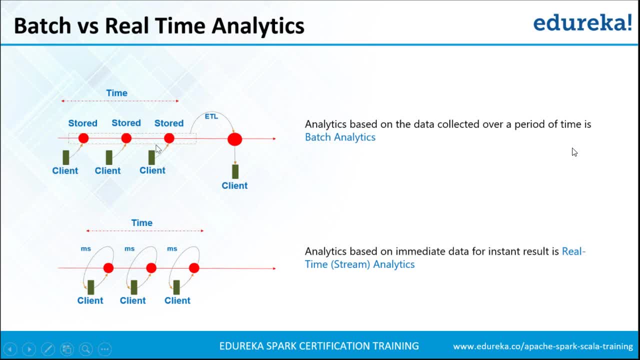 image. right, it says that client is giving the data at different, different intervals. okay, and what we are doing? we are storing the data. let's say that client has given the data at 8 am in the morning, we stored it. then client is giving the data at 10 am. we have, we are storing it. and then at 12 pm, we are storing it. but what we are doing? 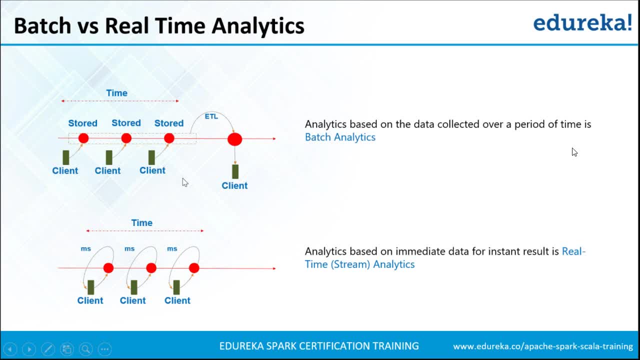 we are not processing the data as soon as we are receiving it from the client. what we are doing? we do have one etl job running towards the end of the day, let's say 8 pm. what it will be doing is we are doing. it will be performing some calculations and it will try to find out the meaning out of the. 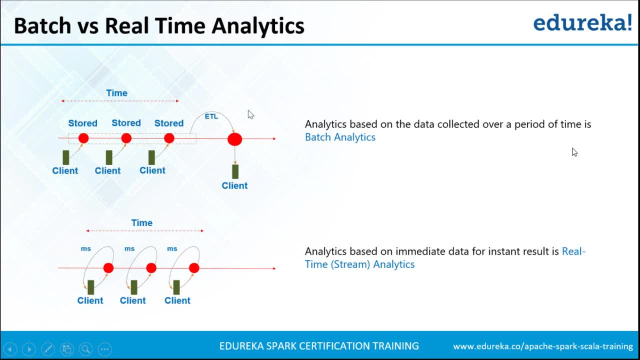 data. so what is it? this is nothing but type of batch analytics, as in, you are not processing the data as soon as you are getting it, you are just storing it and then, at later point of time, you are doing the processing on it. okay, then what do we have? we do have real-time analytics, so what do? 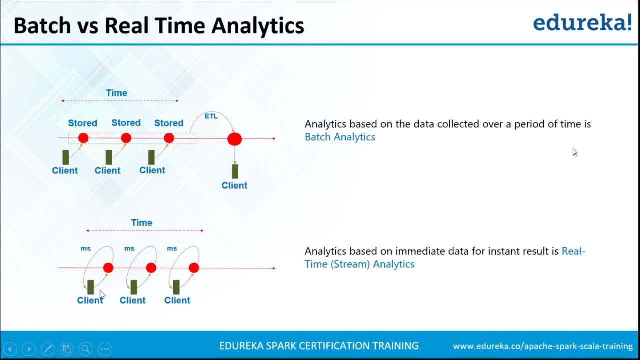 you see, here it's like as soon as we receive the data from the client, right job is done: running for the processing. so it's not that that we are collecting the data and then we are saying that the end of the day will be generating the results. so what is this? this is nothing but real. 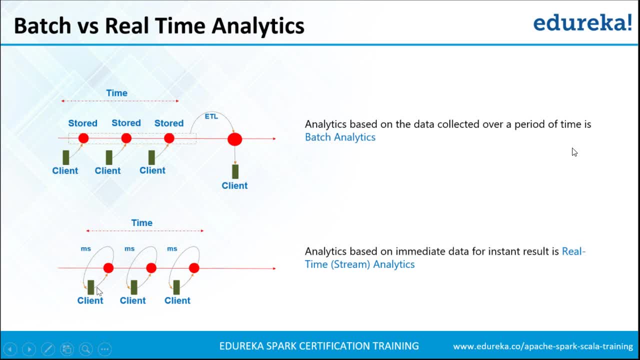 time analytics. so now here, when we talk about real-time analytics, right, the best example is online uh transactional system. so whenever you swipe your card on the pause machine, right so you should be getting the response within seven seconds. so, basically, for the payment gateways, SLA is of seven seconds, so within seven seconds you should. 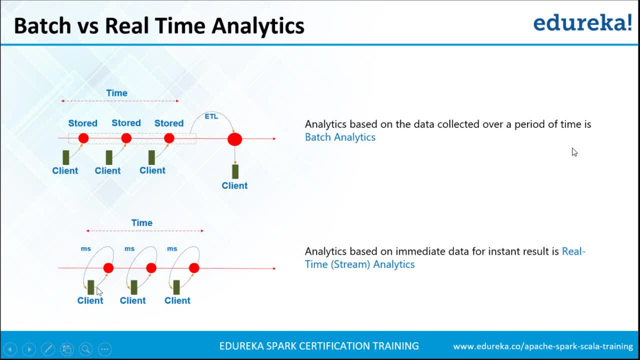 get the acknowledgement if your transaction is approved or rejected. so it's not that that visa as a payment Gateway saying that I have a VR. as of now, we are collecting the data from all the customers. at the end of the day, we'll be running the job and then, at the end of the day, you'll get. 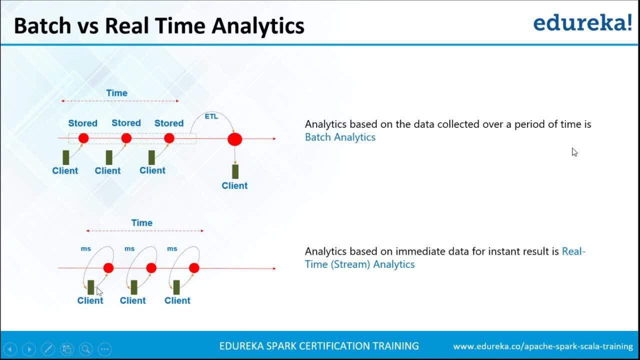 to know if your transaction is approved or rejected, right? that's something which is not happening. so as soon as payment Gateway- Visa, MasterCard- they are receiving the data, right, they should be doing the processing on that data to approve it or to reject it, and also they need to run the fraud detection algorithm as 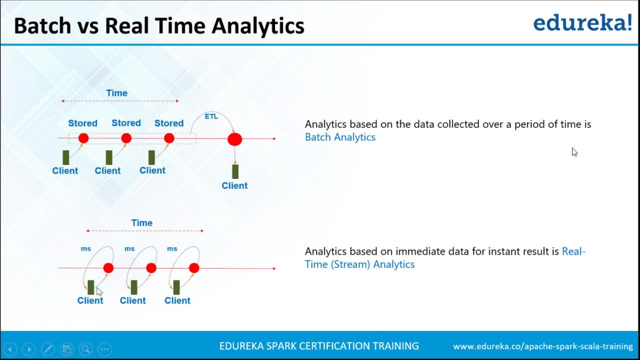 well, right, so this is what the example of real-time analytics is, but actually, in practical, there is nothing right like real time. right, so as an, it will always be near real time. so I'm taking the example of online transaction system. right, so it's like we do. they do have a SLA of. 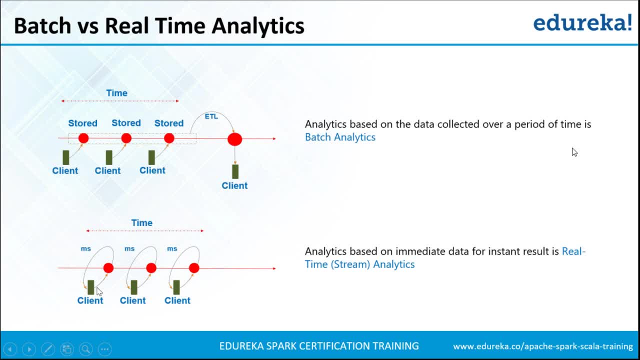 seven seconds, right, so there is some delay of seven seconds. it's not real time, it's near real time, okay, so always there will be some delay, right? Ravi says fraud detection is not part of ML. it is part of ML, but, Ravi, before they send you the acknowledgement, if it is approved or rejected- 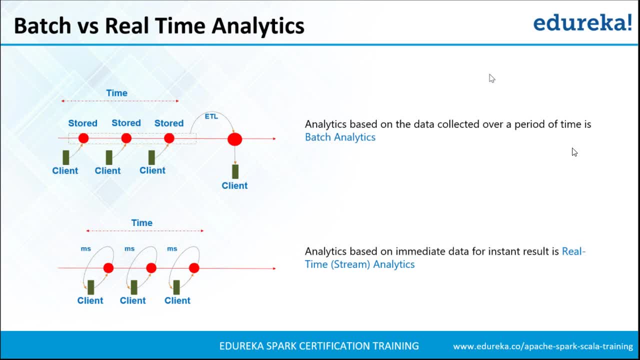 they need to run this fraud detection algorithm as well. so they do have this SLA of seven seconds, right? so within seven seconds, data. let's say that you are in India. Visa has got a data center in US, so within seven seconds your data needs to travel to. 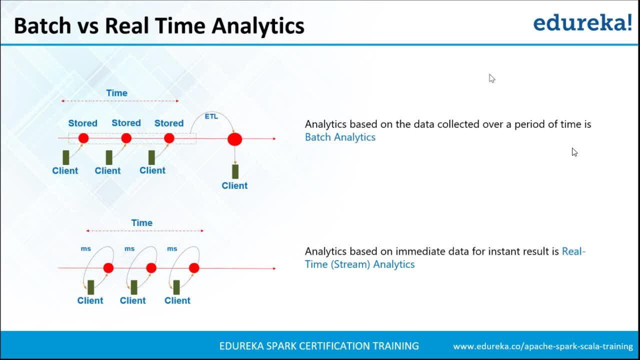 US, and meanwhile it should run a fraud detection algorithm as well to check if it is a fraud detection, fraud or transaction or not, and then, accordingly, they will be sending the response. so the point is, we do have very less time to process this data. it's not that that we are. 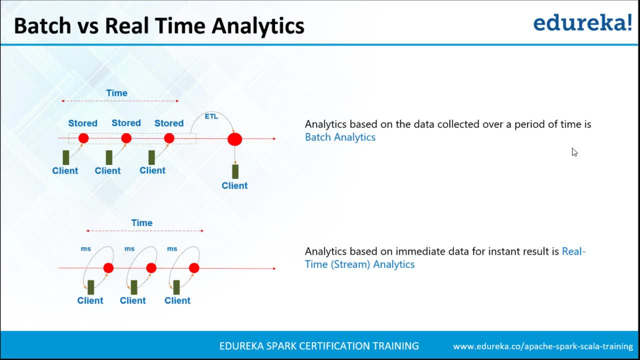 saying that, okay, we are visa, is saying that we have collected it and the end of the day will be processing it. okay, okay, six seconds is the time Spark takes. so, basically, what do we? SLA is uh, SLA is of six seconds, right, so they will, you know, they will tune the performance and they will check if Spark is. 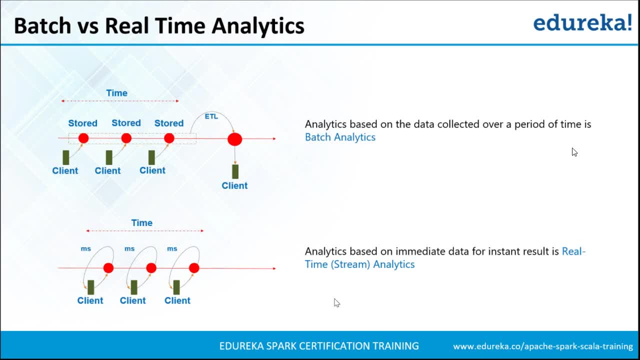 able to, uh, give the results or not, otherwise they'll have to use the accelerators and all to increase the processing speed. okay, so here we are not talking about spark as of now. I'm just taking the example of real-time analytics, like: what is it in actual? okay, so, guys, is it clear? 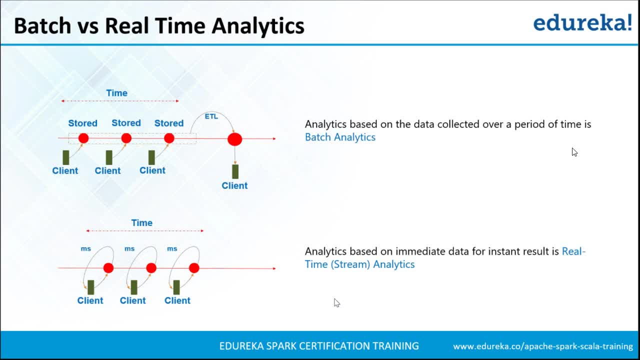 any questions how tuning is done. in fact, that's again a detailed discussion. okay, but as part of this webinar we do not discuss any of this. some things in detail, but when it comes to the performance tuning, we use persistence, we use the partition collapse. those are again the advanced. 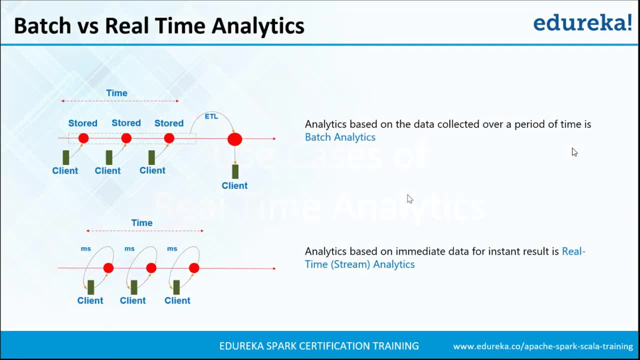 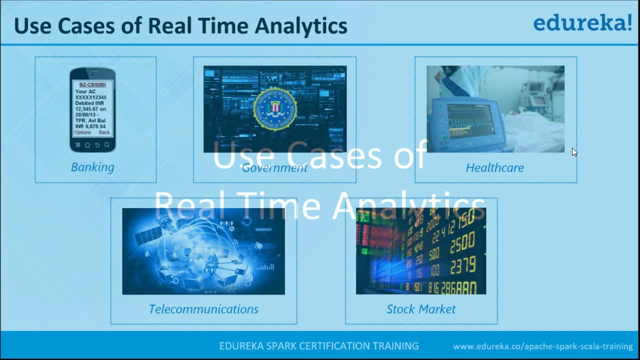 concept. okay, so let's move on. so now, use case of real-time analytics: banking, government health care, telecommunications, stock market- what are these? all these are examples of real-time analytics. okay, now we need to understand that. why to? why to use spark when hadoop is already there? 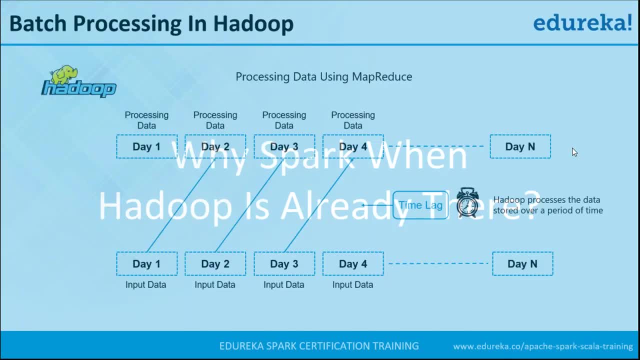 so, guys, for processing this huge amount of data which has got varieties and also which is getting generated at a very high speed, we already have a framework which is known as hadoop. okay, and if we compare the performance of hadoop with the legacy systems, hadoop is 100 times faster. okay, it's already there, so now the 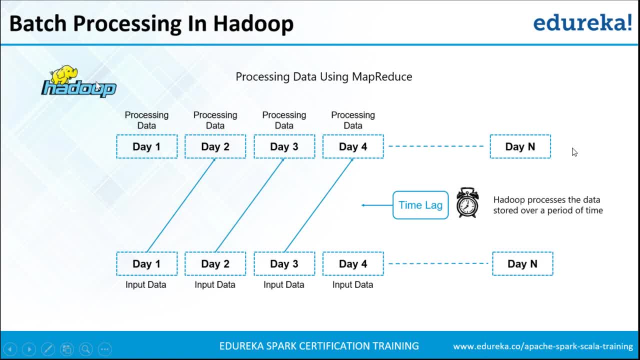 question comes: if we do have a framework already which is designed specifically to store and to process big data, why there is a need to use spark. okay, and that's what we'll be discussing now. so, guys, basically, when we uh talk about hadoop- right, so what we say? we say that it is designed to do the analysis on the batch data, and you know what. 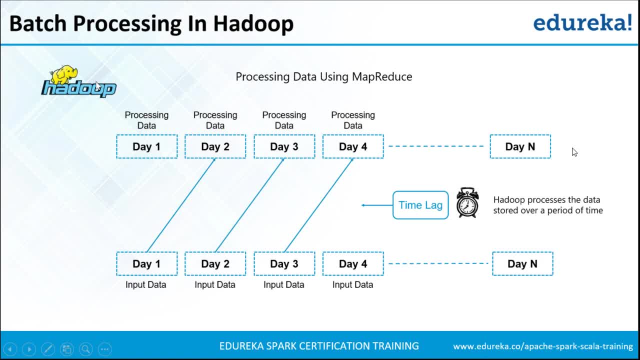 is batch analytics. as in, we will be collecting the data over a period of time and then we will be doing the analysis on that. as in, we are not in hurry to generate the results right, and hadoop is best for that. it's like how hadoop is different from other legacy system. 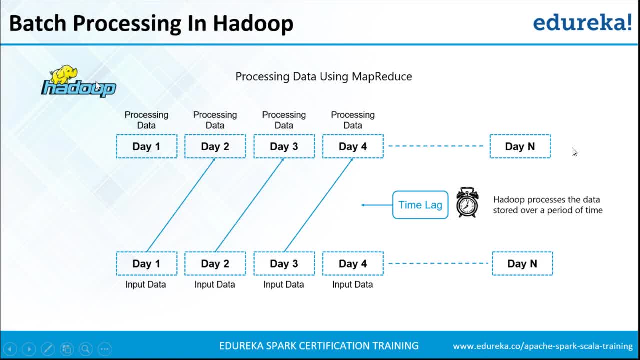 hadoop can handle any kind of data. okay, so it's not like rdbms, where rdbms says, or sql server says that we will be- uh, we will be- processing only structured data. okay, so hadoop says that you know, i can handle any kind of data, any type of data, and also it is 100 times faster than 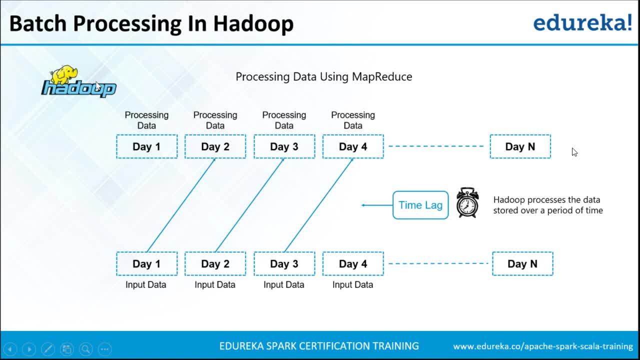 other legacy system. but the drawback of hadoop is it is designed to do the analysis on the batch data, as in on the data which is coming at regular intervals. okay, so yeah, what it does it? it processes the data stored over a period of time. now, when it comes to spark, right, so we are saying that you know this time lag is not acceptable. we. 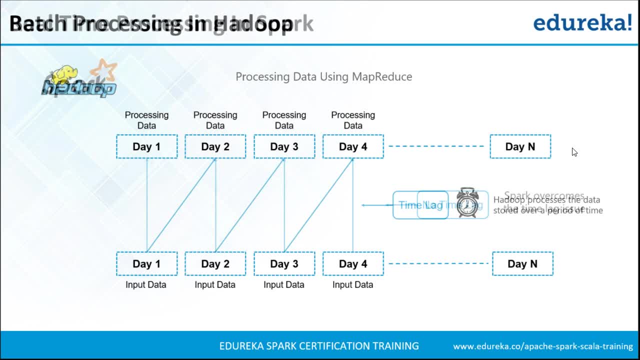 are entrusted in getting the results as soon as we get the data. so in that case, hadoop will fail, and the reason for that is hadoop always reads and writes the data to and from the desk. okay, so now this huge amount of data, it will be written to the disk and again, this huge amount of 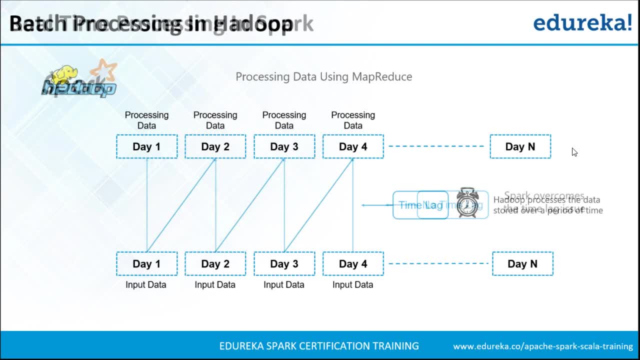 data, it will be read over the disk. so, because it is doing reading and writing to and from the disk, right, that's why it is always slower. because it is being reading and writing to and from the disk, that's why it is always slower. fine, so now when it comes to spark, right, spark has overcome. 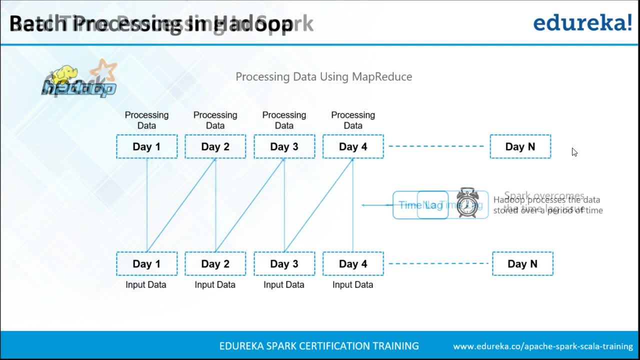 the limitation of hadoop and it says that i am capable of doing the real-time processing. spark is saying that i am capable of generating the results quickly and it's 100 times faster than hadoop. faster than Hadoop. and how it does that technically it is doing the in-memory processing, So what? 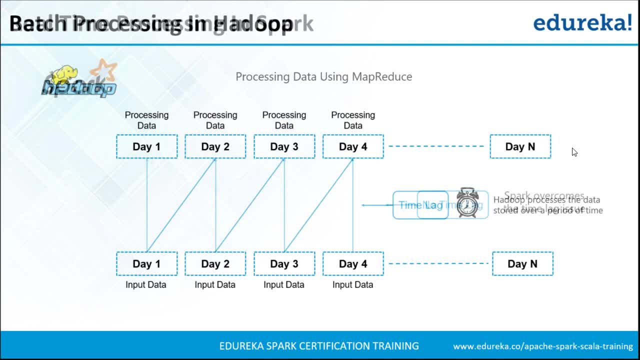 Hadoop was doing. Hadoop was always reading and writing the data to and from the disk, but when it comes to Spark, what is it doing? It's reading and writing the data to and from the memory, and you know right that whenever, like, we cache something and if you try to process it, 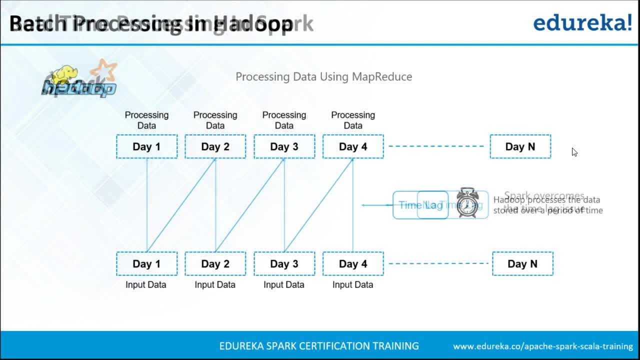 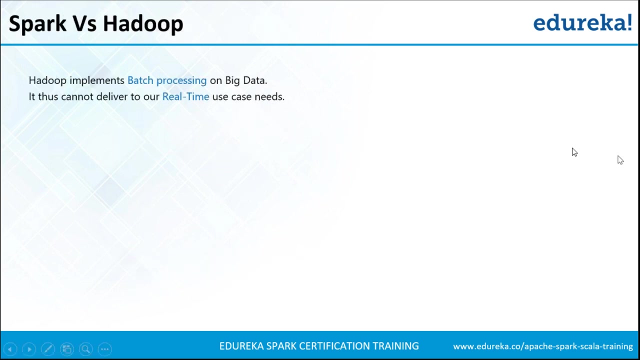 we will be getting the results at a very high speed. So, guys, is it clear? any questions so far. Any questions so far, anyone? Okay, I don't see any questions coming, so let's move on. Oh yes, I have a question from Ashutosh, and the question is: what is the best for health care system? 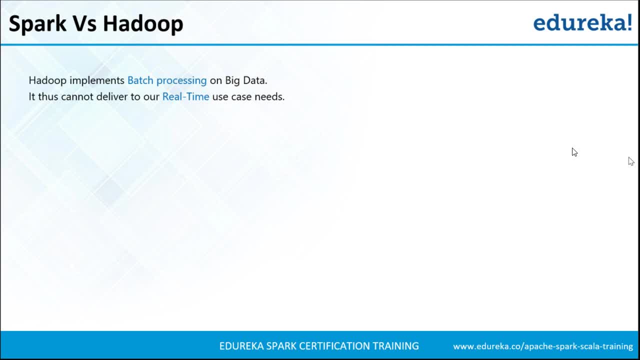 So it will depend on the use case, like: what is your use case? So now, let's say that you know you have a smart watch and it is reading your heartbeat and everything, and what is the use case? we are saying that it should be sending the notification to the doctor immediately, as soon. 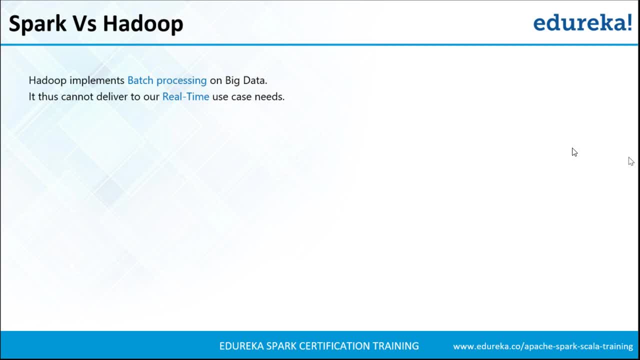 as your heartbeat or you have an abnormal heartbeat. So that's the example of real-time data collection. So basically, it's your data can be done to the, the data is getting collected and at the end of the day will do the analysis and will say like if the heartbeat is abnormal or not. 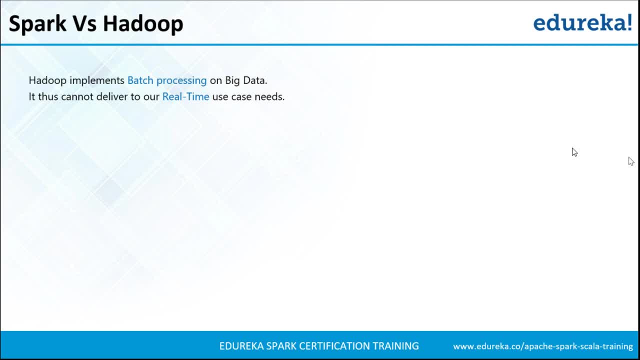 So it will always depend on the use case, what you have. So now one example, okay Located, if I take example of Facebook. so now, whenever you load your profile right, or whenever you log into your Facebook profile, it should have the notification that superpower failed. 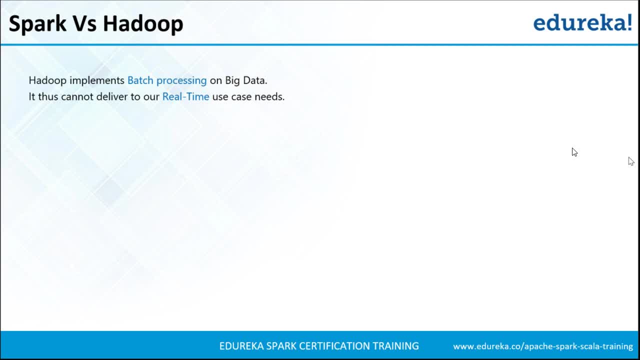 Okay, what training are you going to do? It should be training so that after you register for nano才, what do you think? what should be the priority for Facebook? to show the friend suggestions or to load the profile with the latest feed? to show the friend suggestion or to load the profile with? 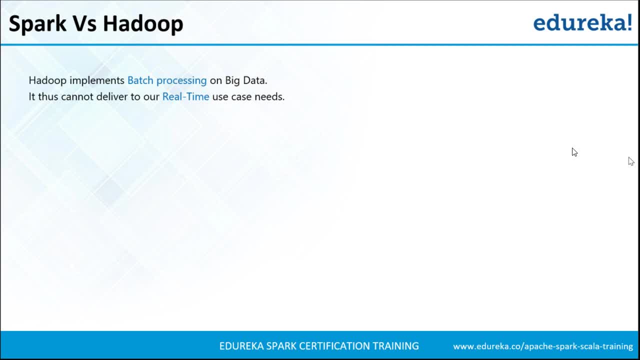 the latest feed. it's basically to load the profile with the latest feed, right, because friend suggestions are something which can be shown or which can be displayed after 10 minutes as well. right, that's completely fine. so now, when it comes to spark what it is doing, it is doing the in-memory processing. 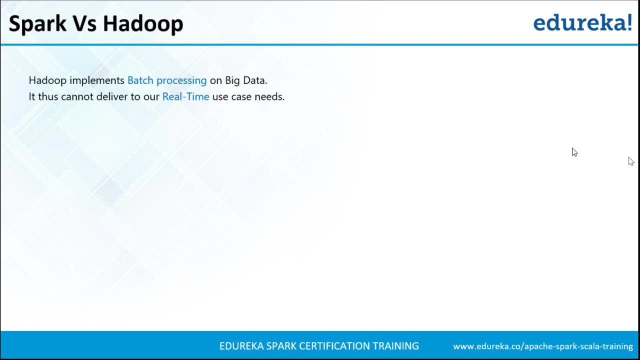 in-memory processing as in, we need more RAM. more RAM means it is expensive, more RAM means it is expensive. so Facebook is saying that if there is something which we can achieve by spending less, why to spend more? so for showing the friend suggestion, Hadoop or MapReduce is being used. 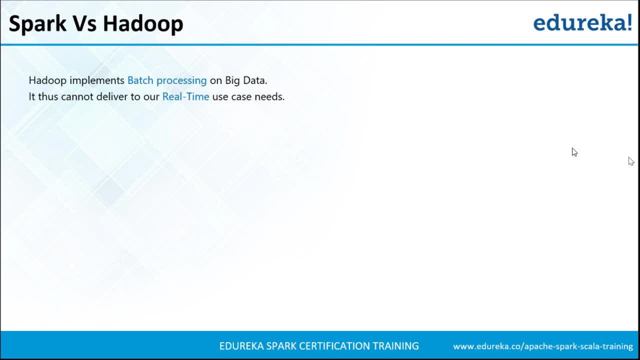 and for loading the profile with latest feed. spark is being used, right. so, similar way, if you take example of any domain, like if you talk about healthcare domain, right, so now let's say that you do have patients historical data, right? so that is something like which can be done using batch analysis as well. so it will always depend on the use case. 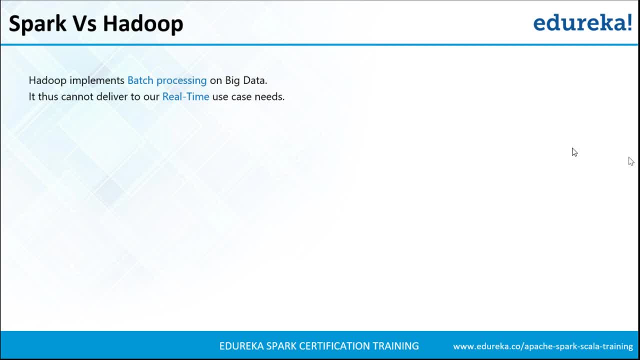 case and based on your need, you will be choosing. we are not saying that spark has replaced Hadoop. no, based on your need or based on your use case, you'll be choosing and that's why we are saying that for batch analytics, Hadoop is the best, but nowadays we are saying that we do have use case. 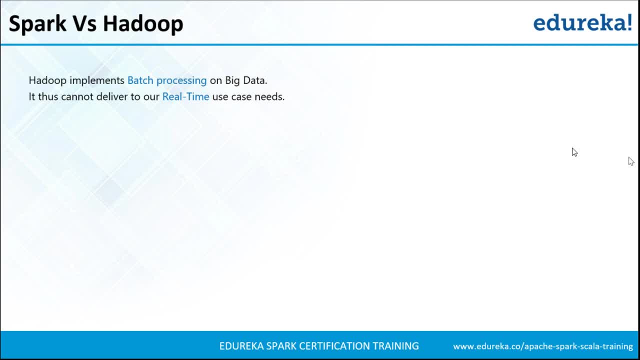 where we are interested in implementing real time analytics. that's where we will have to use spark. okay, okay, so yeah, is it clear to all? okay, so what do we have? we do have Hadoop, which will be implementing the batch processing, and then Spark, which is for real-time use case. We do have batch processing and then we do have 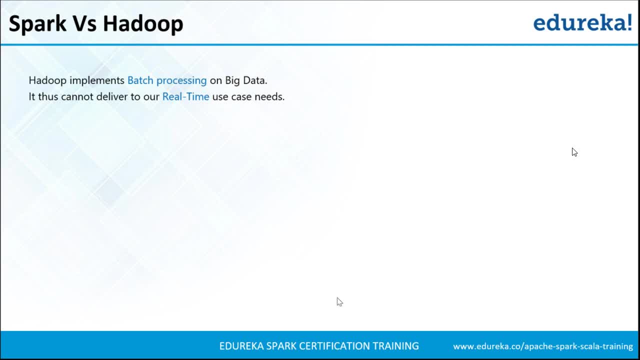 Spark for real-time use case. Okay, So now let's say that our requirement is to process the data in real-time and to handle the input from multiple sources, and which should be easy to use and which should be there for fast processing. What we'll be doing, we will. 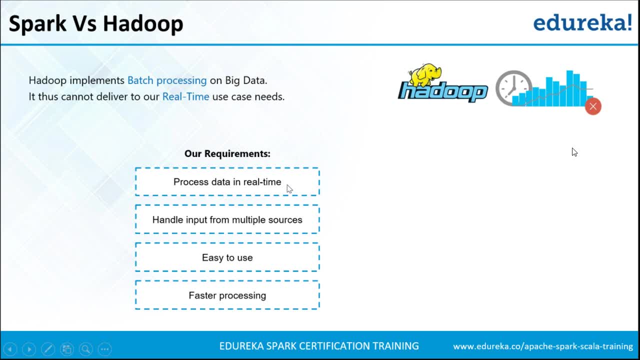 be using Hadoop, but not for all, As in, if we are using Hadoop, Hadoop says that I'm not capable of processing the data in real-time, I'm not easy to use and also I'm not capable of doing faster processing. When we say faster processing, right. So it depends like what. 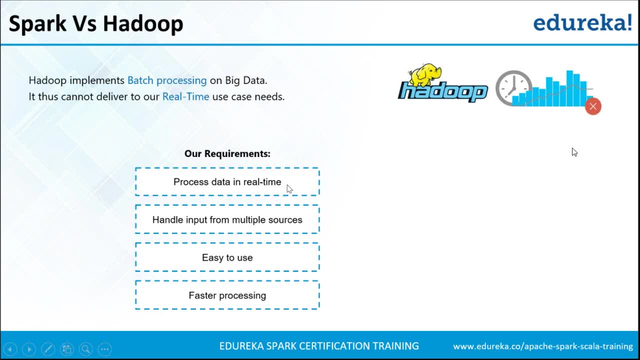 is your requirement. So, in a way, Hadoop is faster than legacy system, or it is faster than your SQL or RDBMS, but based on our need or on use case, we'll be saying that it's slower. Okay, So yeah, Hadoop says that I can handle input from multiple sources, but 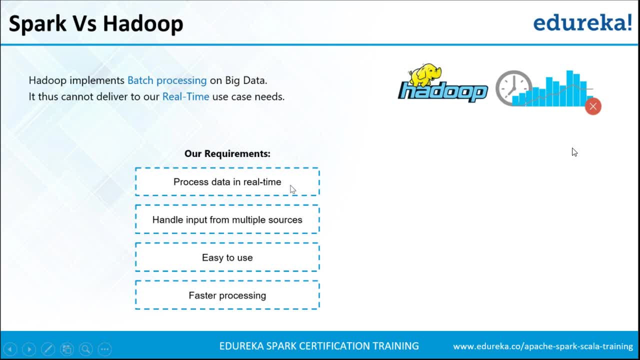 when it comes to Spark. Spark says, Hey, I'm not capable of processing the data in real-time. okay, Not to worry, I am capable of. I'm capable of serving all the needs, which is, I can process the data in real-time, I can handle input from multiple sources. I'm very, very easy. 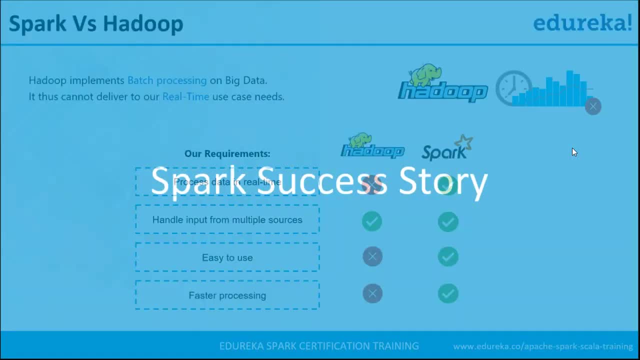 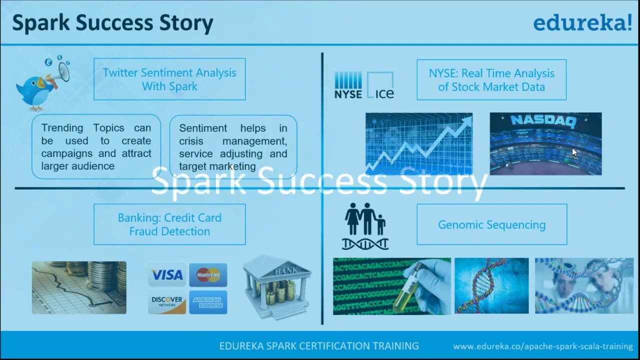 to use and I'm much faster than Hadoop. Okay Now when it comes to Spark success story. so basically, Spark is being used for doing the sentimental analysis on Twitter, as in right? So as in whenever someone is tweeting something on Twitter, right? So you are interested. 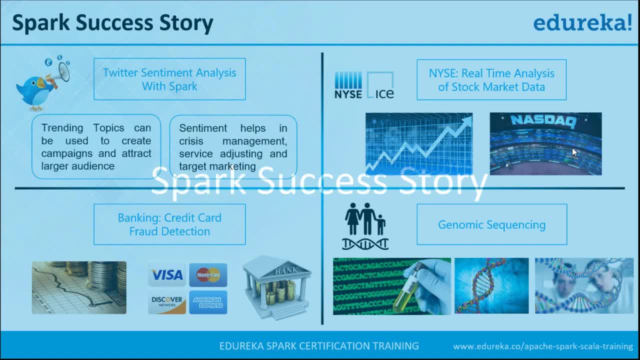 in knowing if that's a positive feedback or if that's a negative feedback. So what you will be doing, you can use Spark, or Spark is being used. So, going forward, you'll understand that. you know how do we do the analysis on live data Or how do we do the analysis on 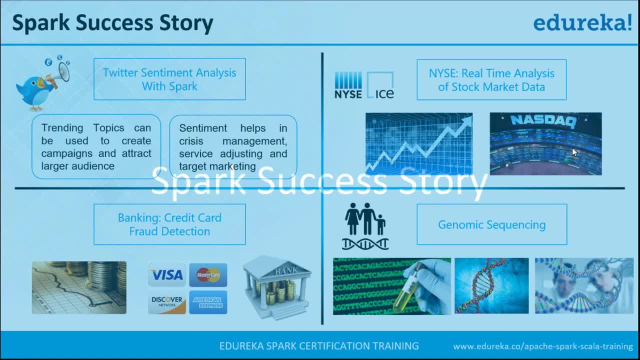 real-time data using Spark And then when it comes to New York stock exchange, basically when it comes to real-time analysis of stock market data, again Spark can be used. and when it comes to banking domain for credit card fraud detection, spark can be used. and 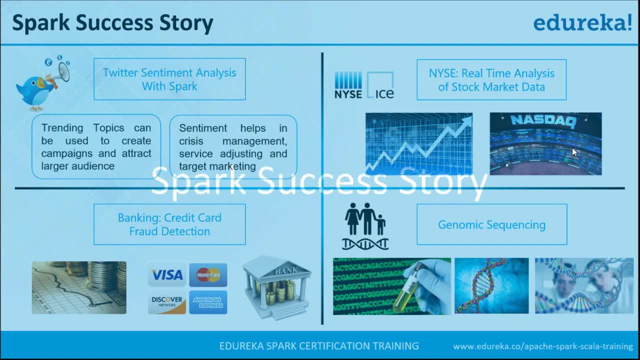 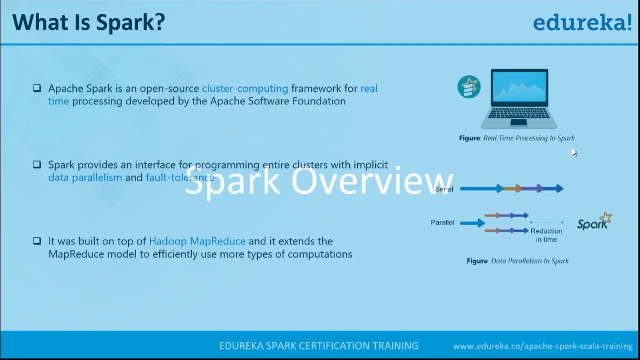 and then for genomic sequencing. again, it can be used. okay, so now spark overview. so what is spark? again, it's an open source cluster computing framework as an internally it will be running over n number of machines and this is from apache. it is open source, you can always download it and you can start using it. and also it has got. 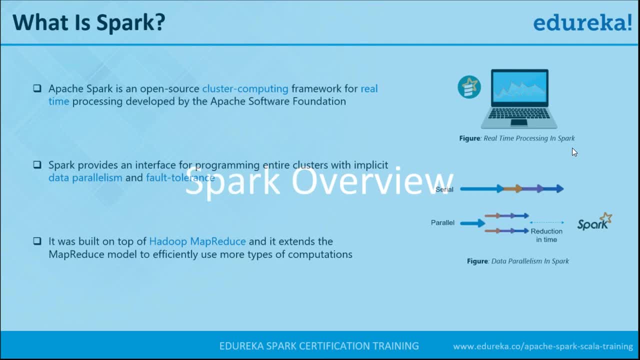 an interface for programming entire cluster with implicit data parallelism. implicit data parallelism as in. you don't need to tell it, like how to distribute the data or how to split it or how to run the parallel jobs. that's not something which you will be doing as a developer. these 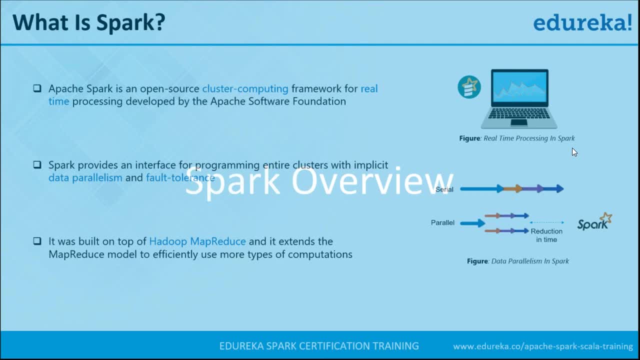 are the things which are being handled by the spark framework internally. these are the things which are being handled by the spark framework internally. and also, it was built on top of map reduce and it will extend the you map reduce model. uh, so what do we have when it comes to hadoop? right, we do have a processing. 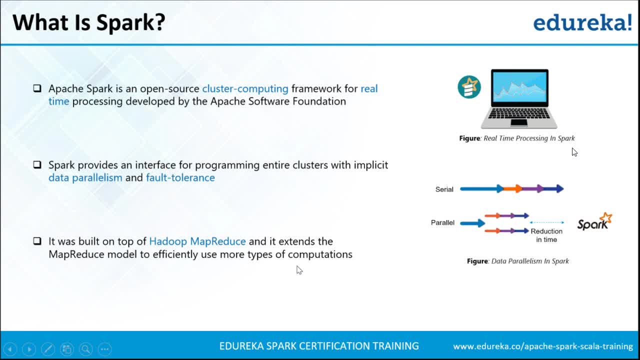 engine, which is by the name of map reduce. so now, when it comes to spark, right, so we say that again in the similar way. it will be following the concept of distribution and of parallel processing, but uh, but it's the spark. is the advanced version? okay, and the integration of hadoop is possible with. 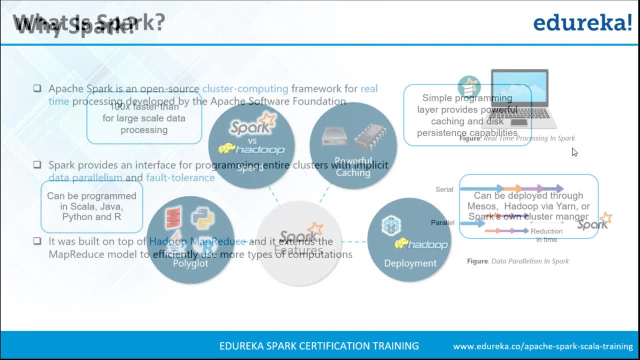 map reduce. and now, why is spark so? first of all, it is faster. it is 100 times faster than the large scale data processing. okay, it is 100 times faster than hadoop. then it does the in-memory processing, or it will be doing the powerful caching, and then it is polyglot, polyglot. 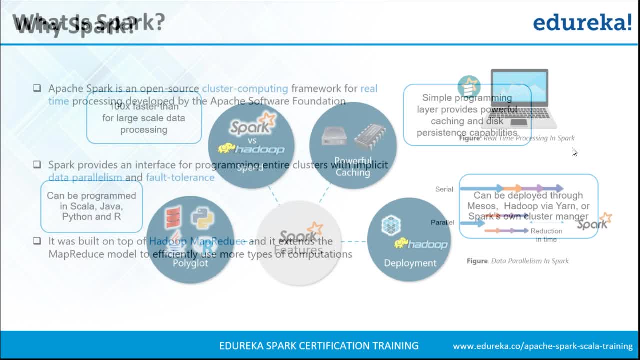 as in when it comes to the implementation of business logic. polyglot, as in when it comes to the implementation of business logic, so that business logic can be implemented using any of this programming language. okay, so basically it can be done using uh, java, python or skella. okay, you can use any language to implement the business logic. 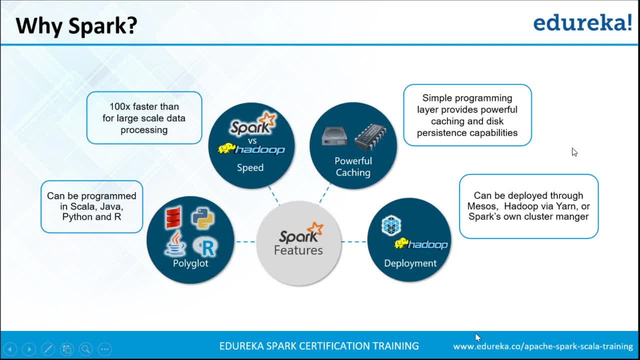 and also when it comes to the deployment. there are different, different modes for deploying spark. so, as in uh hadoop, can it? spark can be deployed through mesos means. so again, it's a, it's nothing, but it's a framework for cluster management. it can be deployed by a yarn, as in yarn can be used. 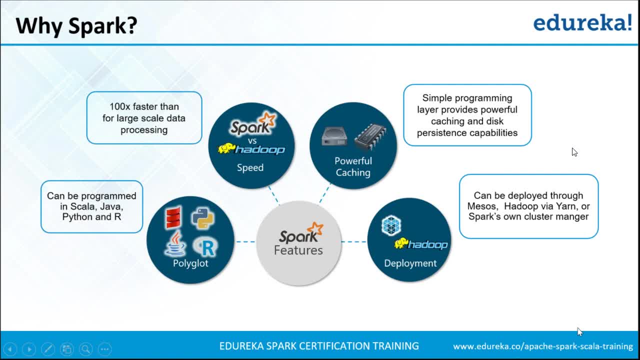 for cluster management, or what it can do, is it? it is having its own master as well, which will be managing the complete cluster, but most of the time, spark will be deployed through yarn. okay, so if you have worked on yarn, you will already be knowing like what does it? 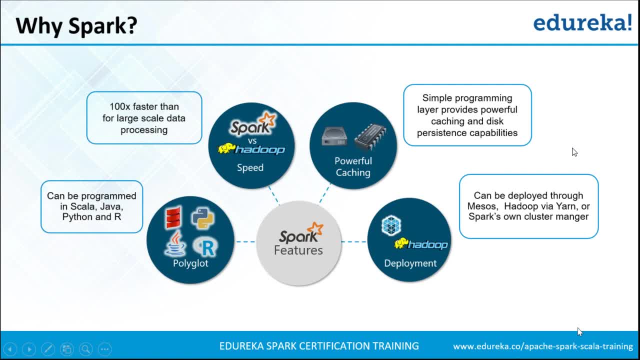 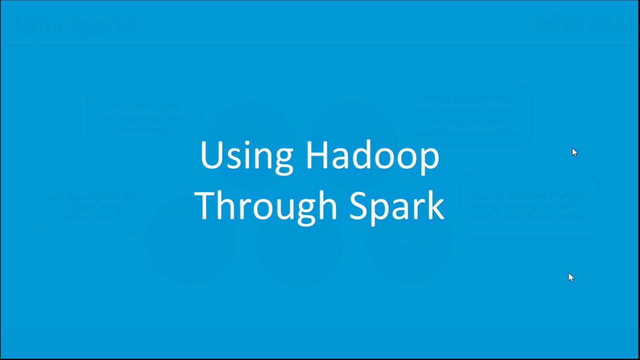 so the same yarn is being used here as well. okay, guys, are you? are you good? so far, any questions? so any questions, anyone? okay, i don't see any questions coming, so let's move on. so let's understand, like, let's say that in your cluster right, hadoop is already being used, so now we will understand that, how the spark can. 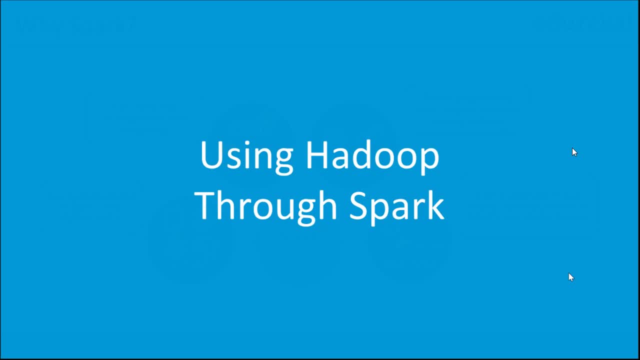 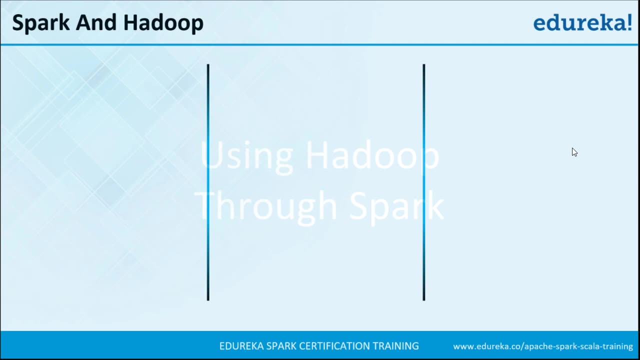 be used. so if hadoop is already there, so how the spark can be integrated? okay, so now when it comes to spark and hadoop, right, so what is spark, guys? so spark is nothing, but it's a processing engine. okay, it's just an engine. it is not having any component for storage. 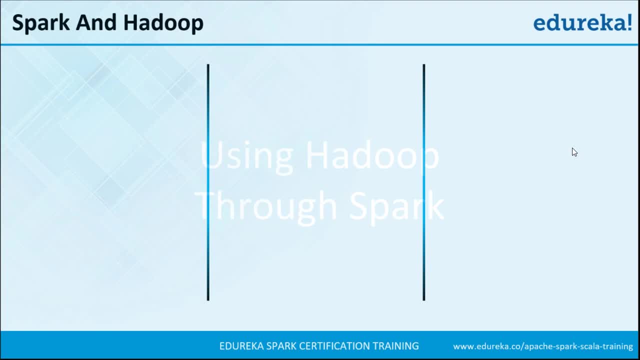 so, basically, when we talk about hadoop right, we say that it has got two core components: one is storage and one is for processing. but when we talk about spark right, we say that it is not having a component for this. but when we talk about spark right, so we say that it is only for. 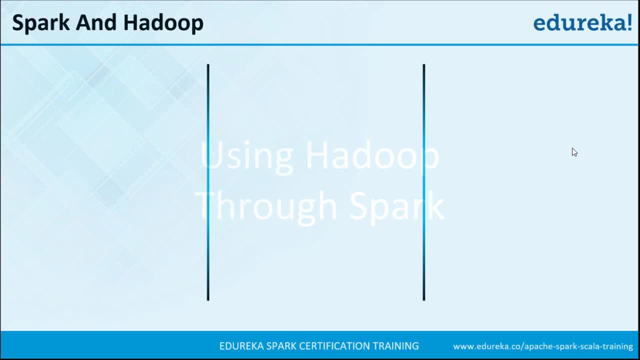 processing. so it is not having any component for storage. so what you'll have to do is always you will have to integrate it with a storage component. so most of the time we will be integrating it with hdfs. but, yes, it has the capability for the integration with amazon s3 or with ec2 or with 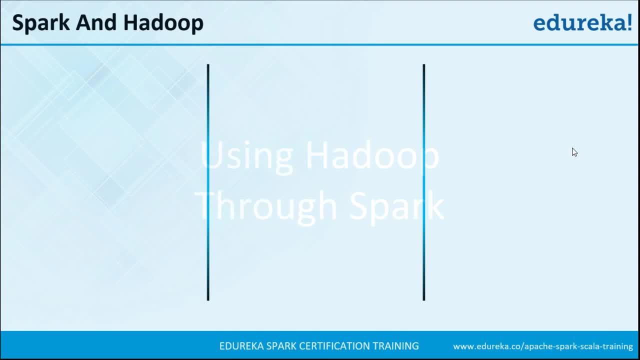 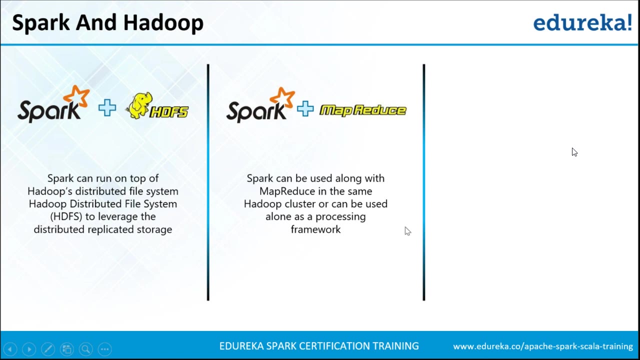 local file system. okay, but yeah, you will have to integrate it with the storage layers. you will have to do that, okay. now, when it comes to the MapReduce, I already took the example of Facebook, right. so I said that for showing the friend suggestion, I said that for showing the 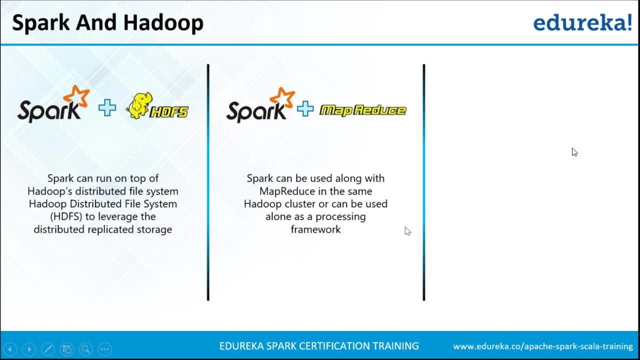 friend suggestion. MapReduce is being used and for loading the profile with the latest Spark is being used, so as in within the same cluster, all both the jobs can run okay. so if you are interested in doing the integration of Spark with MapReduce, both the things can. 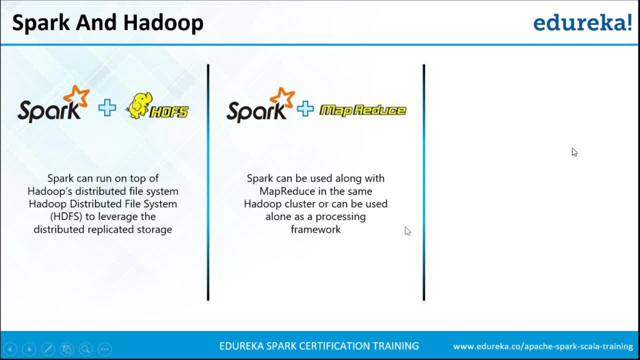 be done in the same cluster. it's not that that you need a different cluster. okay, then what do we have? we do have Spark with Hadoop Yarn. so, yeah, what is Yarn? Yarn is nothing, but it's a framework for cluster management, so Hadoop will be using this. 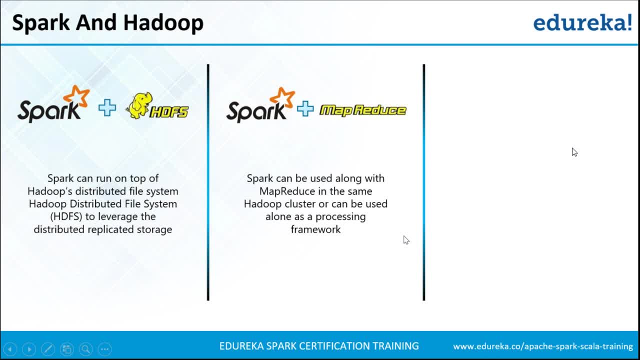 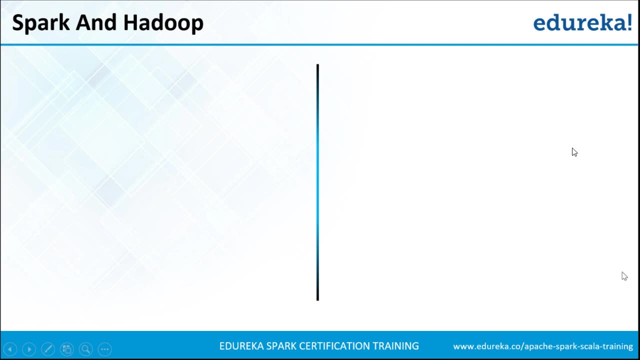 cluster management framework. again, Spark can also use the same framework, okay, so, yeah, integration of Spark with Yarn can also be done. okay, so now Spark and Hadoop. okay, so this is something which you need to understand, so you should not be thinking that Spark is designed to replace Hadoop, and I think this is something which we had already discussed. 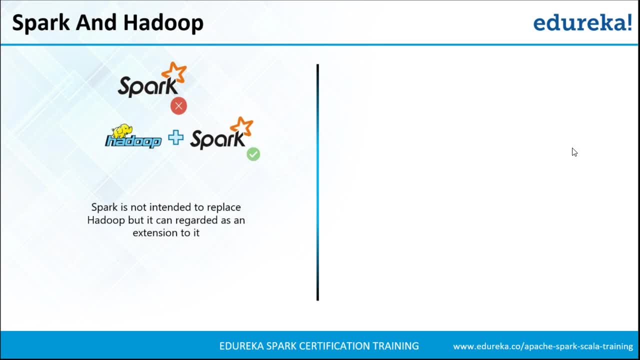 so it's not designed for replacing Hadoop, so Spark is serving a completely different purpose. our question is: Spark can not do clustering without Yarn. no, it has got its own manager for cluster management. it can do that, and it's not about clustering, it's about cluster management. 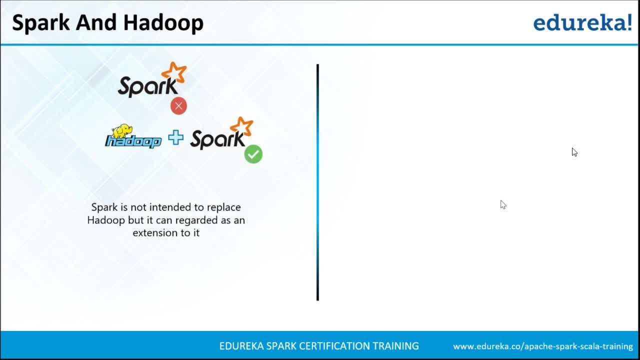 Ravi, and that cluster management it can be done using Mesos, using Yarn, or Spark has got its own manager as well, okay, so yeah, Spark is not intended to replace Hadoop and you know already, right, the use case will be different. so always it will depend on the use case or on the requirement. 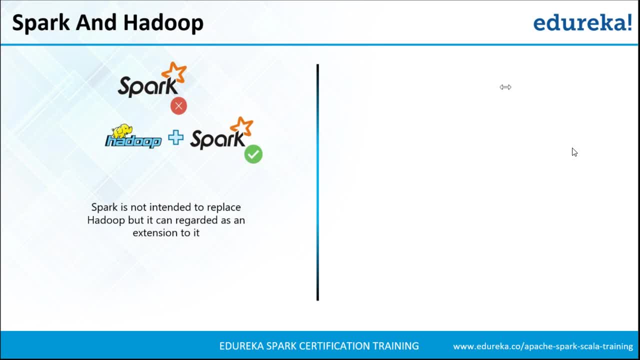 if it has, okay. I have a question: if it has at its own, why use Yarn? so basically, Yarn is the framework which was specifically designed for cluster management. it is having n number of extra functionalities, which is Spark's standalone cluster is having. so now Spark plus MapReduce- same thing which we had already discussed- that the integration. 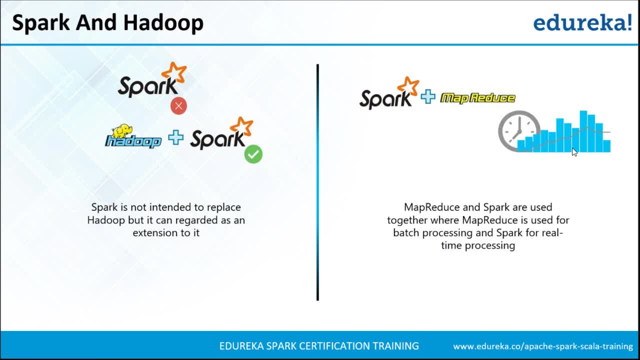 can be done based on your need or based on your use case. you will be using it, so now let's discuss the features. so let's discuss why Spark is so famous. okay, sorry, I forgot that. now, all of a sudden, Spark is a web-based platform, so you will be using it and it is. 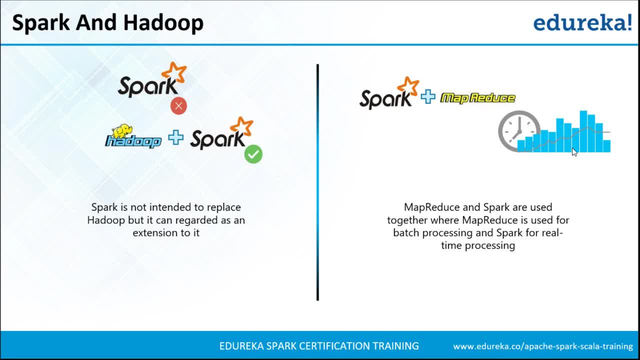 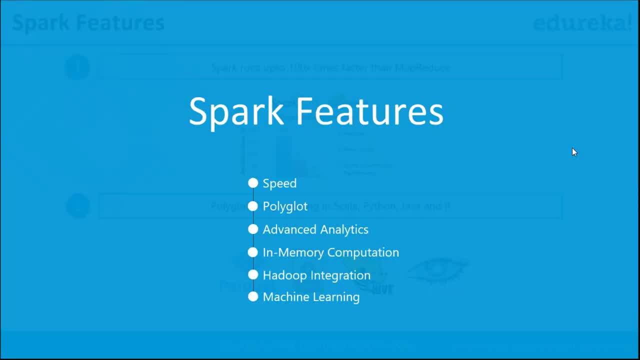 kind of a common concept in terms of that you should not do Yarn, then you need to do it before you start, even know it. it's not using it for the reason that I mentioned earlier, or why is it being used so widely these days? okay, first of all. first of all, we we talk about speed. 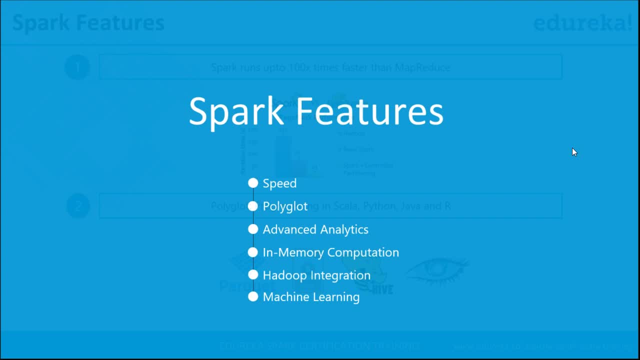 okay, it's 100 times faster. it will be giving the results at a very high speed. it's polyglot. as and when it comes to the implementation of business logic, hey, it can be done using any programming language. as in, you can use java, python or scala- any programming language can be used. 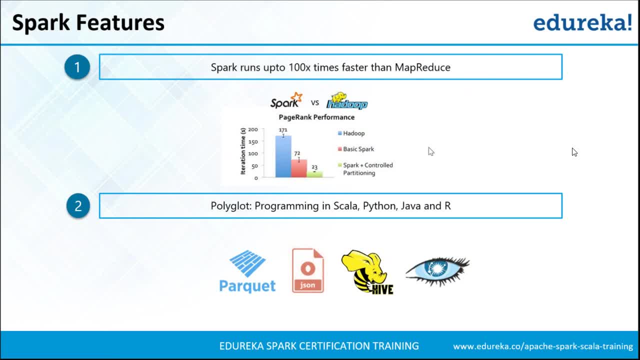 wherever spark is installed, yarn is. must i conclude that? no, that's what i'm saying, ravi. the integration is possible with yarn, apache, mesos and standalone. it's not that that every time with spark yarn will be used, but most of the time you'll see yarn is being used. 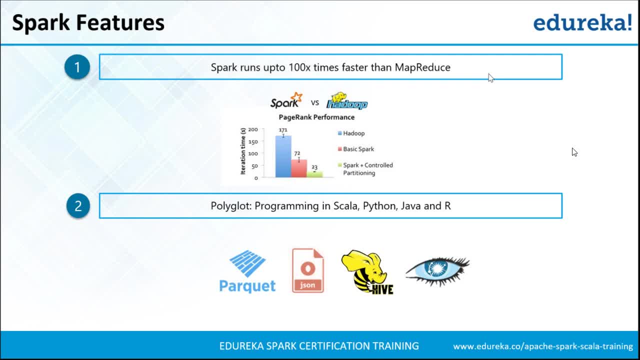 okay, so yeah when it comes to the features. so basically, it is faster and it is polyglot, as in we can implement. what we can do is we can implement the business logic using any programming language. then what do we have is so, basically, it does a lazy evaluation. and what do we mean by lazy? 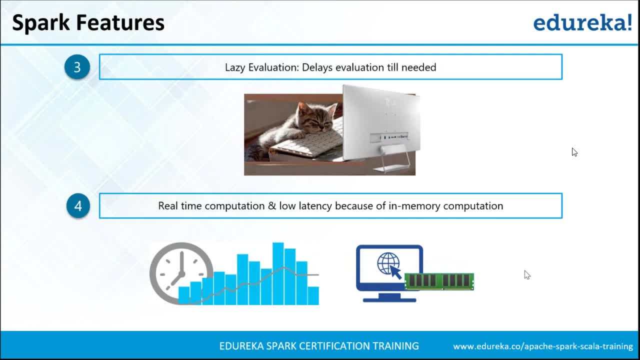 evaluation as in it's like, when you ask it to perform any action, right, what it will be doing, it will be storing the set of instructions, and whenever you ask it to give the results right, then only it will be executing those set of instructions. okay, it is. it does the lazy evaluation. 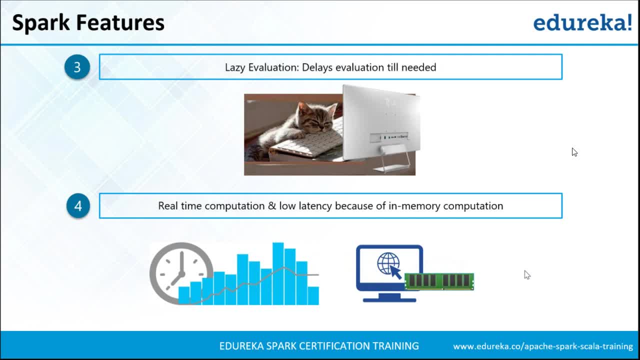 and the. but this you can save a lot of computation cost and also it does the real-time consumption and low latency, because it is doing the in-memory processing, so latency is very, very low. then integration is possible with hadoop. so if for your project hadoop is, 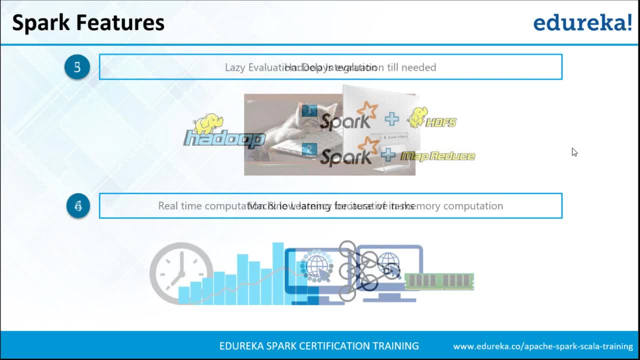 already being used, then, and if you are interested in getting migrated to spark, it's very, very easy, because in that case you'll you'll just have to do the integration of spark with hdfs, so you don't need to migrate your data and you need to migrate spark. you need to integrate spark with yarn again. 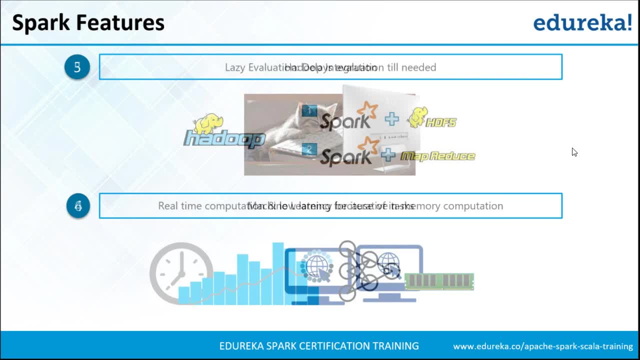 you don't need to use any other framework for cluster management, only for processing. you will be using spark and also it has got the capability. it has got the capability using which you will be implementing the machine learning algorithm, so you will be using the machine learning algorithm. 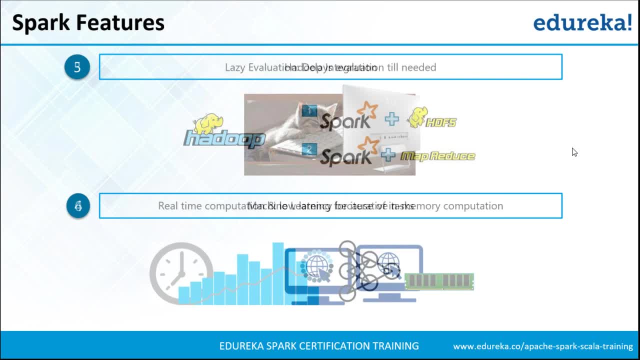 so iterative task, as in, it will be, uh it, what it will be doing. it will be, you know, accessing the same set of data again and again. so what happens in case of machine learning algorithm? so one algorithm will be running n number of time on the same data set to give the optimized model. 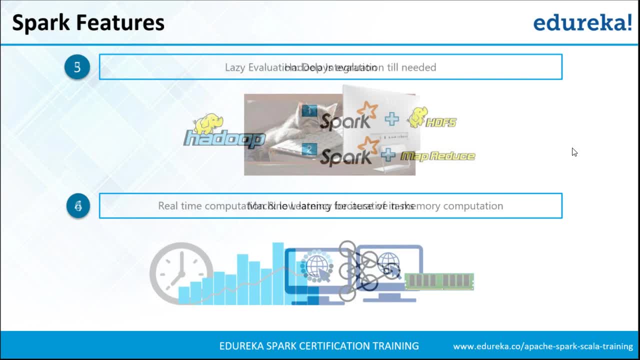 right. so now let's say that the the this data set is present on the disk. so what it will have to do is, every time it will have to read and write the data from the disk, every time it will have to read and write the data from the disk. so how spark is helping this park is saying that, hey, not to worry. 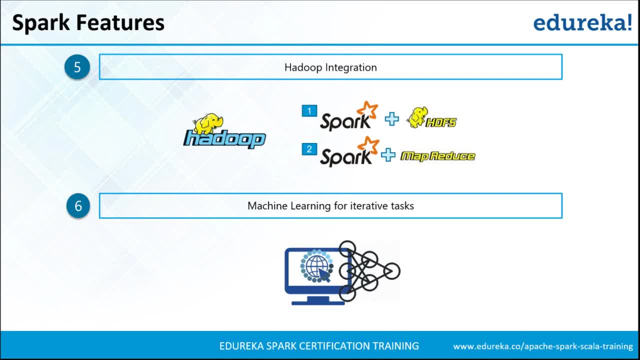 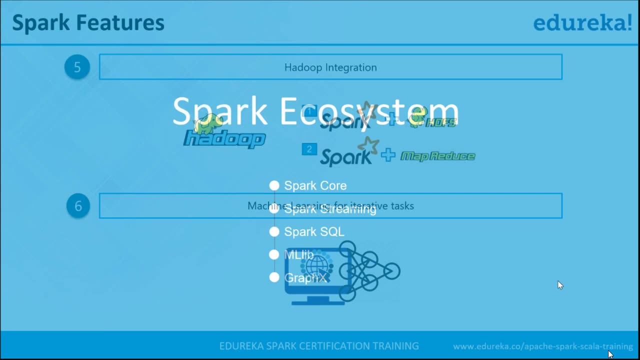 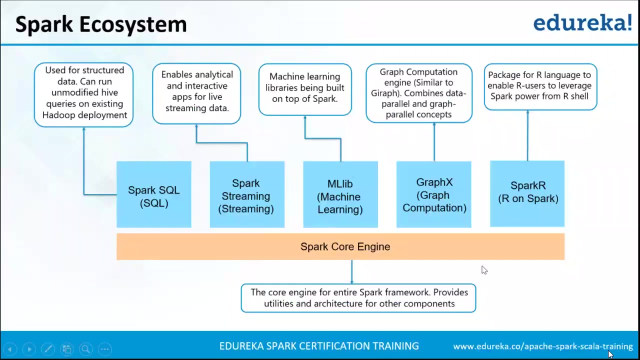 i'll keep this data set into the memory so that you don't need to read it every time from the disk. okay, uh, yeah, that's about machine learning. now let's talk about spark ecosystem. okay, so we will understand. like, what do we cover as part of spark ecosystem? okay, so guys, first of all, 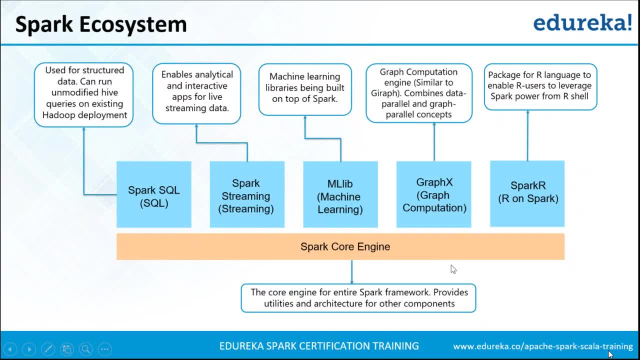 what do we have? we do have one core engine. okay, that core engine is nothing but spark core engine. so it is having all the- you know- basic utilities. it is having all the utilities and architecture. fine. so now on top of this core engine. so when we talk about this core engine, let's say that you are interested in implementing a business. 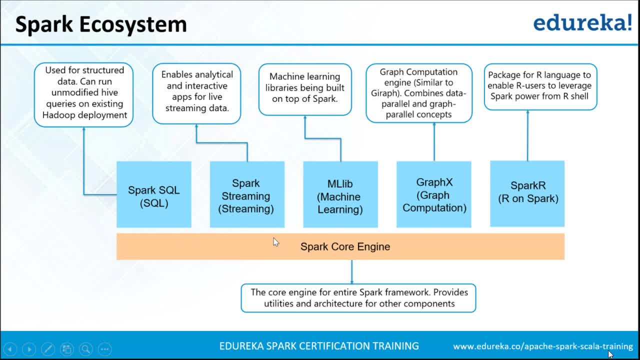 logic. so how will you be implementing the business logic? so you will be implementing the business logic by using a programming language, as in: you can use java, python, uh, scala. okay, you can use any language. if you are interacting with this spark core engine, you need to use a programming language. 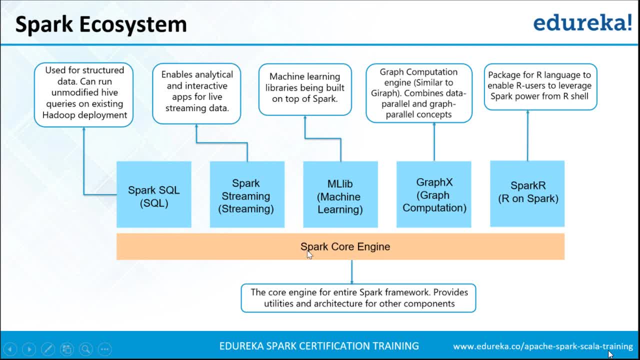 now let's say that you don't come from a programming background and you are saying that requirement for you is to do the analysis on real-time data. you are saying that you are saying that you don't come from a programming background. you are saying that you are saying that you are. 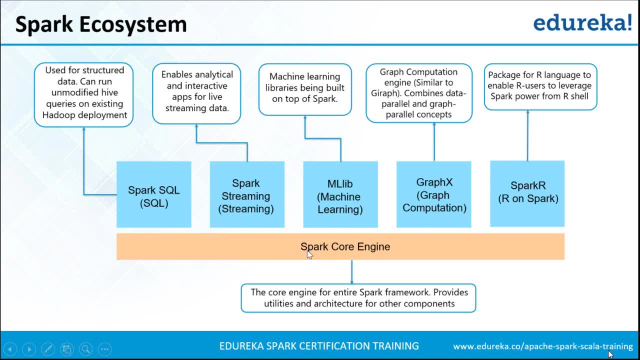 saying that you don't come from a programming background and requirement for you is to do the analysis on data. so now, if i take one example, as in, i have two kinds of developer. i do have a java developer and i have a sql developer- and i'm asking both the developers to read a table. 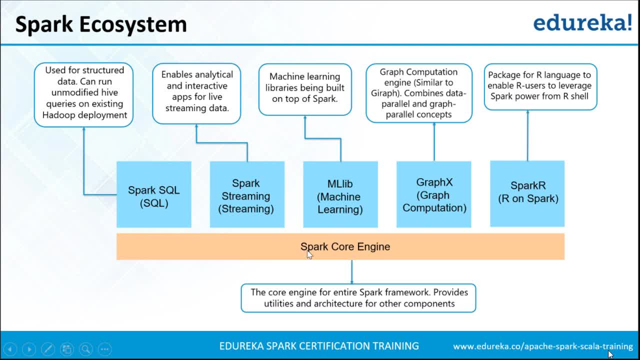 what am i doing? i am asking both the developers to read a table. so now, what do you think? who will be giving me the results faster? sql developer? right, because sql developer will just say: select, start from this table and that's it. on other hand, right. a java developer will have to write at least 10 to 20 lines of code, right, so? 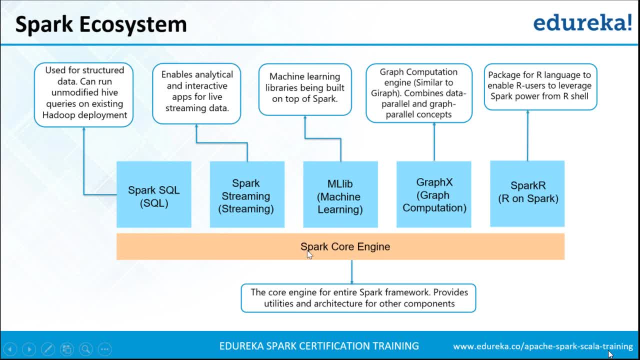 a java java developer will have to make the jdbc connectivity and then a java developer would be able to read the table and print it fine. so the conclusion of this example is: if we are interested in doing the analysis on the data right, it is very, very easy if we are using a sql like language. 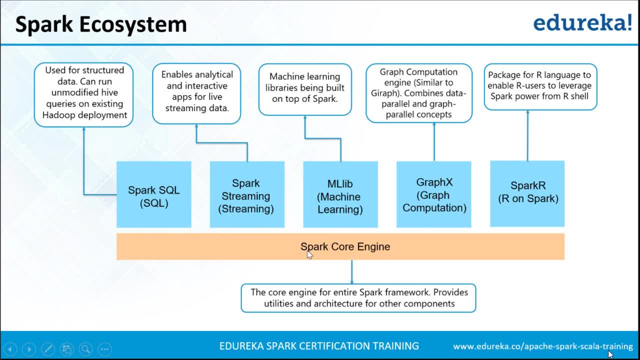 fine, and in today's world, 80 of the analysis on the data is being done using a non-java programming language. okay, so that's why what spark says, sparks says: hey, not to worry if you are interested in doing the analysis on the data and if you do not come from a programming background. 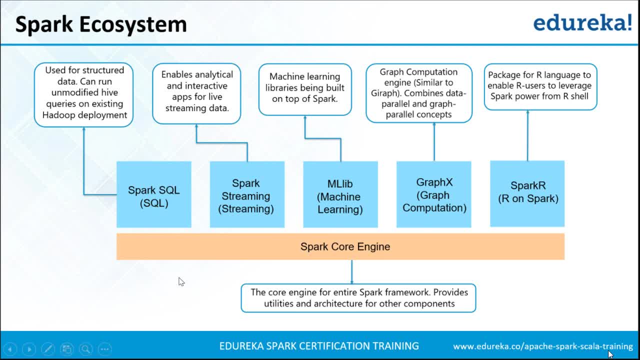 you can take help of this module, which is nothing but spark sql. okay. so what it says? it says that when it comes to spark sql, you will be able to write you. when it comes to spark sql, you will be writing sql like queries for doing the analysis. okay, and when we say sql, it means you can use it only to do the analysis. 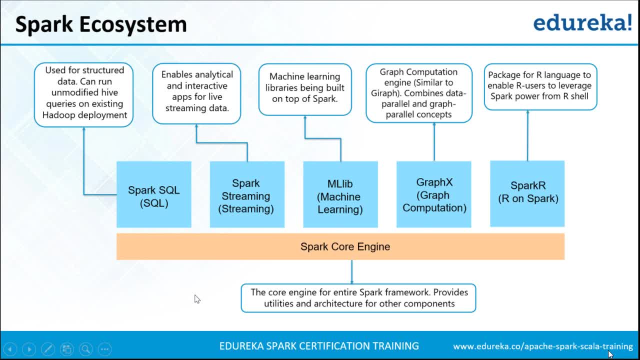 on structured or on semi-structured data. you cannot use it to do the analysis on unstructured data. so if you say that your requirement is to do the analysis on unstructured data, you will be using the course bar api only. okay, again, you will have to write the program to process the unstructured 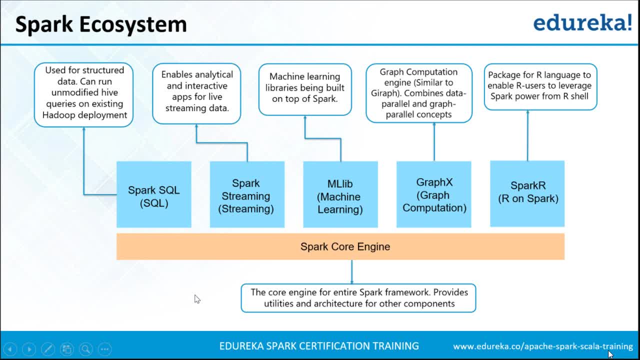 data. that is something which you cannot do using spark sql, okay. okay then what do we have? we do have spark streaming. so spark says that i do have one more module which is by the name of spark streaming, and it says that, using this module, you will- if 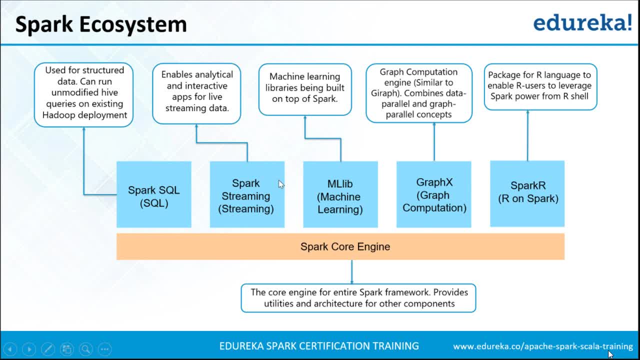 you use this module, you'll find a number of inbuilt functions which will help you in doing the analysis on the real-time data. then we do have a module which is uh, for machine learning. let's say that you are interested in implementing machine learning algorithms. then again you can use r. 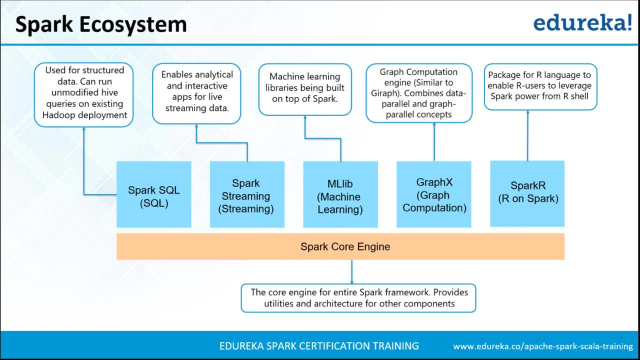 sorry, you can use spark. then if you have a graph data right as in, you do have friends and then friends of friends, if the need is to do the analysis on that kind of data, then graphics can be used. so basically, graphics is similar to neo4j. okay, neo4j is a type of no sql database. 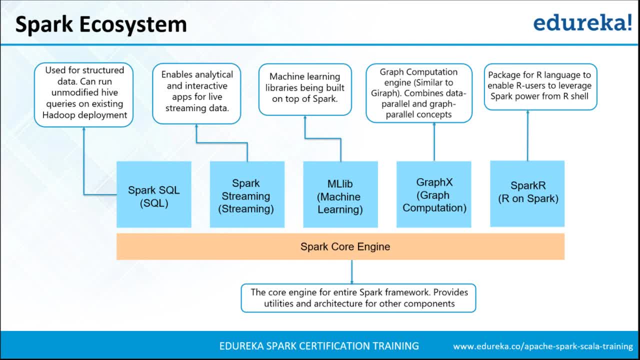 which is designed to do the analysis on graph data. and then what do we have? we do have r. so basically, r is a programming language which is designed specifically for doing the statistical analysis. so if you think that you are interested in doing the statistical analysis, then you can integrate. 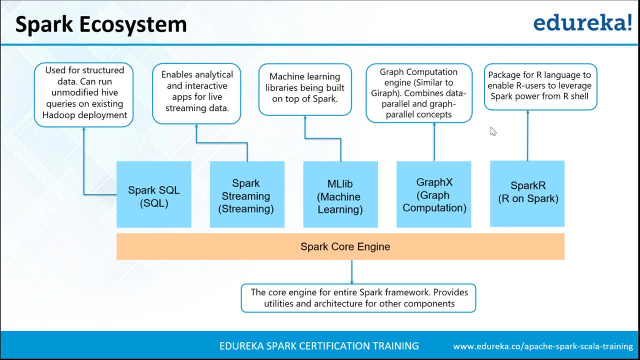 spark with r. okay, okay, our question. um, in spark, you will make table and schema for structured info data. yes, so now that's something which, uh, which we cover in detail in the code. so, as in, you will have your input data in form of a file on hdfs. the only thing is you will be taking help of the data frame. 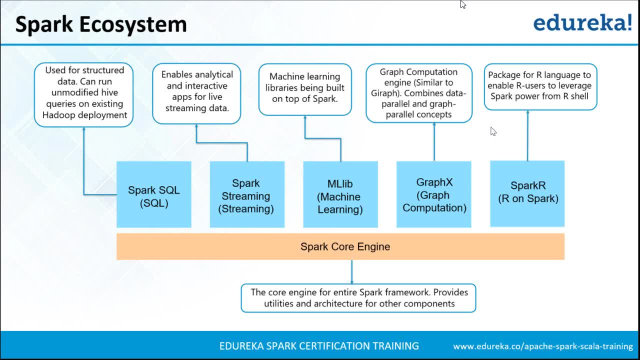 so it will. it will show you. it will show you your data in form of rows and columns and you will be thinking that internally. you will be thinking that internally, uh, there is a underlying table. okay, the only thing is it's kind of abstraction or it's a kind of grid we'll be placing on top. 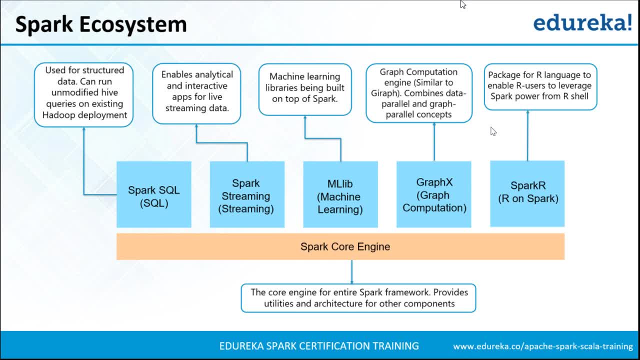 of the data, and you will be thinking that your data is in form of rows and columns. okay, so this is a product of the style design id in general. so you will be kind of going to the all the data aspects like, uh, you have hdfs and then you have right now. 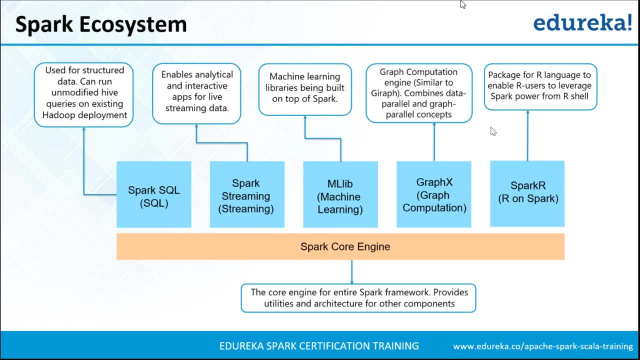 hdfs, and then you have ancients and you have, you know, the all the things that are gonna be used to do the trading. so after we run that, we will call it python for spark, okay, okay, like you have r for spark. same way, python for spark is also there, yes, and we call. 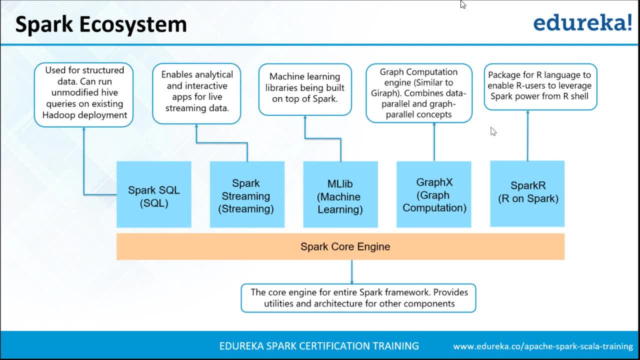 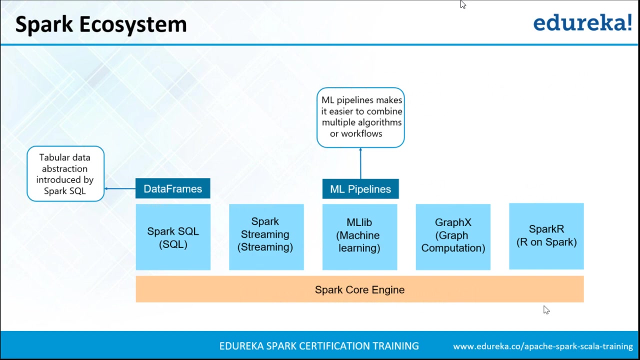 that as pi spark. so if you are uh, interest, if you are interested in implementing the, Okay, Okay, So let's move on. Okay, so now shots effects What you have. You have a file on HD affairs, or you do have a file with you, And what you are doing is you are placing a grid on top of this data. 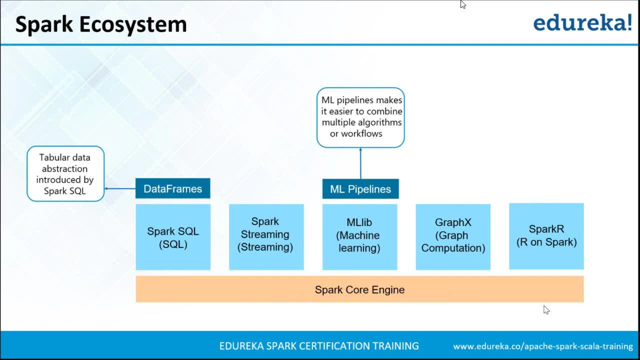 What do you have? you have a file with you and what you are doing. Guys, am I audible? Okay, perfect. So basically, up. so what you have. you have a file and what you are doing. you are placing a grid on top of this data. So the point is, if you look from top right, you will be able 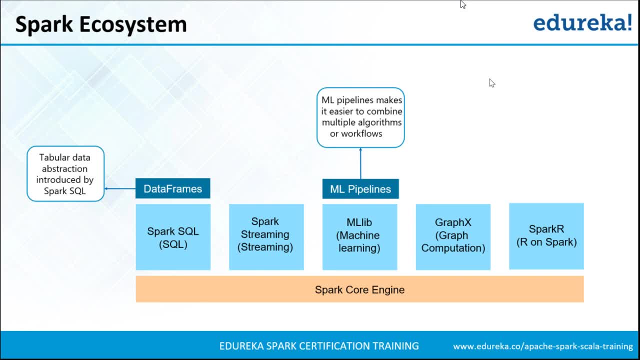 to see your data in form of rows and columns. So that's what this data frame is doing. simple thing: You have data and you place a grid on top of it and you are not changing the underlying structure. Underlying structure will still be the file. It will still be the. 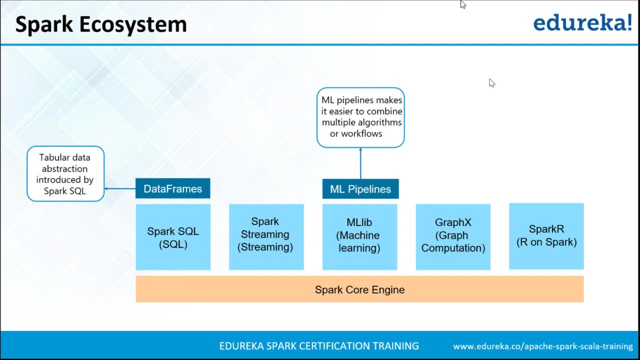 file. Okay, and yeah, this is about Spark sequel. Then what you have is, if we talk about Spark streaming right again, we say that we have n number of inbuilt functions. So those are the functions which will be seen going forward. then, when we talk about machine, 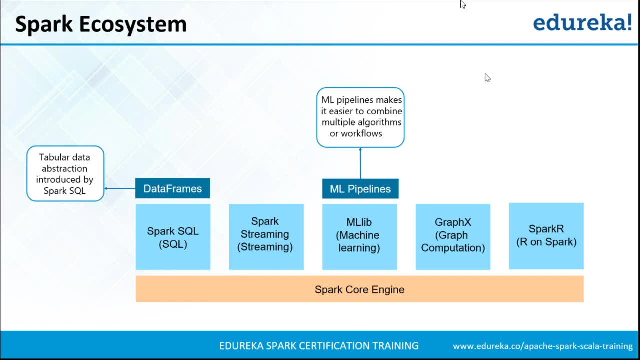 learning library, right, So here you will be creating the machine learning pipelines. So basically, you will be combining a number of things, will be creating a pipeline, and it will make your job very, very easy, Like if you are interested in implementing a machine learning algorithm. Okay, And yeah, now that's so simple, So yeah, 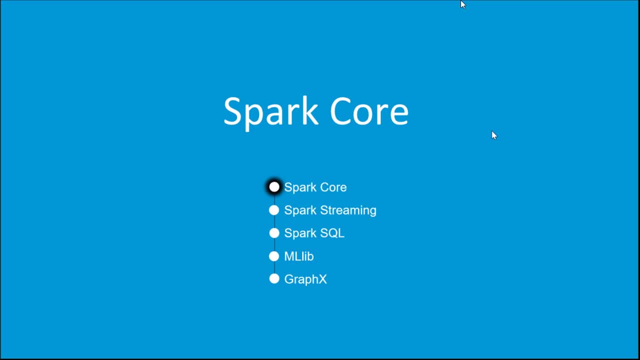 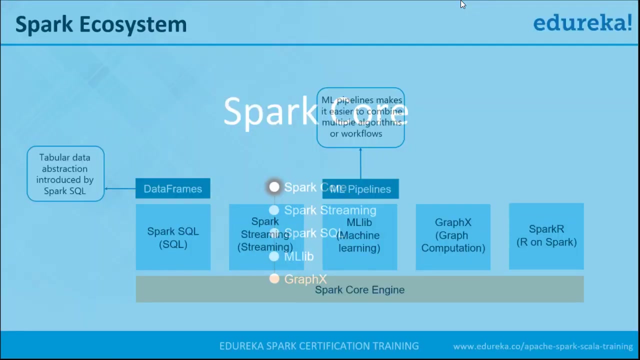 we are going to start. Okay, see what is this spark core? so basically it's nothing, but it's the, the, the core engine. okay, and what we discuss? we discuss that we have ecosystem. so what do we mean by ecosystem? as in, you know, all these modules or all these components, they are working together as a team. 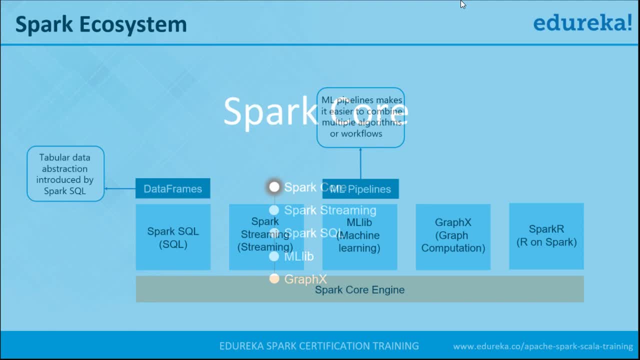 okay, they all are having different, different characteristics. they are not competing with each other. we started this ecosystem in our fifth or sixth standard in biology, right where we started this food chain and animal chain. so what is the significance of that, or what it signifies? it says that you know we all are dependent on each other. so that's why we say: 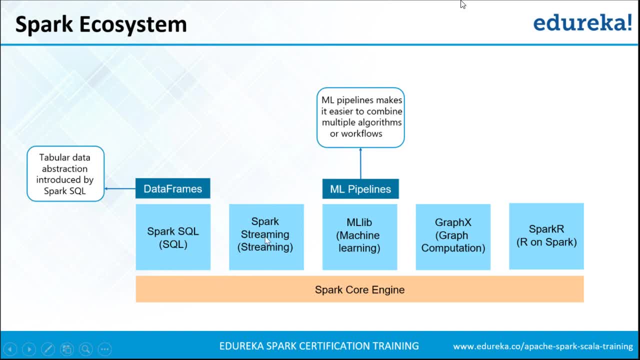 that it's an ecosystem. why? because spark sql, spark streaming, mlb graphics, spark art- they all are running on top of this and they are not competing with each other. spark sql will say that i have a different characteristics all together, but i am dependent on spark core. 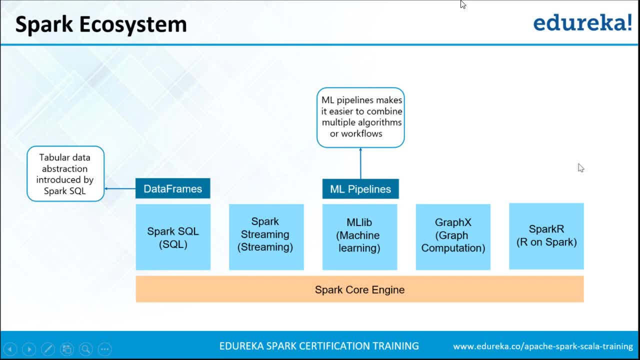 engine. so now spark core engine, right, it is capable of understanding a business logic given in, given in a programming language, given in a programming language. so whenever, whenever you talk about- let's say that you have written a sql query- what it will be doing internally, it will. 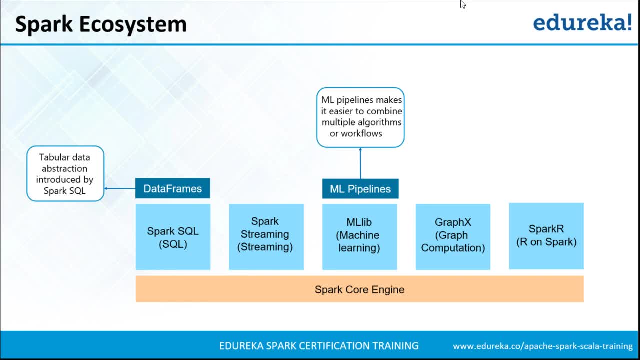 be converting your sql query so that it can be understood by the spark code engine. okay, so i have a question here, like why it's not shown? because pi spark is not something which is extra module. that comes as part of spark core engine, only it's. it's not a module, okay. 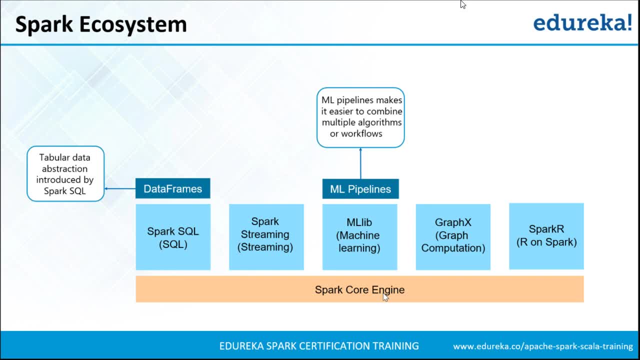 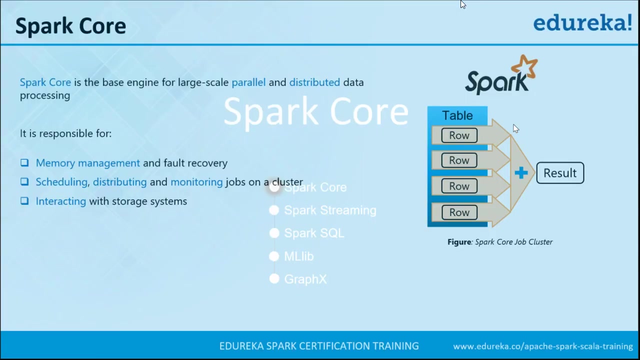 but when we talk about r, right, so there are n number of functions which will help you in doing the statistical analysis, and that's something which is not coming as part of the spark core engine. okay, so let's move on. so now, if i talk about spark core, right, so this is the engine which is? this is the engine. 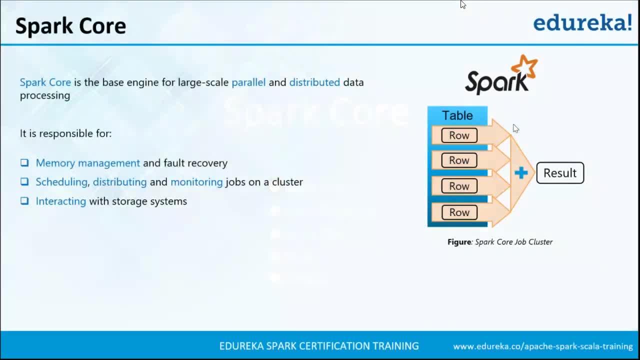 which is responsible. this is the engine which is responsible for memory management and fault recovery. so it's like now what we will have. we will have all our data in the memory. so let's say that something goes wrong. so let's say that something goes wrong, then how it'll. 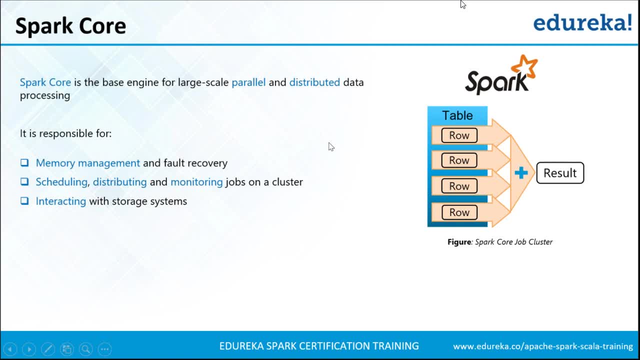 be recovered, the data and everything. so it will be handled by core engine, then scheduling, distribution of the data, monitoring all the jobs running on a cluster. again, it's a role of a spark core engine and also it will be interacting with the storage system. okay, so yeah, does. 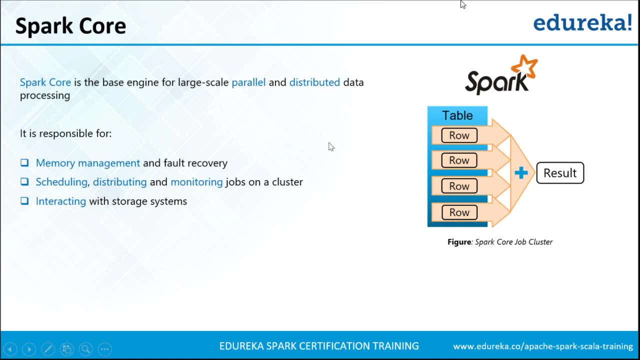 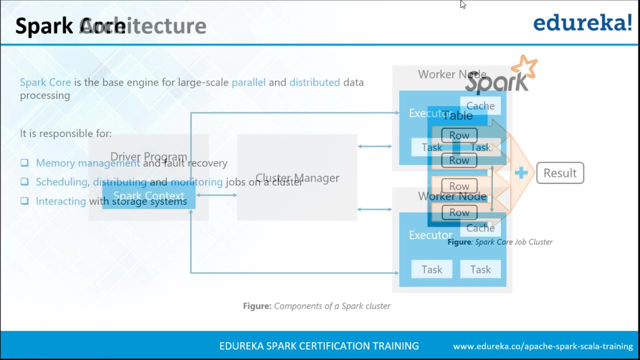 does spark support s3? yes, it does. the integration can be done with s3, with ec2, with the local local file system and also with the HDFS. so yeah, now this is the spark architecture. again, it's very easy to understand. if you've walked on hadoop already, then it's a very easy for. 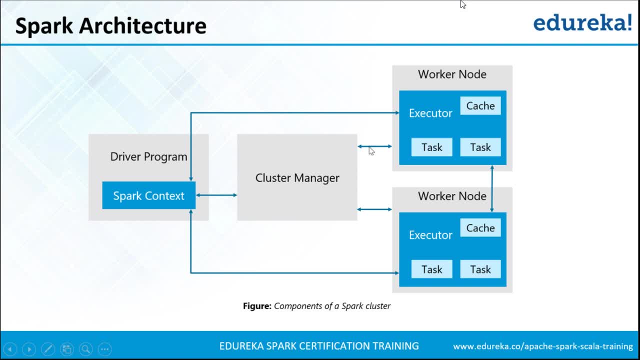 you to understand. so what do we have? it's like, let's say, that we do have a cluster of two nodes, as in two machines would be running in parallel, and in case of spark right, terminology is bit different and here we are calling them as worker node. in case of hadoop right, we 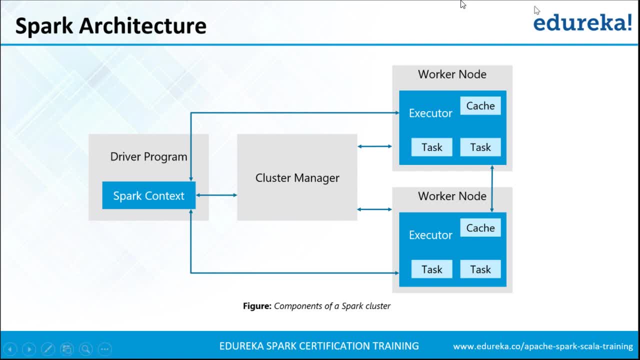 them as data nodes. so what you have got here is you do have worker nodes right and on each worker node, what do you see? you see cache right. so this is something which will be missing in case of sorry. so this is something which will be missing in case of hadoop and why it would be missing. 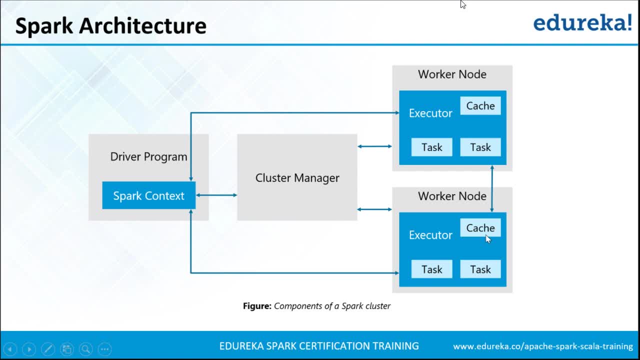 because uh hadoop, uh doesn't need, uh, basically, it doesn't do in-memory processing, right, it is not doing the in-memory processing and that's why we say that you know this cache would not be there. but now spark does the in-memory processing, so you can see that we do have cache. 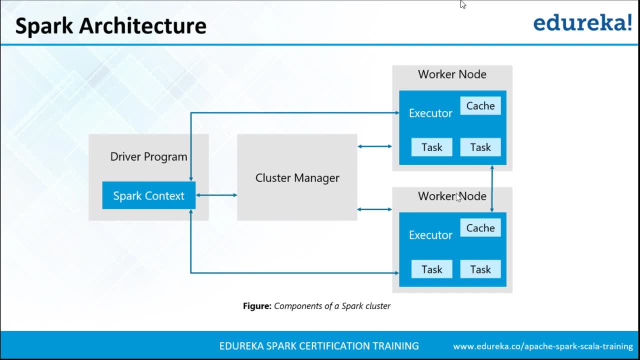 right, we do have worker node. and then what do we have? it's like we do have a driver program or it's, or we do have a spark context which is nothing but the main entry point. so you as a client, right, you will be submitting the program here or your job details here, and then it will be going and 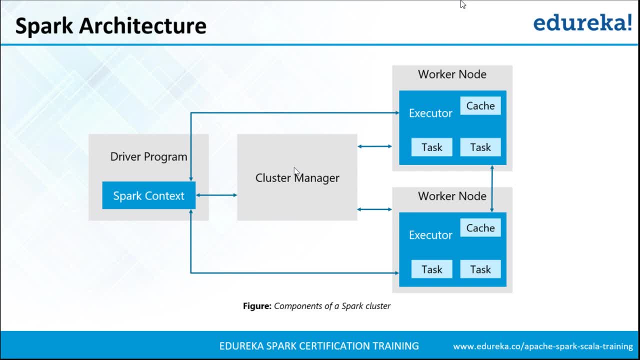 it will be interacting with you, and then it will be interacting with you, and then it will be interacting with this cluster management framework and it will say that, hey, you know I need to submit this job, Can you help me? and running this job already. 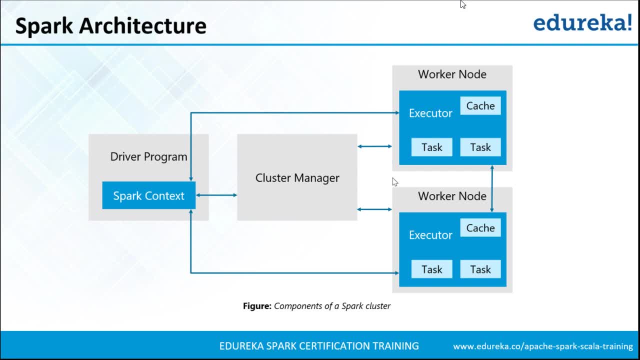 So internally, cluster manager will say that okay, your data got splitted to these many partitions and these two partitions are there on worker node, one and two right, and then on the worker node will have a executor or the container, which is nothing but compute plus. basically, it's nothing but compute, right. 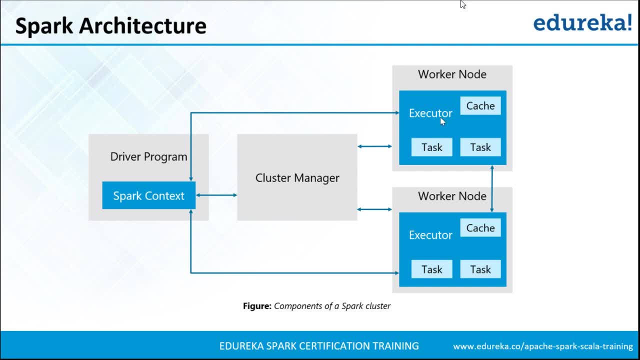 So now compute will be given wherever your data is and then the jobs would start running in the panel. So for each job there can be multiple tasks running right. So it has a similar architecture. How does it do the? no, Ravi, It is not having a fixed size like we talk about block in HDFS. 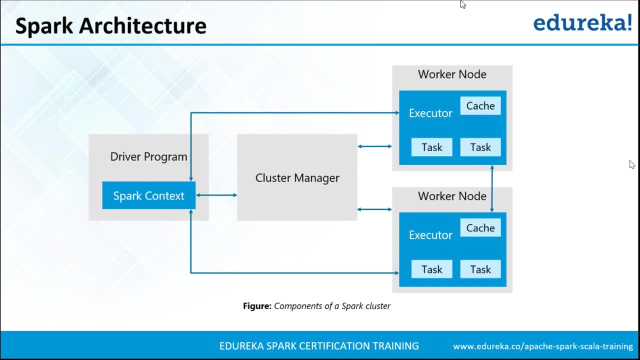 So that I the maximum size is 128 MB. So when it comes to the default partitioning and Spark right, It will be doing based on the number of codes and the number of executors. It has got a different formula altogether. It's not fixed like Hadoop or like HDFS. 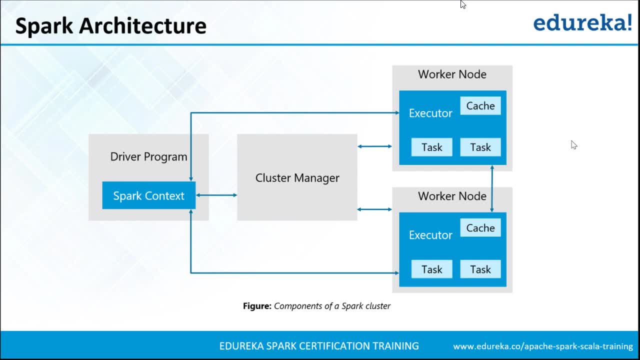 So always it will differ, no fixed size, and it will depend on the number of code and the number of executors which you have for your job. So, yeah, let's move on. No, you, you don't need to worry about that until unless you are working on the optimization. 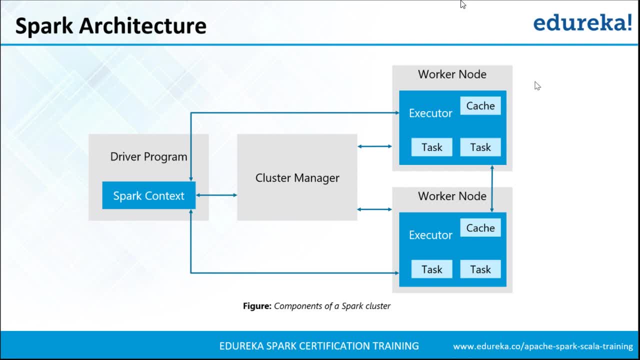 Okay, so there are ways of performance tuning or, you know, optimization, in which you will say that if you increase, Then you'll be getting much better result. In that case, you need to know that formula and you need to say, like, how many number of partition should get created? 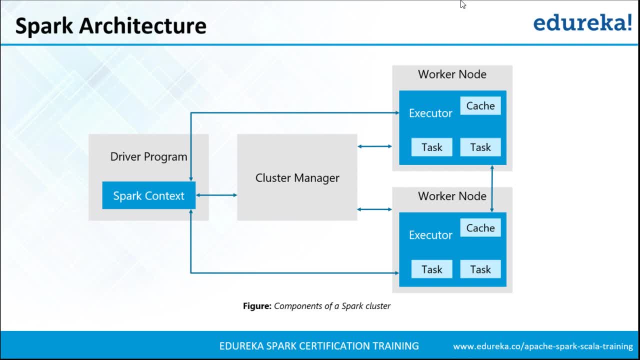 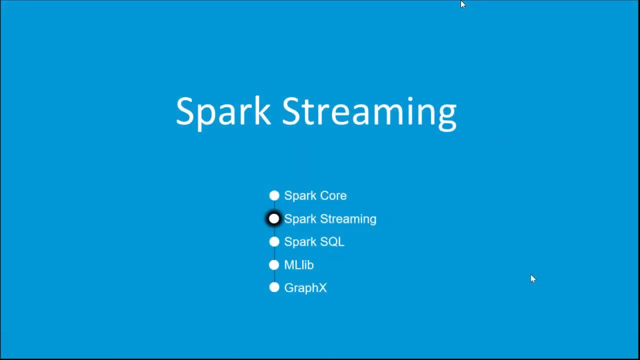 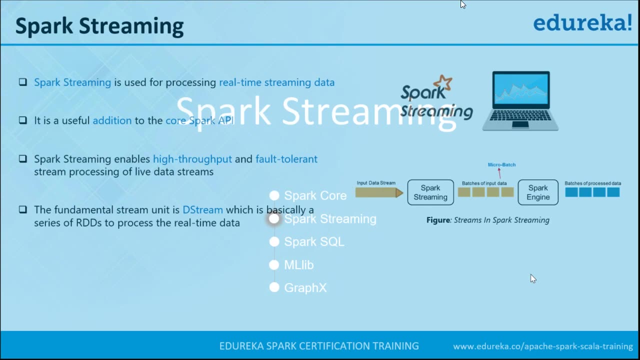 Okay, So let's move on. Okay now, spark streaming. So, again, this is the module which is being used to handle the real-time data. So what is the use of this? So just pay attention to this. So what? what we are feeding to spark stream. 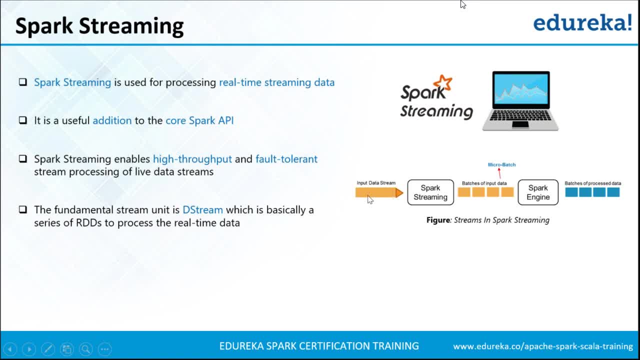 We are feeding a input data stream which is continuous. what you see here, You see a continuous data stream, as in, the data is flowing Continuously. right then, here, What you will have to do is we will have to what we are doing. 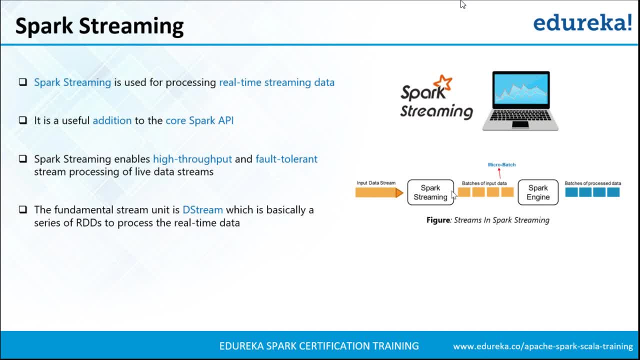 We are feeding the continuous stream to the spark streaming and what it is giving as an output? It is converting this input stream, or input data stream, to the batches of input data as an now, this is nothing but the sequence of RDDs. So what, what? what we had fed to spark streaming, basically, 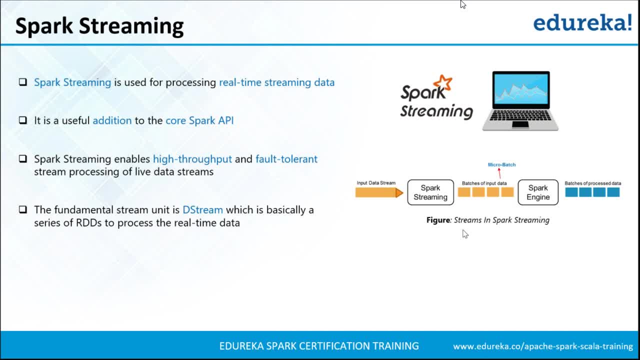 we were feeding input stream and what we are getting as an output of. as an output of it, We are getting the RDD of RDD of different, different sequences. guys, Give me a second Okay. so yeah, what do we have? we do have batches of input data. 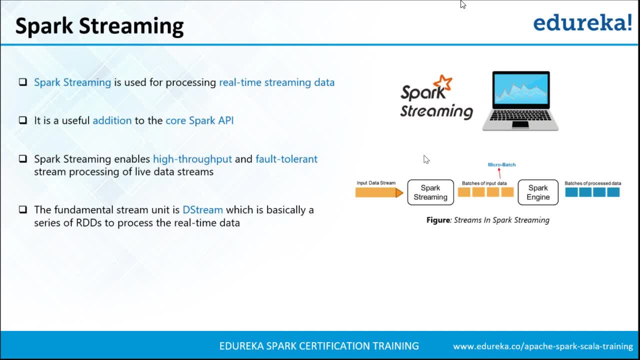 So this is nothing but the RDD. it is nothing but the sequence of RDD getting created at a specified interval. So basically, you will be telling this thing to the spark stream: that whatever continuous data you are getting, split it with the interval of every second. So now you'll be getting the data at every second. 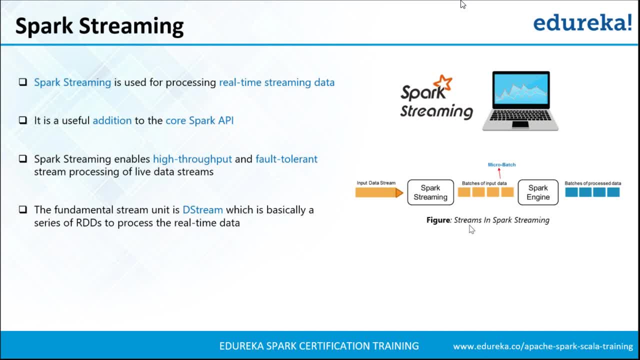 or you can specify the interval to 2 seconds or 5 seconds, like that. Okay, And then here, what you have is you have a spark engine, right, and this is the same spark engine, and it's like, once you go into the details of this, park engine. 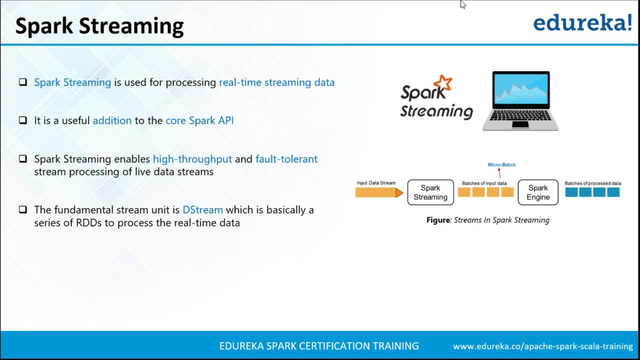 right, you will understand that. how do you work with the RDDs? and here, what spark streaming is assuming? spark streaming is assuming that you already know how to deal with the RDD, So what? that's why what it is doing. it is saying that I'm making your job easy. 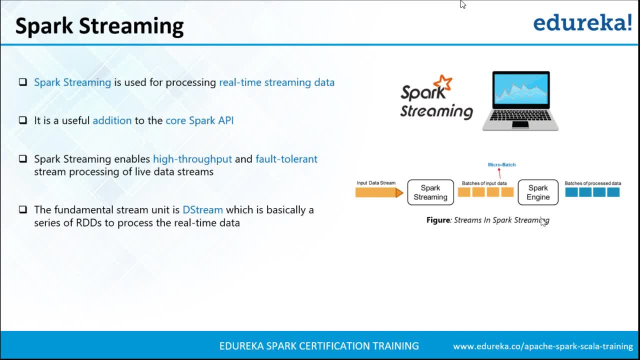 It says that you already have expertise on working with RDD. So now what I'm doing? I'm getting this continuous input stream and I am creating sequence of RDDs right. So now, if you know how this course park engine works easily, you will be able to work on spark streaming. 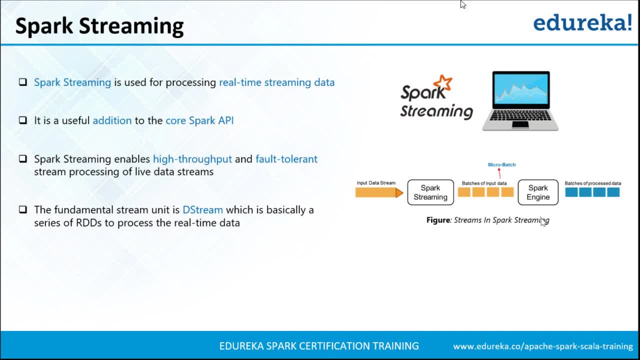 Is it mandatory to stop start Hadoop to run spark application? No, we are just talking about HDFS, not about map reduce. Okay, and also, what makes park faster than map reduce? spark design memory processing Hadoop, It doesn't do that. 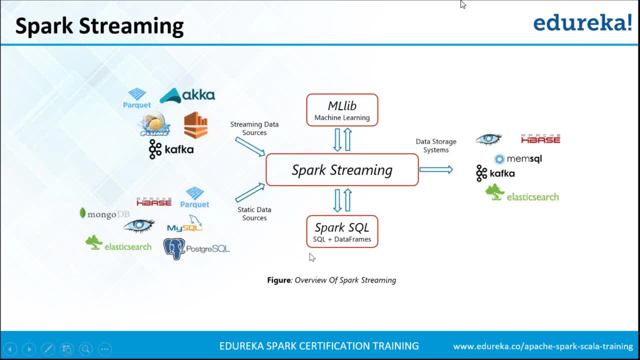 So yeah, now when it comes to the application of spark streaming. so what do we have? we do have various streaming data sources, as in. we do have Kafka park- a flume, So it's like we will be getting the streaming data. So as in, let's say, Uber, right, Uber in actually is using Kafka, spark streaming and MLF. 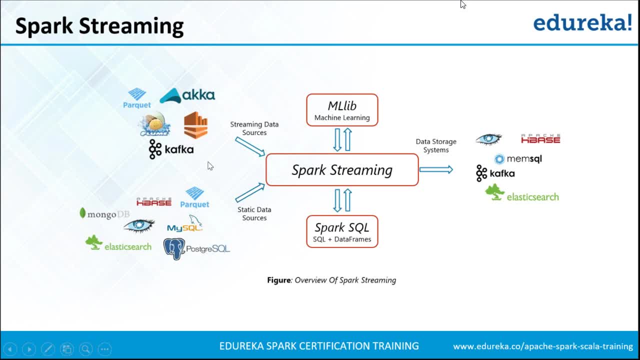 So, whatever data, Kafka is collecting the date. So Uber is collecting the data using Kafka. The data is being fed to spark streaming, The data is being fed to spark streaming for processing, and then on top of that data, Uber is running the machine learning algorithm. 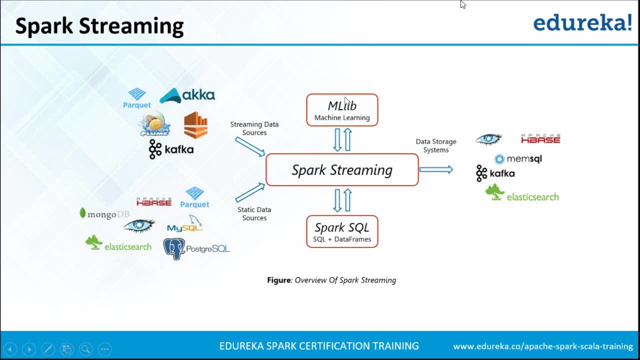 to understand that. what are the areas with high demand or with low demand, and accordingly, they are having this search price right. So, yeah, and spark is capable of getting the data from static data sources as well. even that is possible, And once you get this data right, you can write. 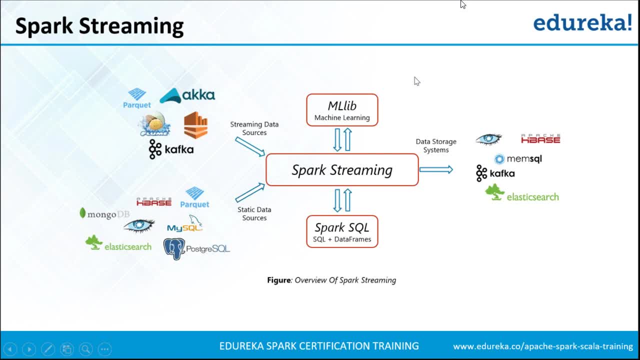 I guess sequel like queries to do the analysis. and yeah, once you have the output, you can store it anywhere based on your requirement. You can store it to edge base, You can, so Kafka or elastic search, Okay, So yeah, this is about spark streaming. 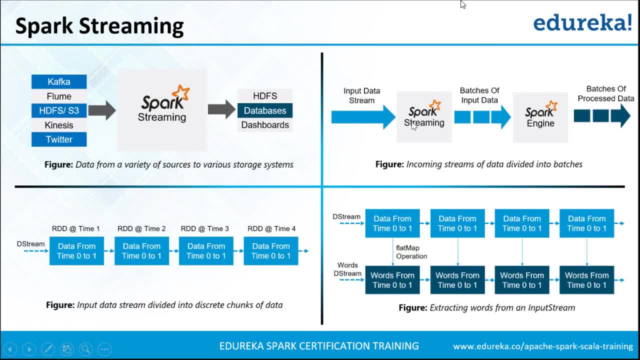 So now, if we go into the details, the same thing. okay. So what I told you? I told you that integration will be done with the streaming sources. here We are doing the integration. then what this park streaming it is doing? it is splitting this stream into sequence of RDD. 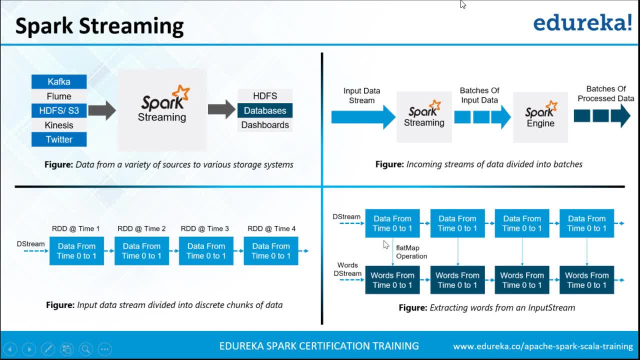 So now, now you see, this is sequence of RDD. So this is RDD a time one. This is already a time to time, three time for, and whatever logic we had to tonight that is getting applied on each and every RDD. So what is up now? if you have worked on code spark, okay. 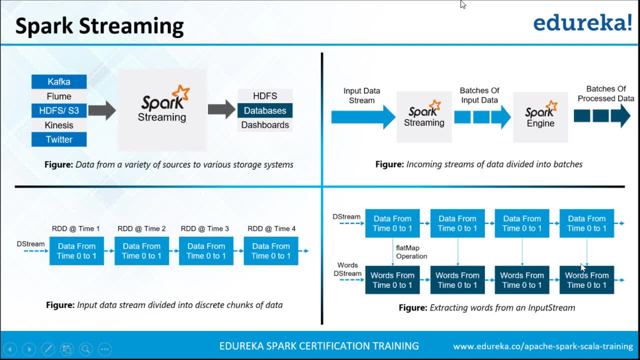 and now, after that, if you start working on spark streaming- hardly there- there are four extra lines which you need to write. that's it Okay. So if you know how to work on the RDD or how to deal with the code spark engine, 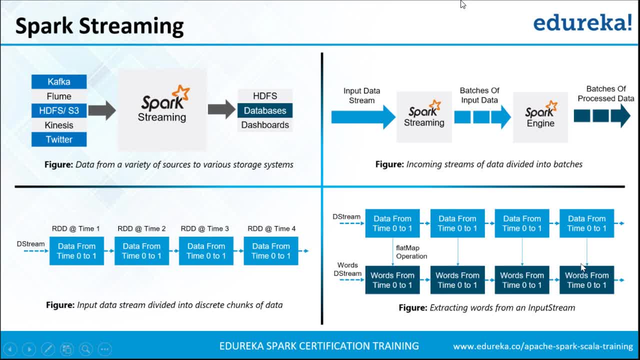 then it's very, very easy for you to deal with the real-time data, Okay, Okay, So the point is here. everywhere It is showing time 0 to 1 because we have given the interval as one second. Okay, but if you look at the complete picture, 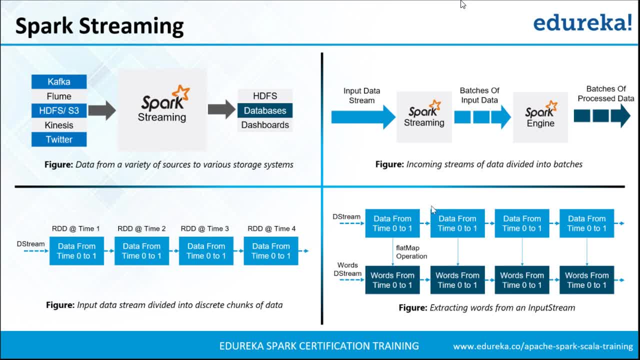 right, so it will be a time one, time to time three, but the interval is a one second day, So as in 0 to 1, it should be like 1 to 2 to 2 to 3, 3 to 4,. 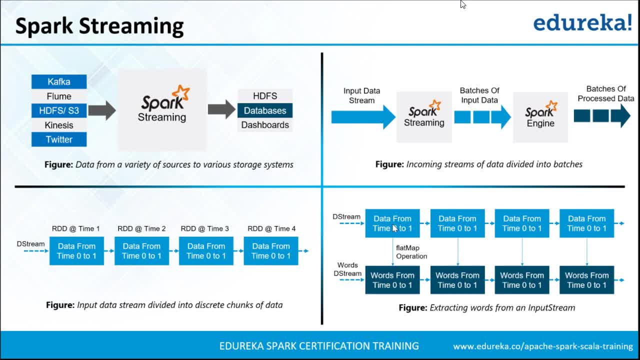 but because the interval is a one second, so they have written it. but yeah, they can, they can make it more readable. where they can say time 0 to 1, then they can say time 1 to 2, 2 to 3, 3 to 4, like that. 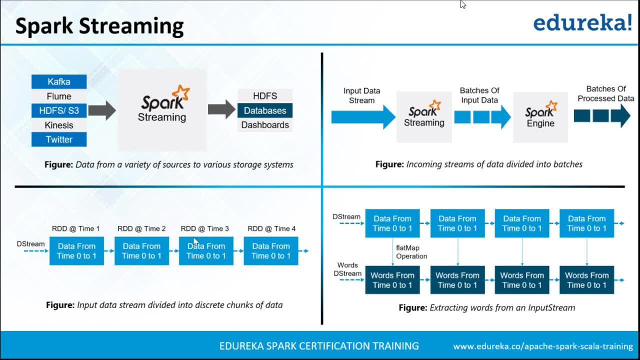 This is what you see here: RDD a time one, RDD a time to RDD Time three and then RDD a time for. Okay, So let's move on. What is the minimum time I can specify? you can give the intervals of microseconds as well. 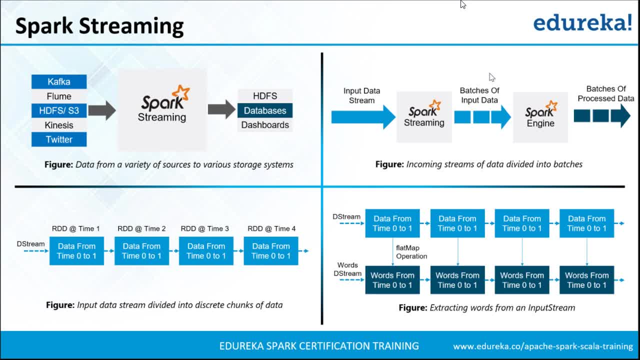 So not sure, like how many of you have heard about storm. right again, storm is the ecosystem component which is designed to, which is designed to do the analysis on real-time data. Okay, Again, it's a ecosystem component which is designed to do the analysis on real-time data. 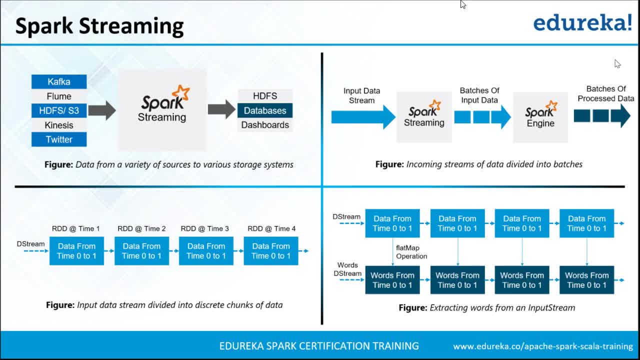 So what is the difference between storm and spark like? in case of spark, right, every time you need to specify this batch interval. That's a different story that you know. this batch interval can be of milliseconds or microseconds, But, yeah, you need to specify the batch interval. 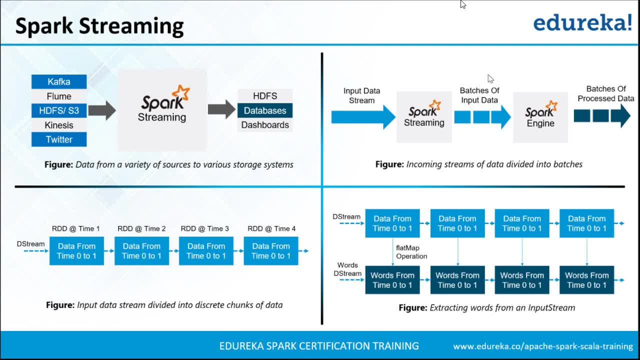 But when it comes to storm, right, you don't need to Do that, and that's why you'll hear people saying that storm is faster than spark, because here again, you are talking about intervals, You are splitting your continuous stream into the sequence of RDDs and then you are doing the analysis. 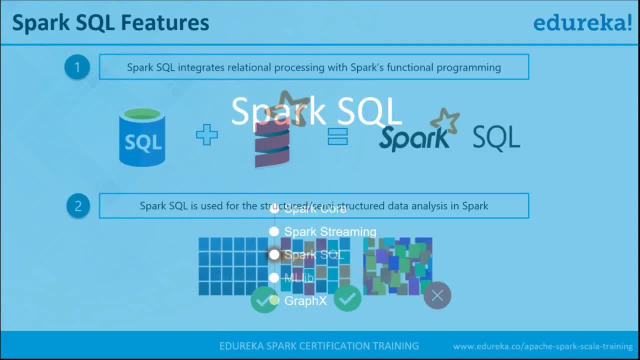 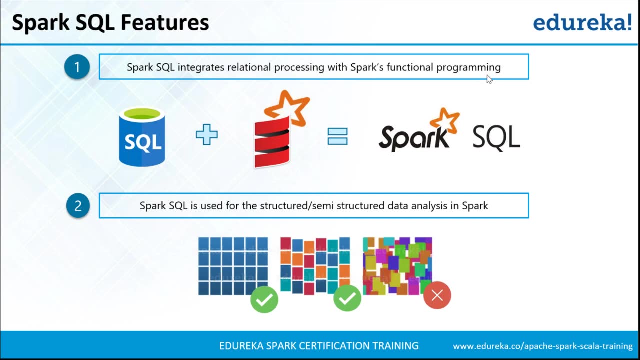 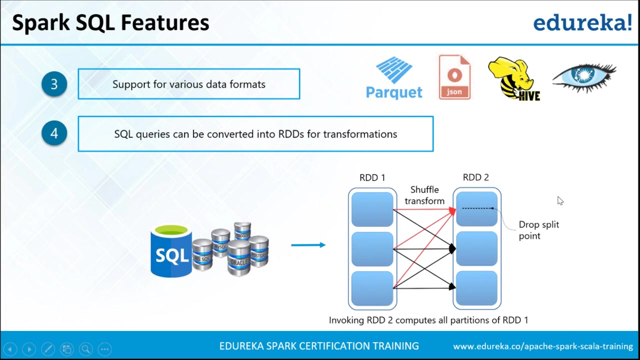 Okay, So now, when it comes to spark sequel, again, you will be using spark sequel to do the analysis on the structured as well as on the semi structure data. Okay, So here spark sequel right, it support various data formats. It supports various data formats. 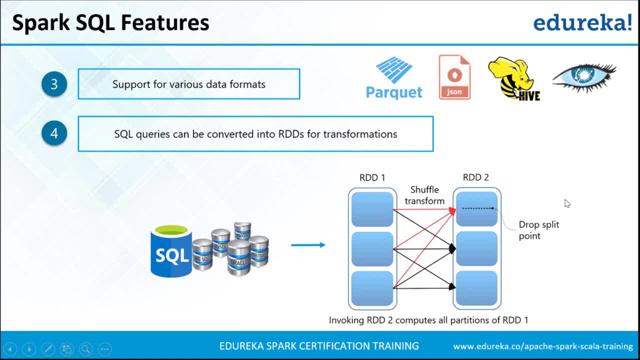 It will say that, yes, you know, it can read the data from hive, It can read the data from park and also it can read the data from Cassandra. Okay, and also whatever queries you are writing right internally, These queries are getting converted into RDD. 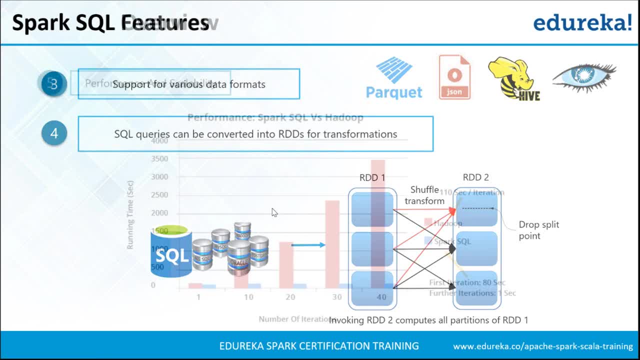 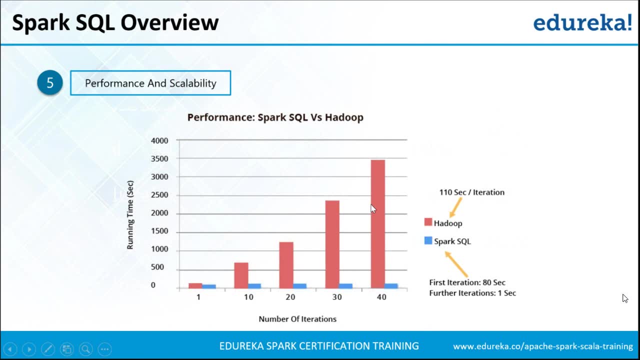 Because that's the code. So now if we look at the performance and the scalability, right. so you see, like every time spark is taking writing the user-defined functions. So those functions you can write using any language. So basically you can do. is you do that using Scala python? 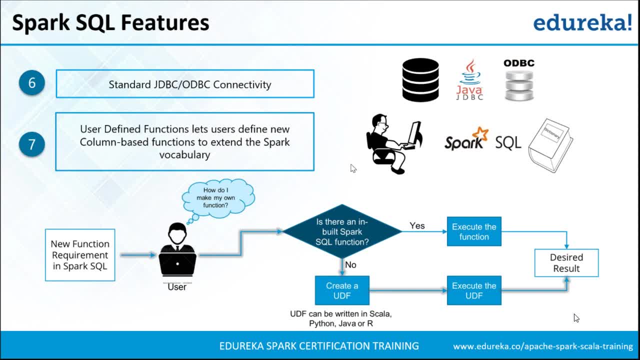 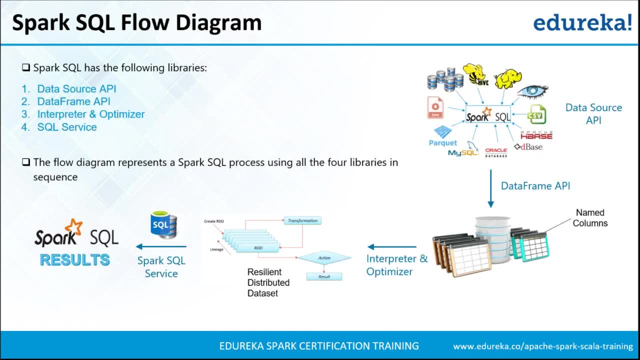 R or Java. Okay, so this is what happens internally. So, first of all, what you will be doing. So, when you start working on spark sequel, right, first of all, you will be Reading the data from a source, right, and this source can be of any type. 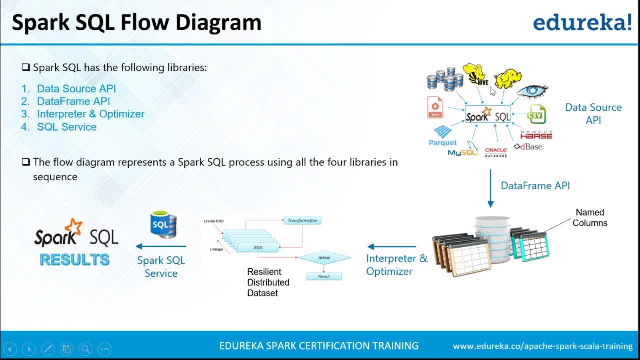 So you see different, different type of sources here. So basically, you see Hadoop, you see how you, you see spark C H, base right Oracle. So for reading the data from a source right, you will be using the data source Right, so reading the data. 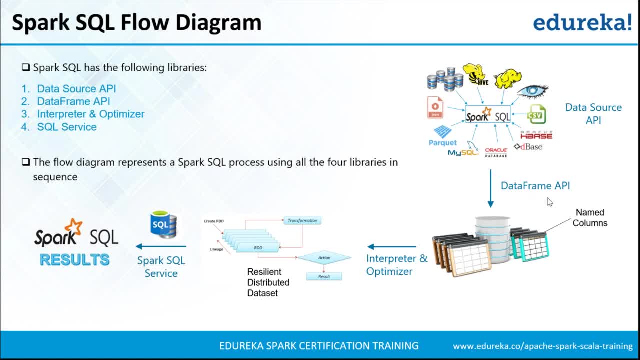 right, you will be using a data source API. Then, once you have read the data, so you will be using the data frame API. I told you right. basically, data frame is nothing, but it's a grid which you will be placing on top your top of your data. 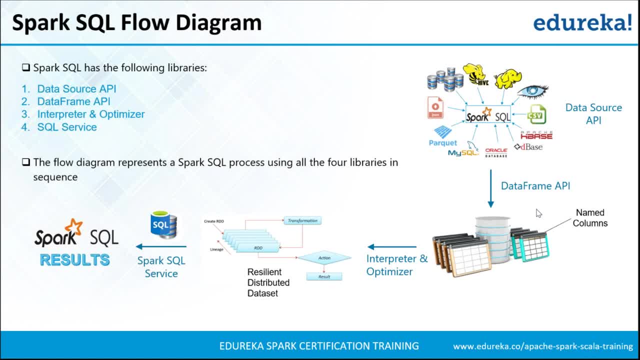 so that you are able to see your data in form of rows and columns. I so what? what it will be doing? It will be placing that grid on top of your data so that you will you see your data in form of rows and columns and you can write the sequel like queries. 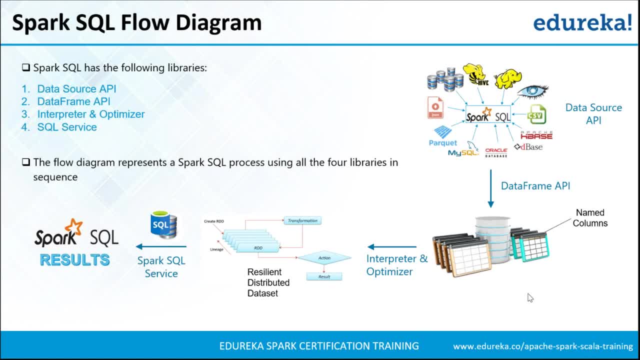 So then, what it will be doing: whatever sequel query you have written, right, It will be generating a corresponding plan for that. So similar, like even high, works on that right. So if you are writing a sequel, like query, so what I will be doing, 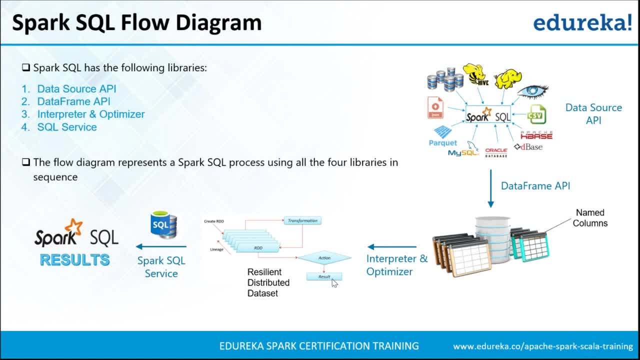 I will be generating a plan and that plan will get. I will be generating a plan and that that plan will get submitted to MapReduce for the execution right. So here for the sequel query right. What do we have code? We do have core as an RDD. 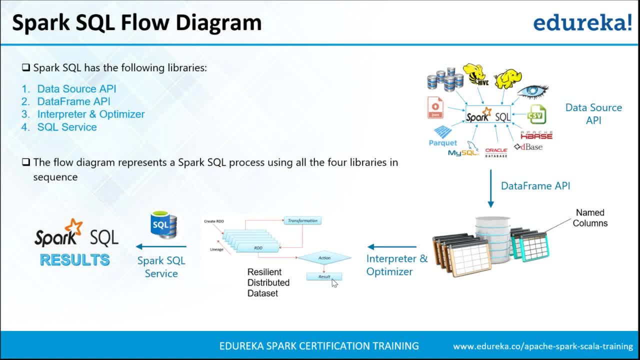 So what it will be doing, it will be, you know, interpreting and optimizing your sequel query so that it can be submitted to RDD for the execution, or it can be submitted to the course park engine for the execution. And finally, what do we have? 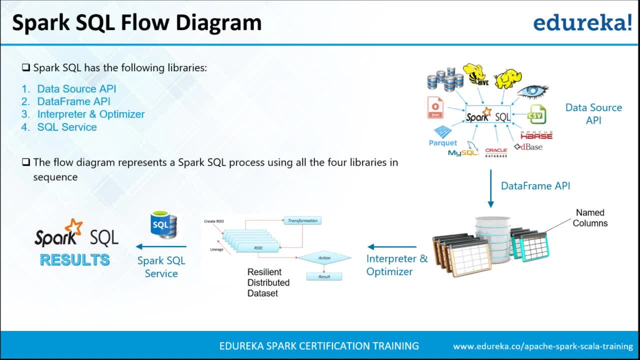 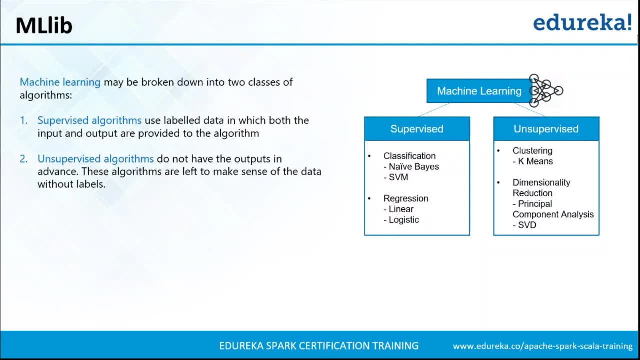 We do have a sequel service API, using which we will be getting the output. Okay, and then? what do we have? We do have MLA, But before that, I see a couple of questions. Okay, the process. if you lower the speed, how do we know what CPU these are? 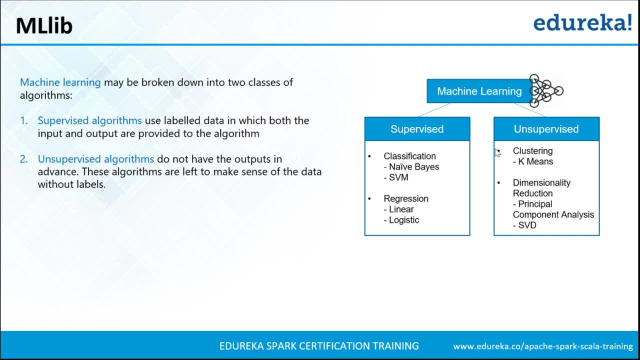 This is what we call as tuning. You will do all the parameters, you will observe the performance and then you will. it's about, you know, experiment. So you will be tuning the parameters and you will be observing the performance. Then our question: each RDD is executed by separate machine in cluster. 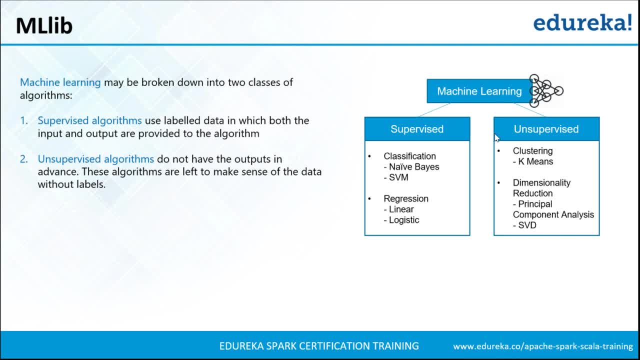 So RDD is nothing but a partition, right? So your partitions will be there in the different different machines and all the machines would be running in parallel. Okay, Yeah, So now when we talk about MLF. okay, so when it comes to spark. 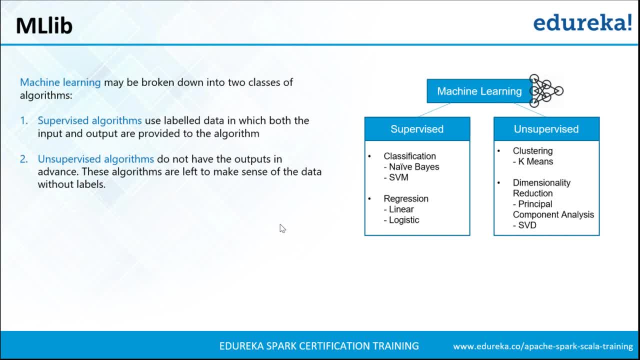 so we do have a, we do have this module. So which would say: is that okay? so we do have a module which says: which says that I do have n number of functions which will help in implementing the machine learning algorithm. So here, what do we have? 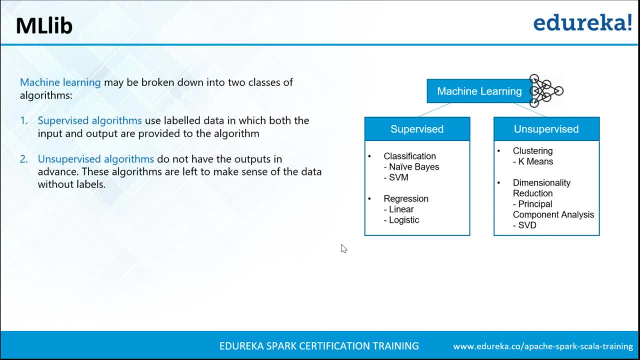 We do have. what do we have? We do have a supervised learning and then we do have unsupervised learning. So, for supervised learning, when it comes to classification, a phase, then support vector model and for regression, linear logistic, these algorithms you can implement. and then, when it comes to unsupervised learning, 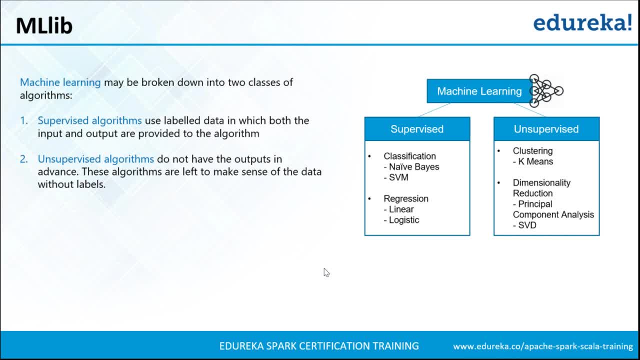 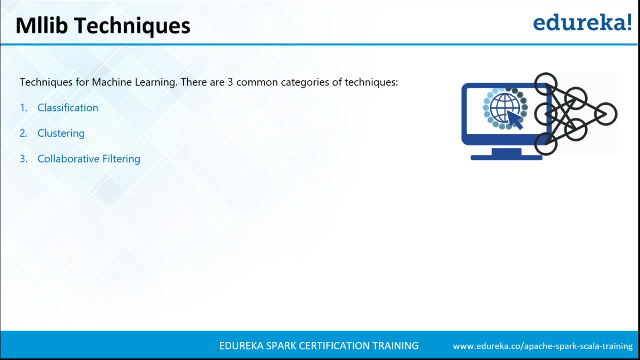 you can implement the key means, clustering. then also you can use dimensionality reduction, right principle, component analysis and these things. Okay, Yeah, then when it comes to machine learning techniques, diet, we do have classification. So what is this classification where we say that to tell me if this is a spam. 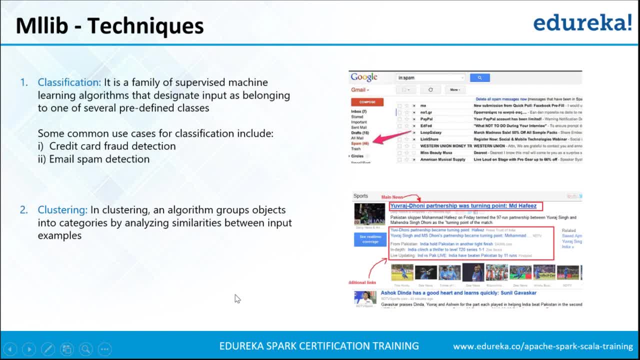 or this is a valid email, So that's nothing but the example of classification. Then what do we have? clustering as in now. I am saying that create clusters or create groups based on the user preference. I'm saying like, create cluster or create groups based on user preference. 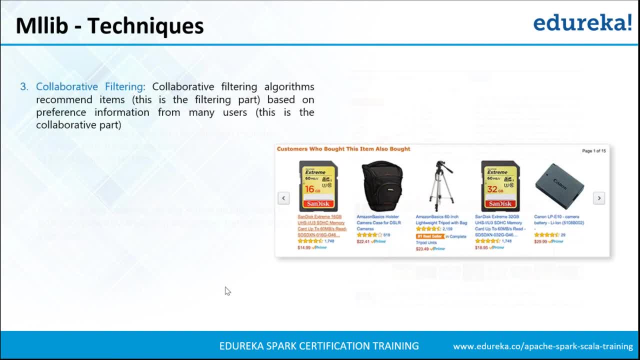 Okay, Then what do we have? We do have this collaborative filtering algorithm, as in whenever you go to these e-commerce portal, right, and let's say that you are interested in buying something, So always, always, you will get this recommendation right that the people who bought this also brought this. 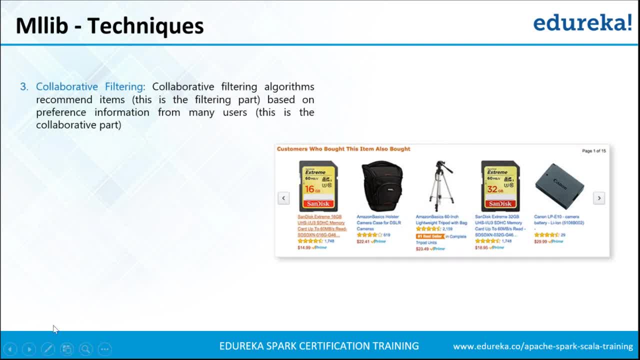 So how are they doing that? So they do have this machine learning algorithm running internally, which is nothing but collaborative filtering, which is nothing but collaborative filtering. So now this algorithm will be comparing the choices of all the users and it will say that you know. 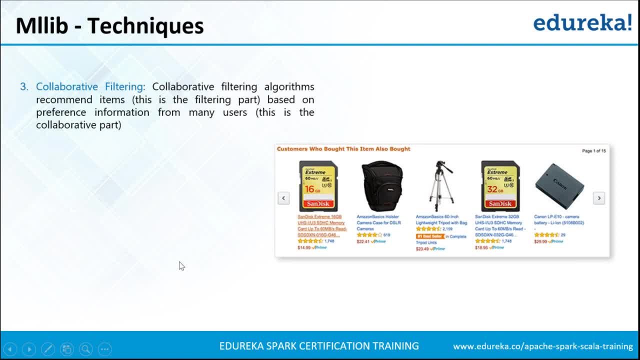 it will say that choice of these, these users, is matching and based on that, we can give the recommendation Okay. And finally, what do we have? We do have graphics, So it's the module using which you, we can do the analysis on the graph data. 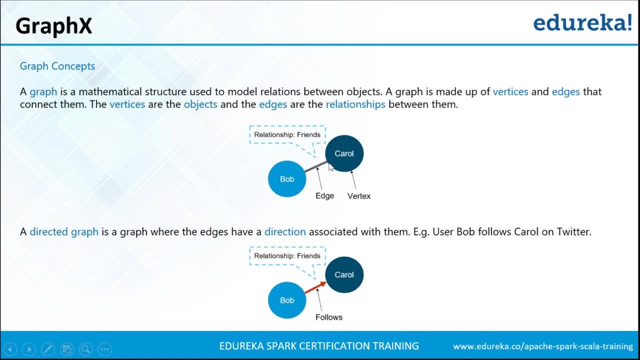 So let's say that this is the concept of a graph graph. So when we talk about Facebook, right on Facebook, what do we have? We do have friends and friends of friends, right? So you, the tree like structure, will be there. It, or graph, will get a directed graph. 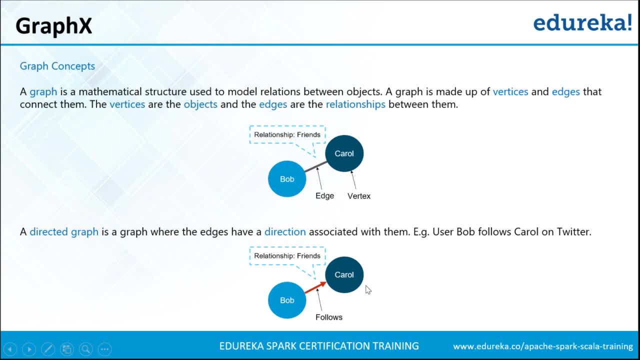 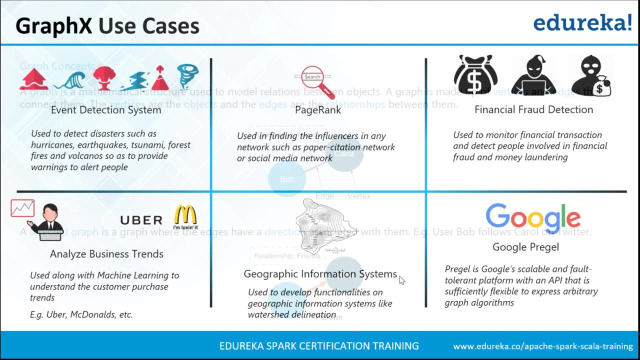 right. So we'll have a directed graph. So if you are interested in understanding the relationship, or if we are doing the analysis on this kind of data, then we can use graphics Right. So we do have graphics from spark. Then we do have Neo4j again. 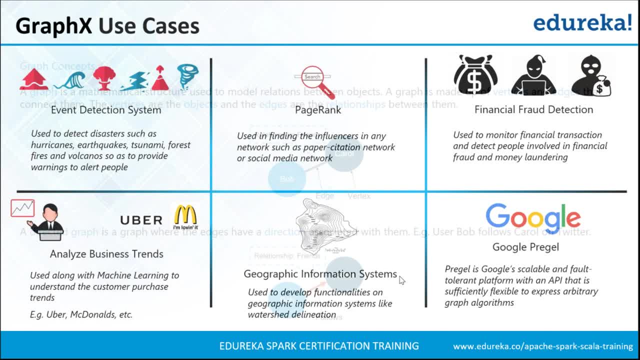 which can be used for doing the analysis on graph data. Okay, And when it comes to graphics use cases, it's being used in the event detection system: page ranking, financial fraud detection. Then we do have a uber and McDonald's. They are using it for analyzing the business trend. 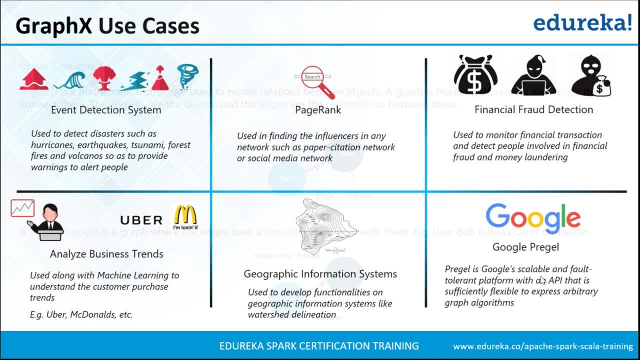 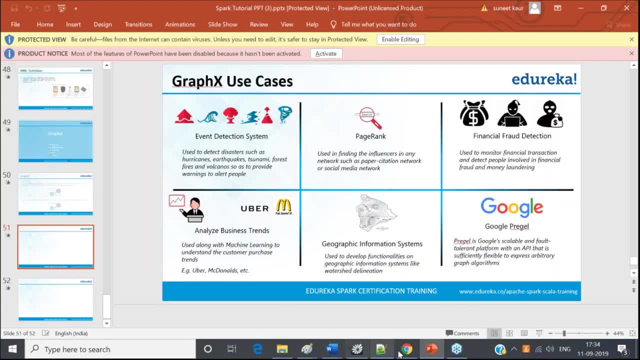 Then, as your graphic information system, Google, preggle, they all are using graphics. Okay, So now let me keep me show you How would you be doing the hands-on. So, guys, when it comes to edureka, so they have set up a multi-node cluster. 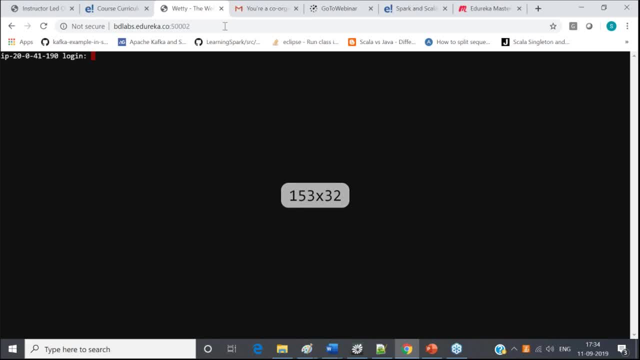 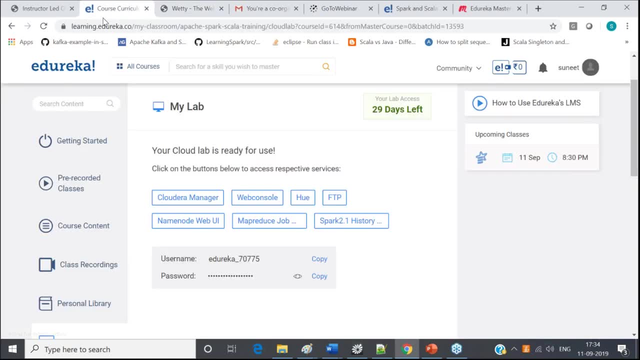 Okay, so you don't need to worry about your laptop configuration, So you just need a good internet connection in order to do the hands-on. So, guys, when it comes to edureka, so if you enroll to any of the course, you will be given the access to the learning management system. 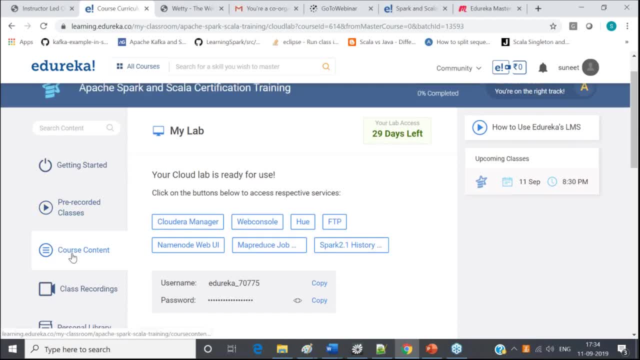 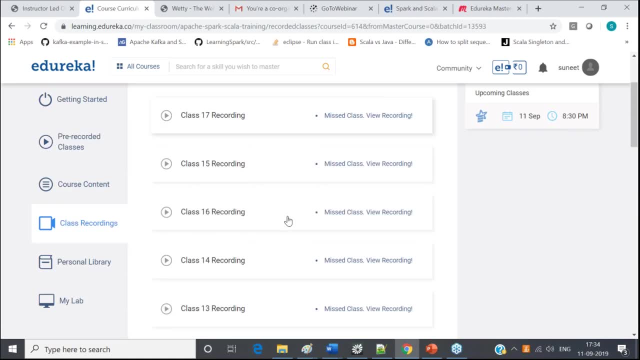 and on this learning management system you will find the course content Like, you will find all the study material presentations, You will have the recordings of the live sessions and also you will get the access to the lab right. So edureka has set up a multi-node cluster. 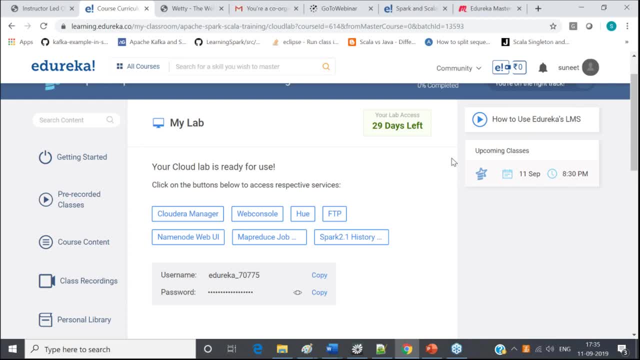 and it is set up in the same way, like your production cluster would be set up. So if you start, if you start working on this lab right, you'll get the idea how things works in the production. So now, what do we have? you will get the access. 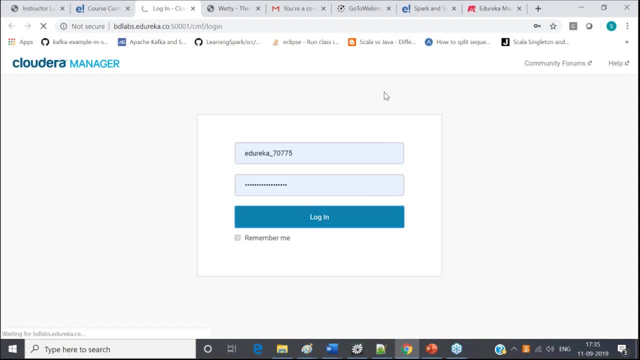 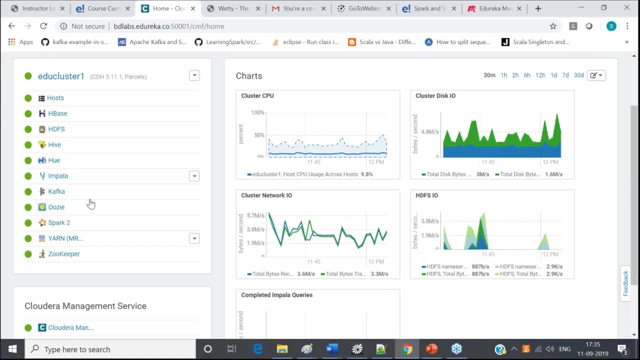 when it comes to the cloud era manager, right? So it's a basically UI which will tell you what all things are Running in your cluster. So these are the services which are running for edureka cluster. So HBase, HDFS, Hive, Kafka, Spark and zookeeper. 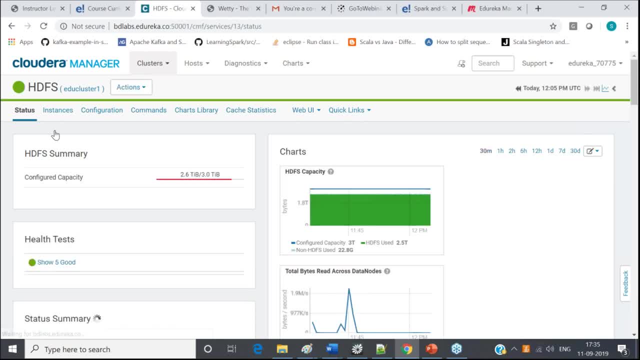 So if you go to the HDFS, you'll see that how many actual machines are running in parallel. So as in if you have installed spark or Hadoop on your system right, it will be running in the standalone mode or in pseudo distributed mode. 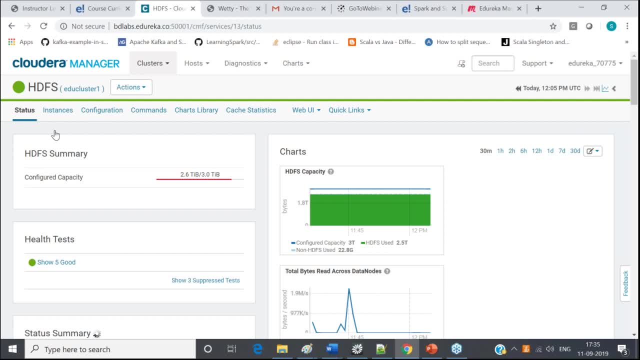 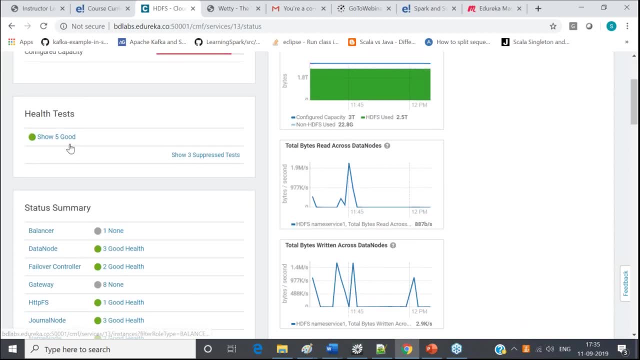 but you cannot execute the program in the fully distributed mode because for that you need actual three machines or more more than one machine. So I did. says that you know we do have five machines, not not this data node. We do have three data nodes and two name nodes. 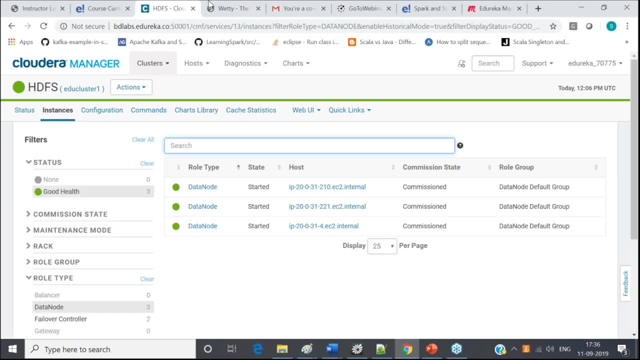 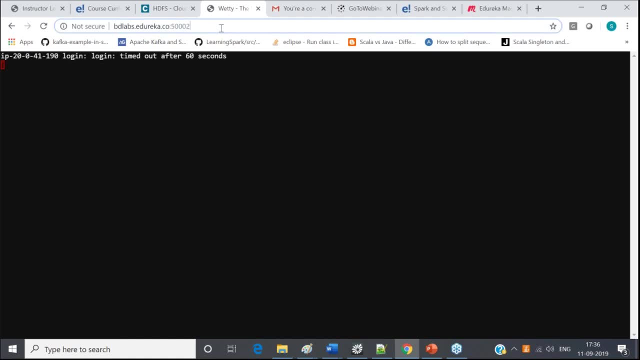 and you will see the different, different IP address and all are up. Okay, and then when it comes to as a developer, right, you will be interacting with the edge node. So this is what the edge node is. So let's say that you are interested in implementing a. 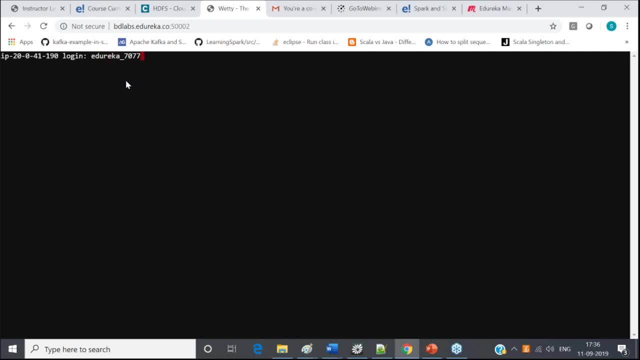 or you are interested in writing a spark code. Let's say this This: okay, So what we have got is we have got this park code, So we do have this edge node. So now, if we are interested in working on spark, right, so we do have an interactive shell. 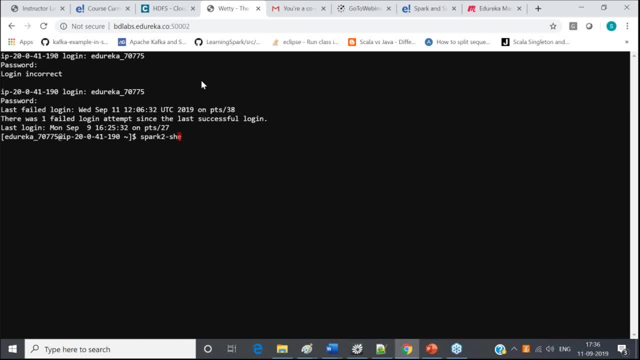 So, as in, you can execute the code here line by line, and if you'll get to know if you're going in the right direction or not, once you get the confirmation that, yes, whatever you are doing is perfect, Then you will be using this IDE. 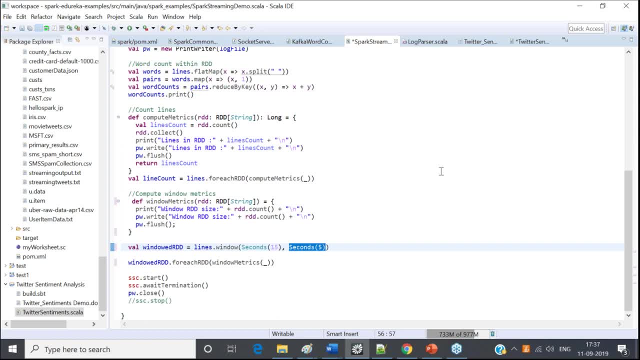 Right, So when it, when it comes to the deployment, so what you will be doing, when it comes to the deployment, So what you will be doing, you will be create. what you will be doing, You will be creating a jar file and then you will be deploying it. 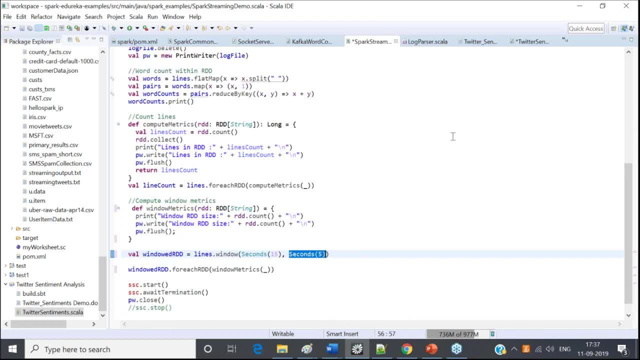 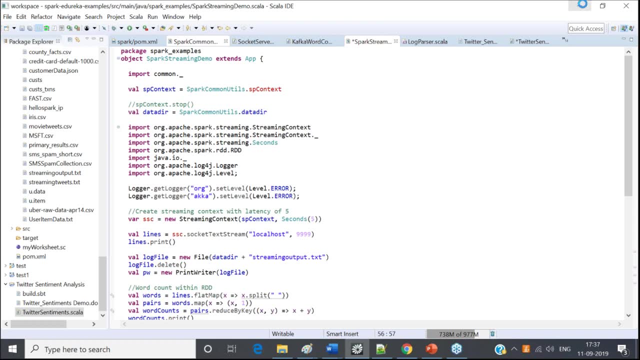 So what? that you will need this ID, right? So here you see what we have written. We have a couple of programs, Right? So yeah, So now let's go here, Right? So here, by default: spark, right, it takes you to Scala. 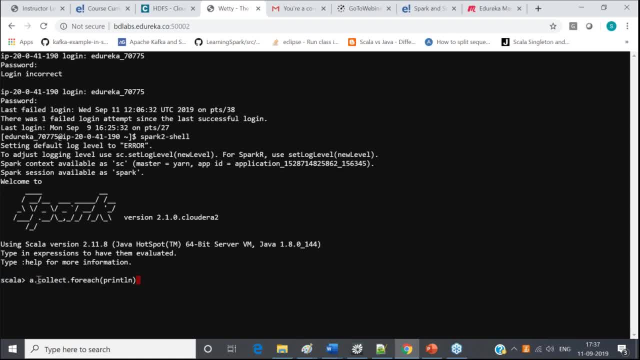 So it says that you can implement a business logic using Scala. So now let's say that here I am reading the text file which is present on HDFS. So this is the path of HDFS and this is the API which will be converting this file into an RDD. 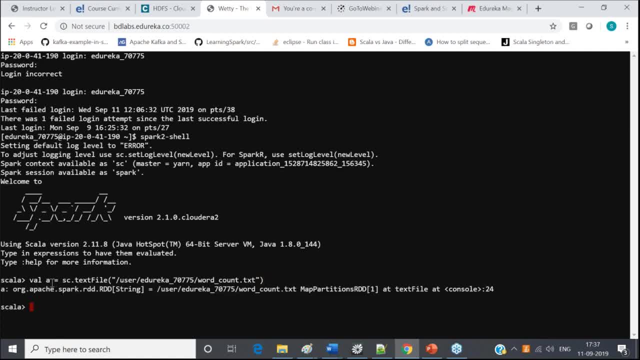 right. So here it says. it says that now I have now this Type RDD and it is of type string. So you see, it is not giving me the result, right, So it's, it's just taking the instructions. That's why I said that it does a lazy evaluation. 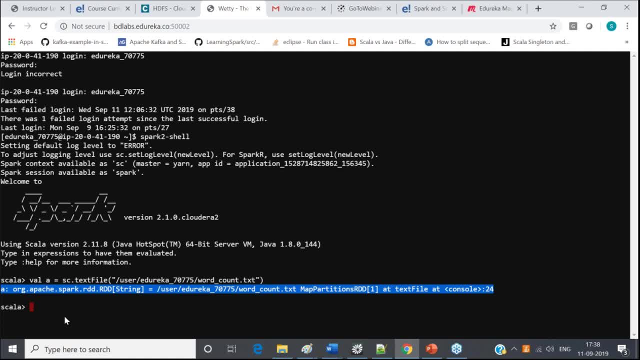 right. So now, if you want to see, like, what is there? So what you need to do is you need to collect it first, because it's running on the different, different machine, and then you're saying, for each, printed, So we'll see what is the content of this. 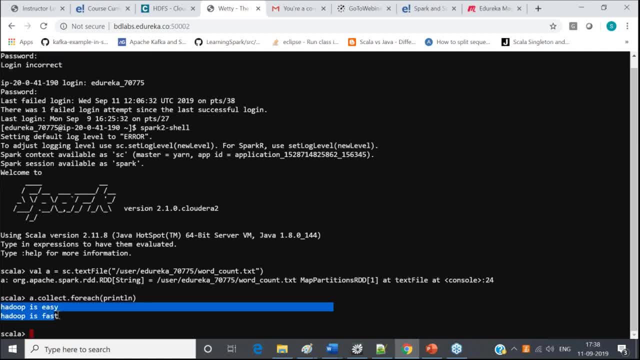 Okay, it says: Hadoop is easy, Hadoop is fast, Right, So you are working on an RDD. So now let's say that you know you are interested. You are not interested in writing this code in Scala and you are interested in working on PySpark. 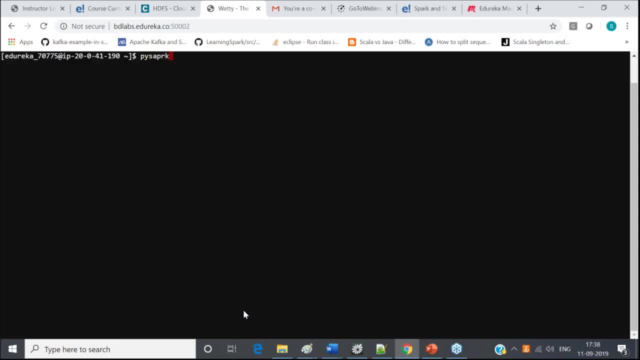 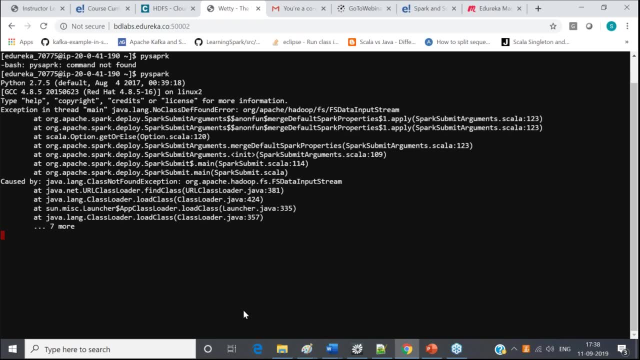 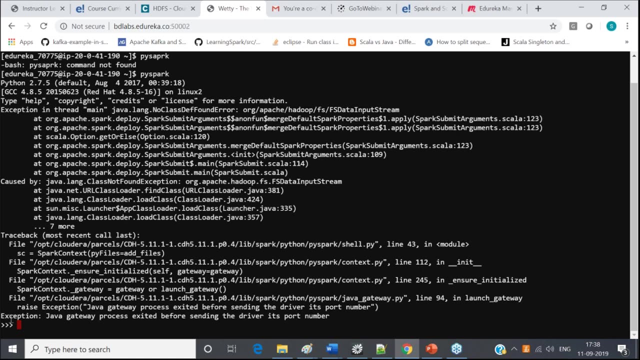 So how do you launch that? So, basically, you will be saying PySpark and what it will be doing? it will be launching the spark shell in python mode. Yeah, so there is some Issue. So yeah, now you are there on the python. 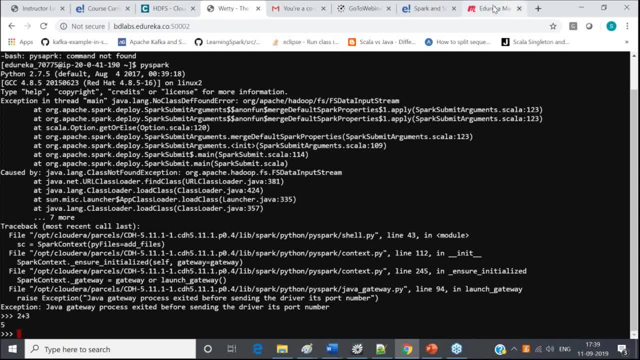 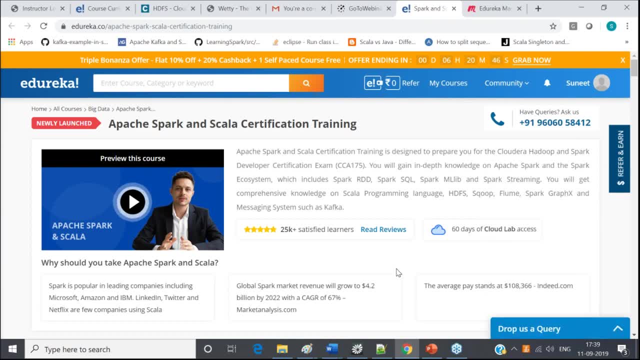 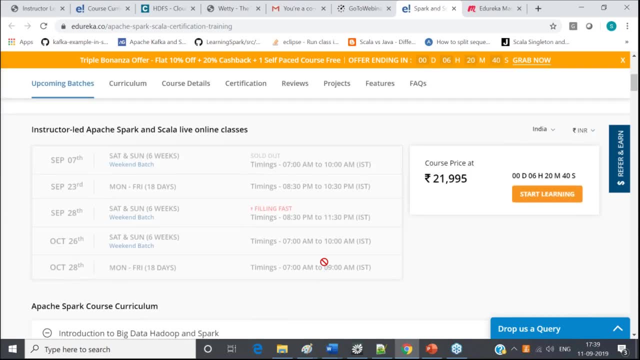 Right, Okay, so, yeah. so now let me quickly walk you through the course which we have from Edureka on Apache, spark and Scala certification training. So yes, guys, you don't see any batches available as of now, So you can keep on checking this page if you are interested. 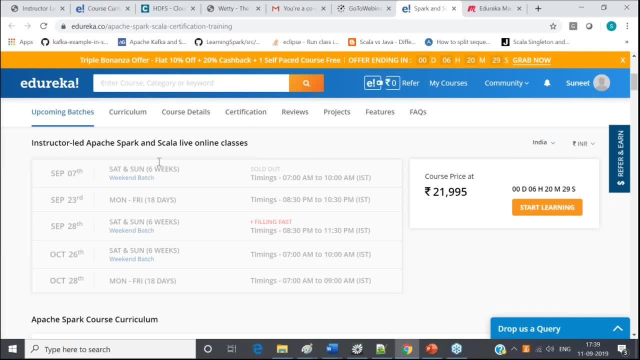 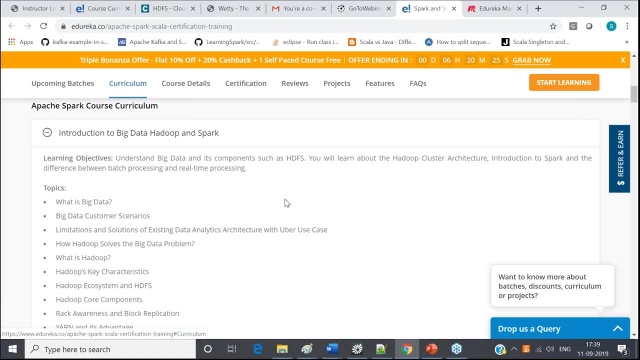 in enrolling, or you can talk to the Edureka support team and let me just discuss the curriculum. So we'll discuss, like what all topics we cover as part of this course. So the complete course will be covered in 12 modules. So in first module 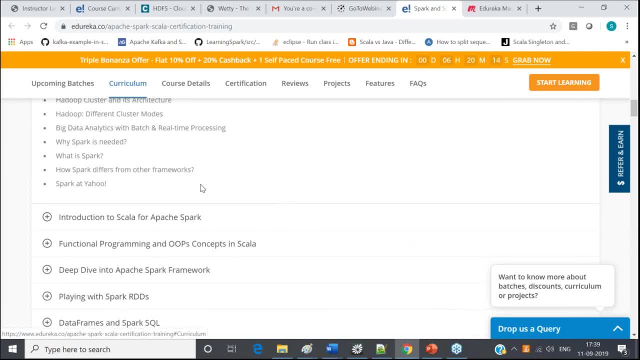 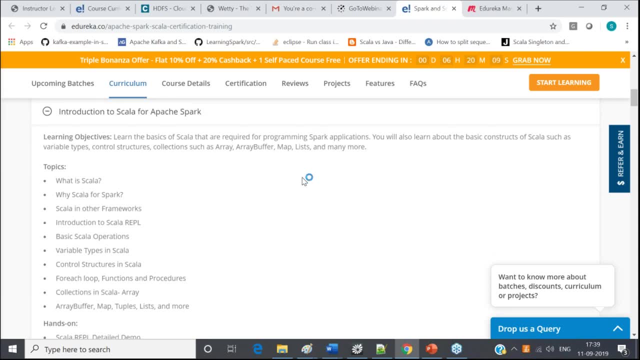 we'll be talking about big Hadoop and spark, right? Then you will be getting expertise on Scala as a programming language, right? Because the base code for spark is written in Scala. So, as part of this module, you will understand what is Scala. 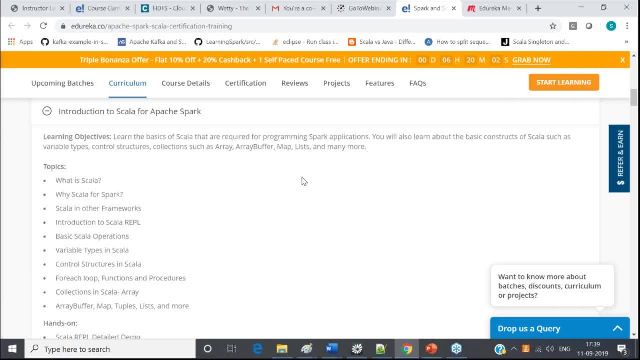 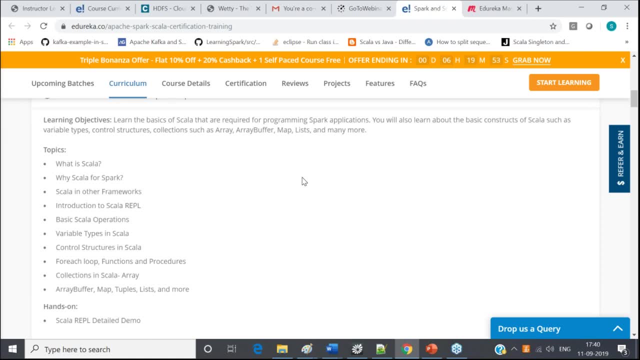 As a programming language. How do you work on it? What is basically the oops concept or how do you define a variable, and all those things. So this module will be dedicated to basic Scala concepts and then you will be understanding all the oops concept. 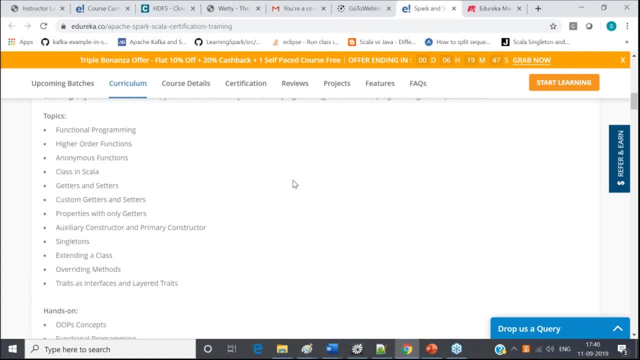 with respect to scale as, and you will understand How do you implement inheritance, Then how do you create classes, objects, then other things related, like getter setters right. as part of this module, oops concept and the function programming concepts would be covered in detail. 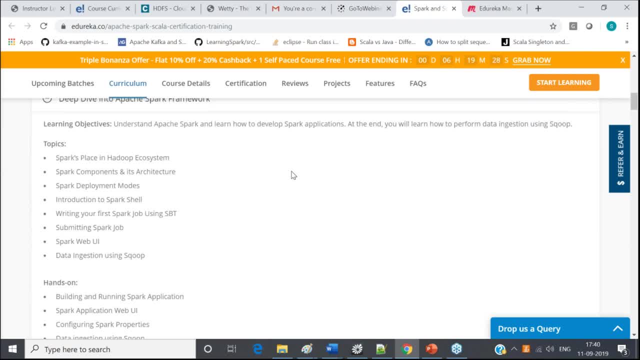 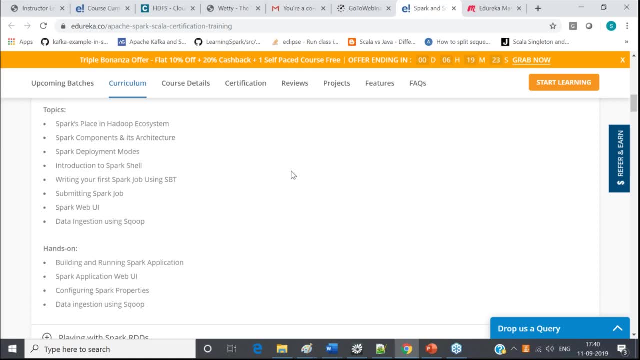 and then you will get. then you will be getting the detail understanding on Apache spark framework. You will be writing the applications. You will be using spark shell, You will be writing the applications using SBT or you will be using this IDE. and also you will understand that how do you ingest the data using scoop. 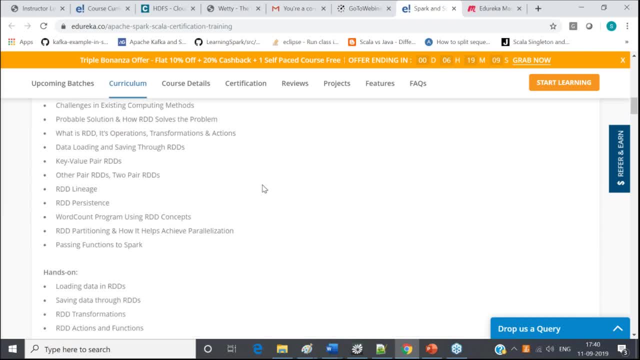 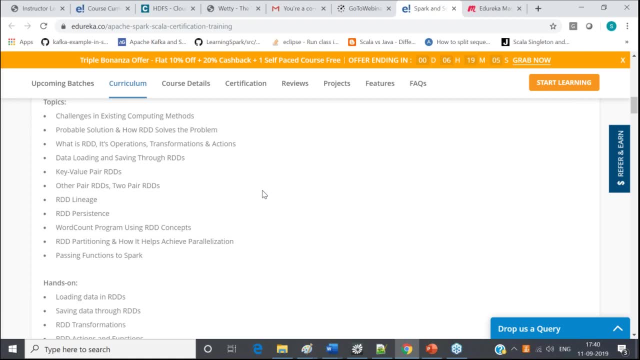 and then you will start working on RDD. So you will understand that How do you implement? the business logic on RDD is: how do you, How do you try, How do you do the transformation, or how do you do the transformation, or how do you do basically, 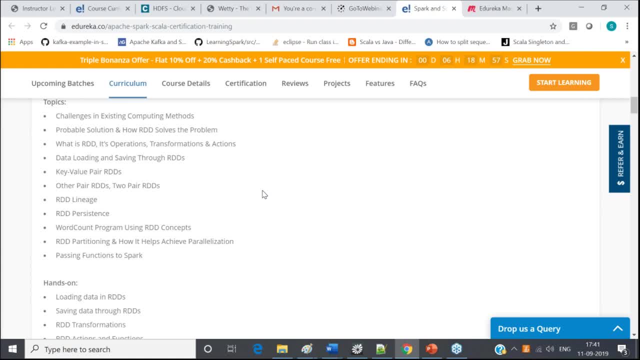 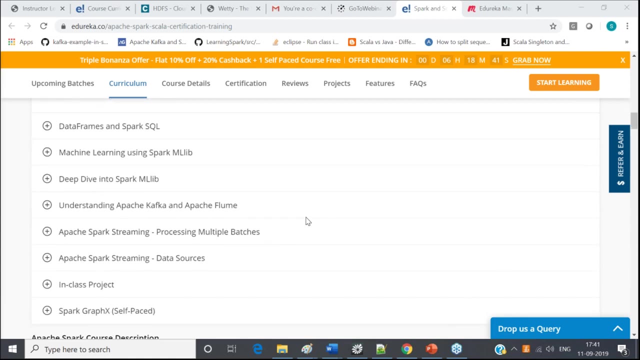 you know aggregation, or how do you load the data, and also as part of this module, only you will understand that how spark deals with the fault tolerance, Okay, or what, if something goes wrong in the memory, then how it will be the computing that and then what we have- we do have data frames. 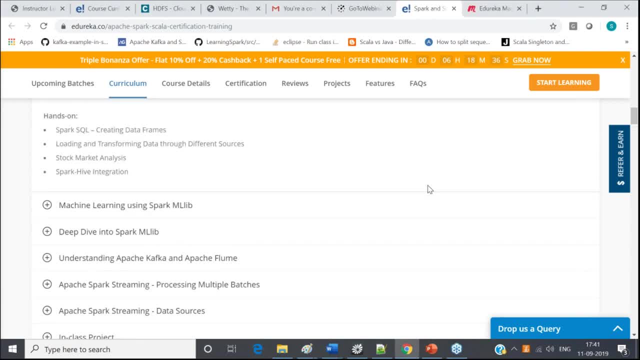 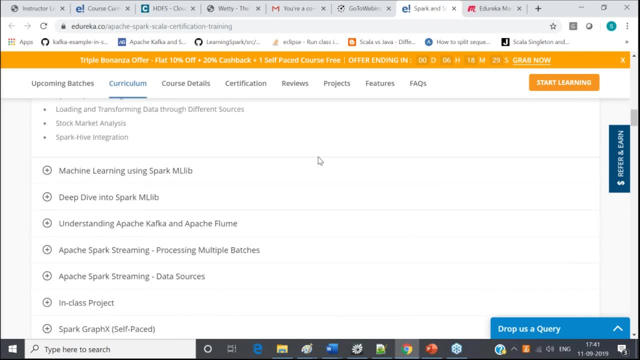 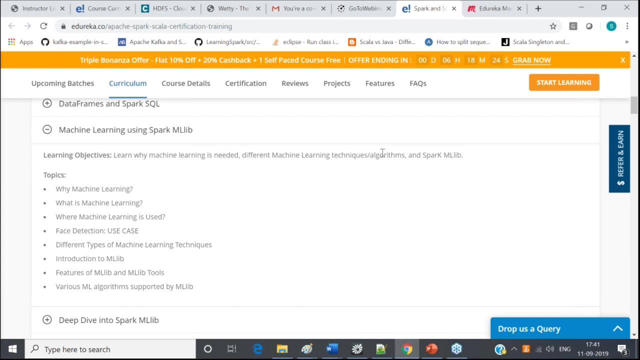 and spark sequel. So as part of this course, you will understand that. how do you Work on the data frames or how will you be writing the sequel like queries? then you will be getting the understanding on the machine learning algorithm. So you will understand what is machine learning, where is being used. 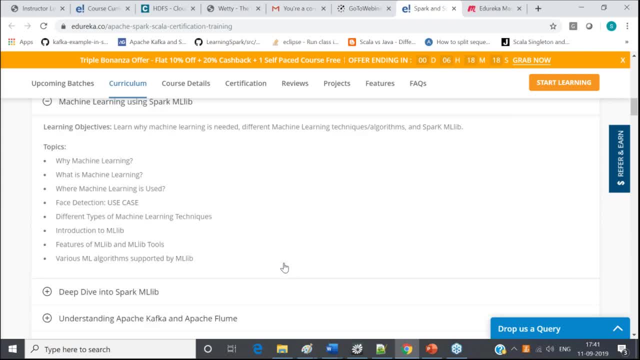 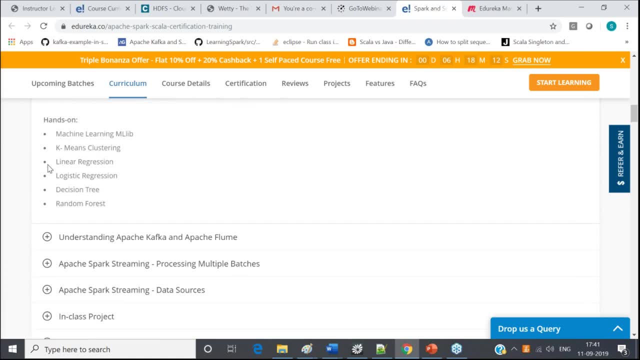 You will be working on couple of use cases and also you will be working like: what are the inbuilt functions which you can use? then deep dive into spark MLA. Then you will be implementing the key means clustering algorithm. You'll be doing the hands-on on logistic regression, linear regression decision tree. 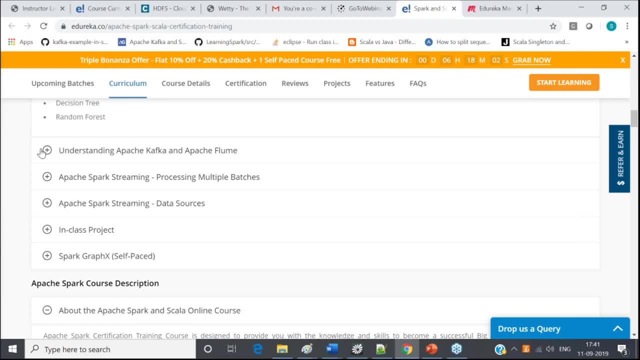 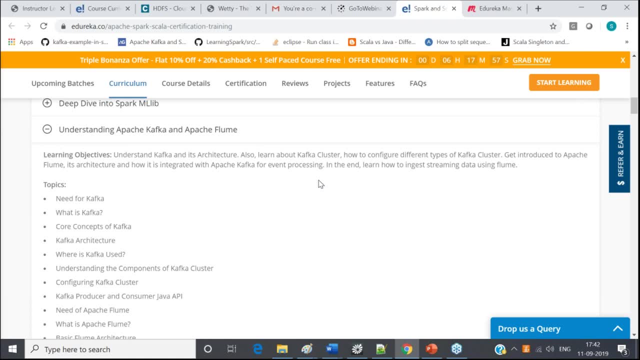 and on the random forest. Then you will be working on Kafka and flume. So you will understand, like, how do you collect the streaming data? What is the Kafka architecture, What is topic, producer, consumer, broker. So you will understand and also you will be getting understanding on flume. 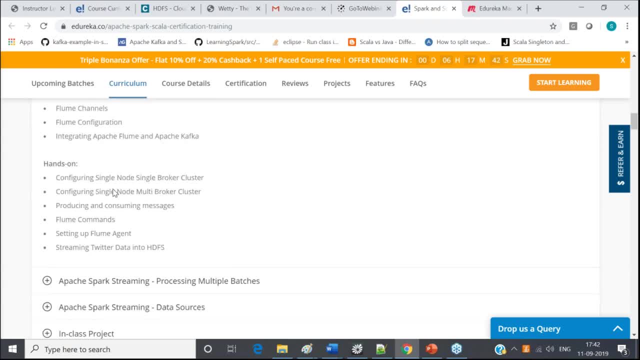 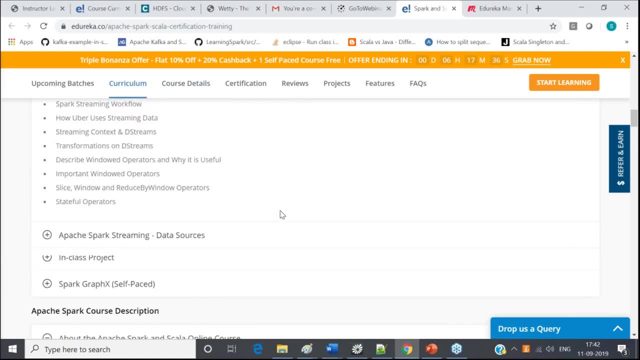 as well as any, will be asked to do the work. You'll be asked to do the hands-on. Okay, then Apache spark streaming. So once you get the understanding that how do you collect the streaming data, then you will go back to sparkcom. 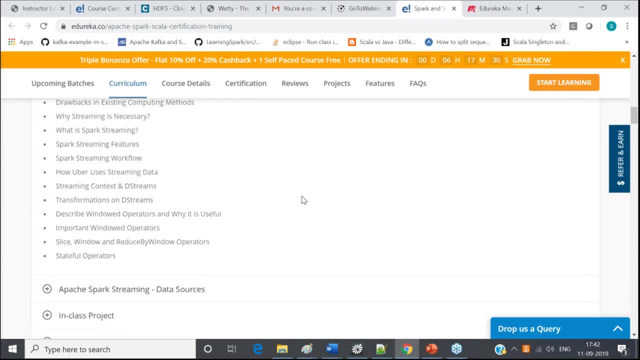 streaming, and then you'll be working on the integration of spark streaming with Kafka and with flume, and then you will be implementing the business logic right. So, yeah, so the head again. you'll be working on couple of use cases. Then there is this in-class project. 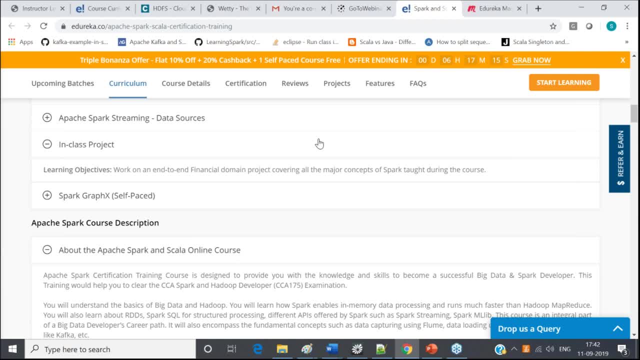 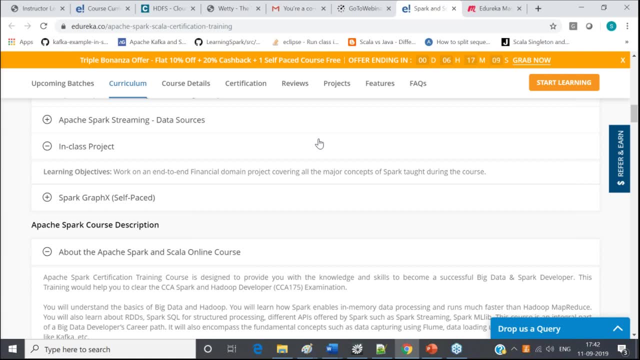 So, yeah, you will be given the data set and you will be. you will be given the data set on the financial domain, as in: you'll be given the data set and you'll be asked to predict the loan repayment ability of a customer, and also you'll be asked to predict. 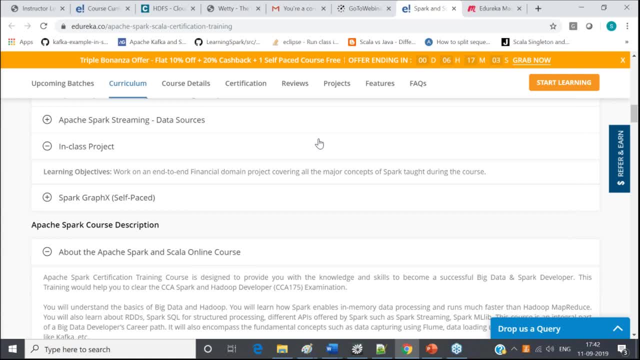 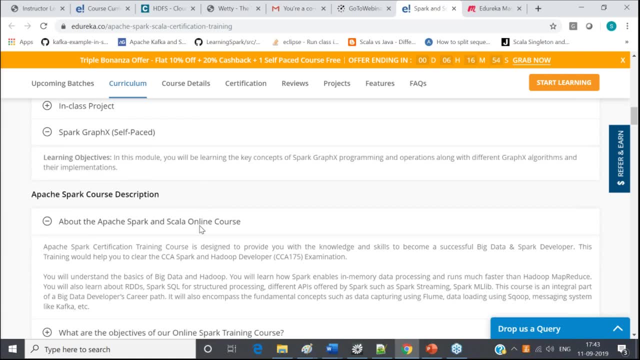 like what is eligibility of the customer and what should be the tenure. and then for graphics, you will be given the study material and the recorded lecture and you'll be able to understand how this park graphics works. Okay, and at the end of the course, 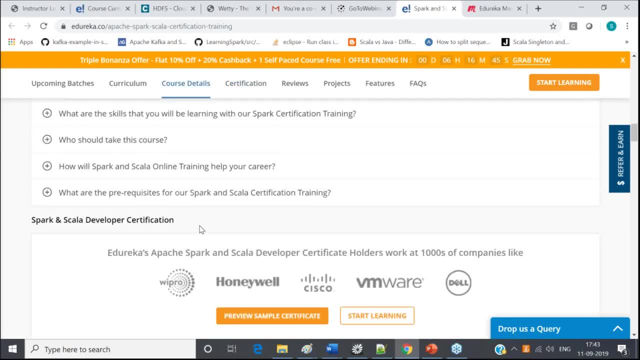 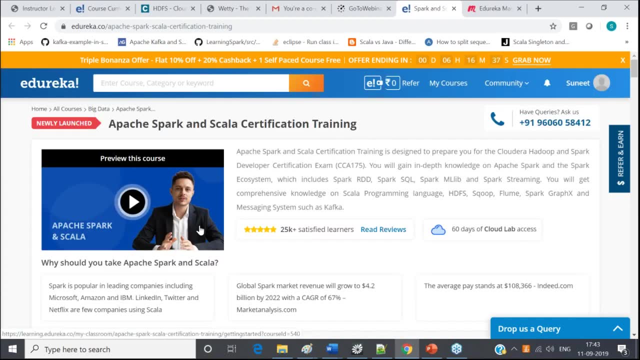 you'll get a certificate from Edureka, and also Edureka has a support team available 24 by 7, which is a technical team, So you can always reach out to them if you have any questions or any issues. Okay, Technology used for achieving the SLA so that we can Google. 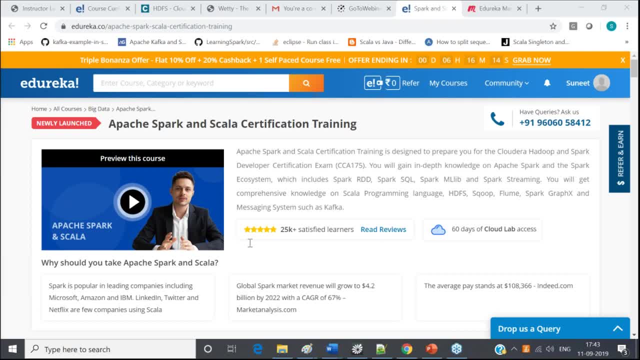 Yeah, again, that will depend on the use case. There are no specific set of components, So every month a new ecosystem component is coming, Ravi. So always you will be starting with the POCs, You will be comparing The performance and then you will decide that for your project. 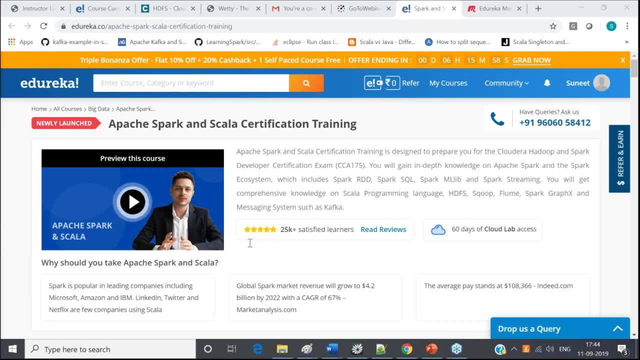 This will be the best accelerator which we can use. Okay, So yeah, any other questions here? anyone before we wrap up the session? Ravi says: can we expect 30-40 likes per year after learning spark, even if you are having experience in some other field? 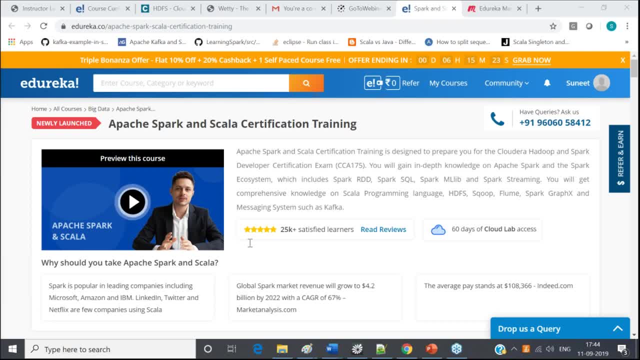 Yes, that depends like how much is your past experience and on what all technologies you have worked in the past. Okay, So, yeah, any other questions here? I don't see any questions coming, So I hope we are good to wrap up the session.